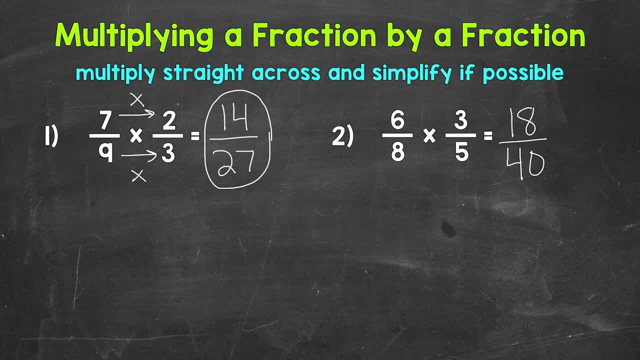 Now eighteen-fortieths can be simplified. The greatest common factor between eighteen and forty is two, So let's divide both of these by two in order to simplify. Eighteen divided by two is nine, and forty divided by two is twenty. 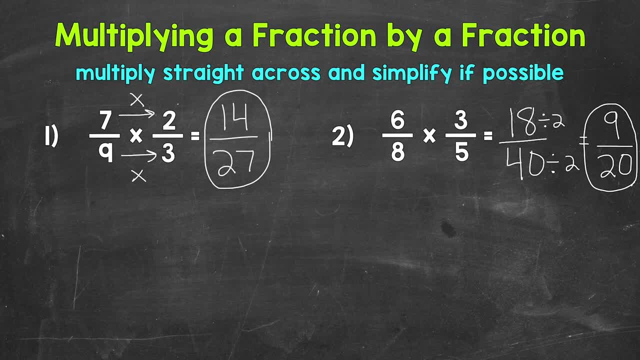 So we get a final simplified answer of nine-twentieths. The only common factor between nine and twenty is one. so we are, in simplest form, The final simplified answer: nine-twentieths. There's how to multiply a fraction by a fraction. 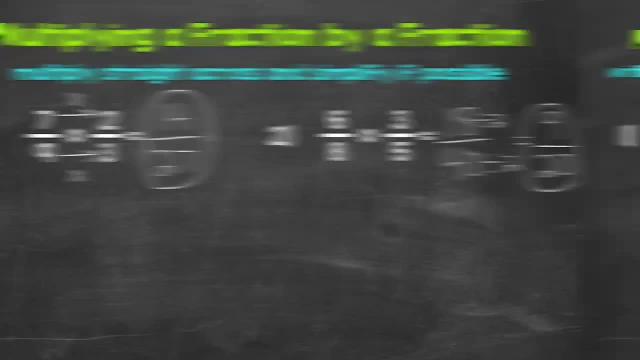 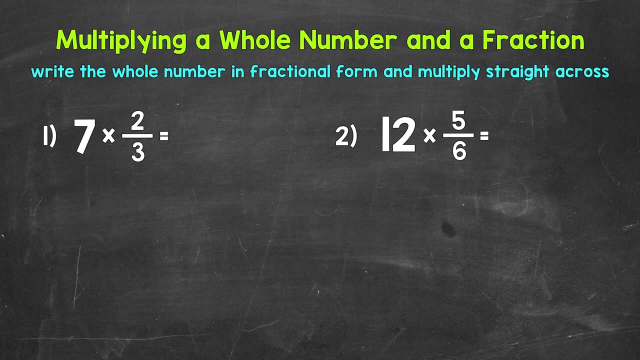 Let's move on to multiplying whole numbers by fractions. Now we will take a look at how to multiply a whole number by a fraction. Let's jump into our examples, starting with number one, where we have seven times two-thirds. Now remember when we multiply fractions. 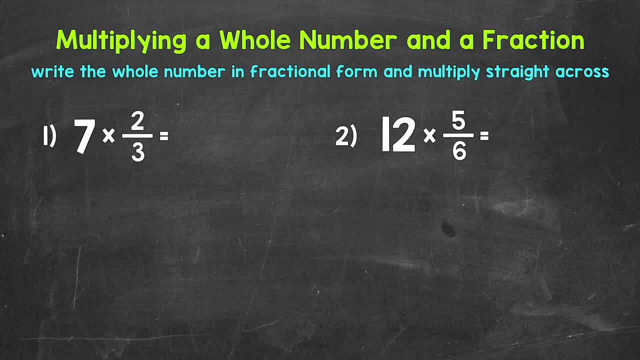 we multiply straight across. So multiply the numerators- the top numbers- and then multiply the denominators- the bottom numbers. Since we have a whole number within this problem, seven, we need to write that whole number in fractional form. That way we have a numerator and a denominator. 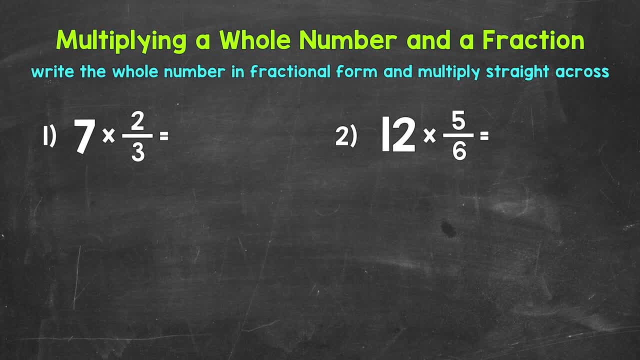 and we can multiply straight across. So let's write seven in fractional form. Now, in order to write a whole number in fractional form, all we need to do is put it over one. We're not changing the value of that whole number, We are just again putting it in fractional form. 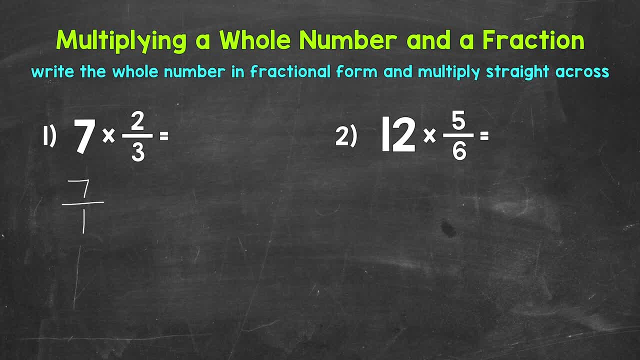 so we're not changing the value of this problem at all. Seven over one still has a value of seven. Then we have times two-thirds. Now we can multiply straight across. Let's start with the numerators. so the top numbers: seven times two. 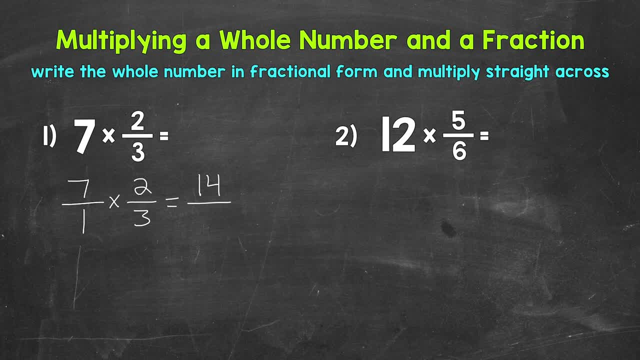 is fourteen. Now for the denominators, the bottom numbers. one times three is three, So we get fourteen over three. fourteen-thirds. Now, that is our answer, but it is an improper fraction, So let's convert it to a mixed number. 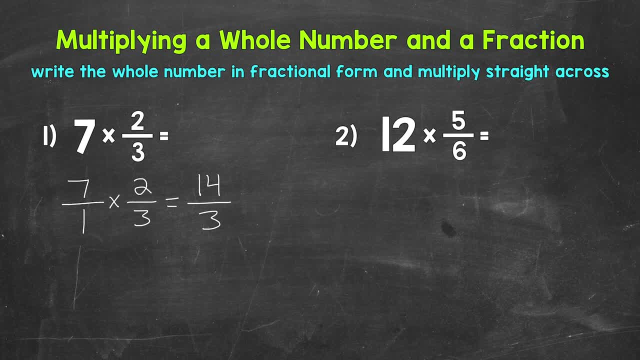 We do that by dividing the numerator by the denominator. So fourteen divided by three, How many whole groups of three in fourteen? Well, four, That's the whole number. part of our mixed number Now we don't hit fourteen. exactly Four whole groups of three gets us to twelve. 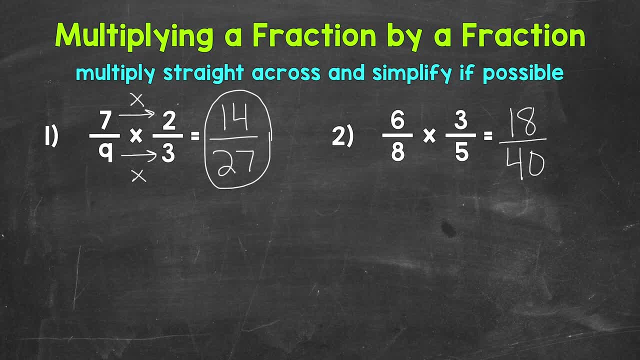 Now eighteen-fortieths can be simplified. The greatest common factor between eighteen and forty is two, So let's divide both of these by two in order to simplify. Eighteen divided by two is nine, and forty divided by two is twenty. 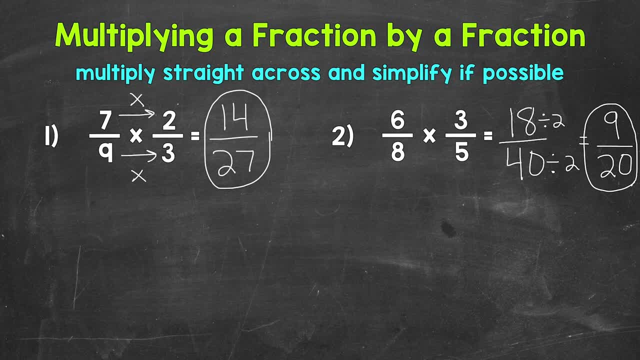 So we get a final simplified answer of nine-twentieths. The only common factor between nine and twenty is one. So we are, in simplest form, The final simplified answer: nine-twentieths. There's how to multiply a fraction by a fraction. 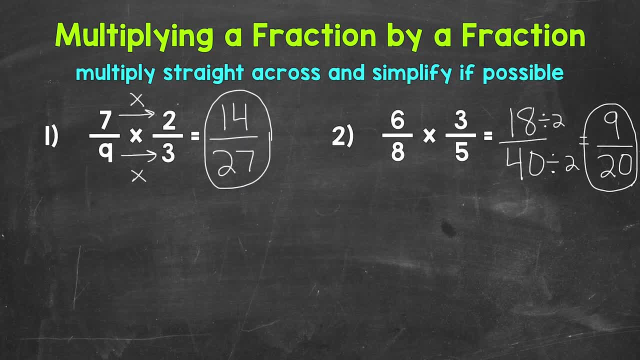 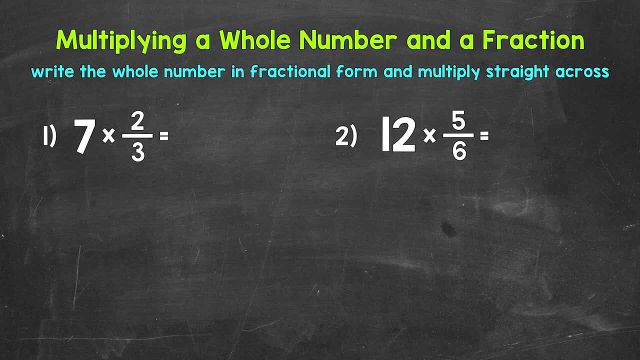 Let's move on to multiplying whole numbers by fractions. Now we will take a look at how to multiply a whole number by a fraction. Let's jump into our examples, starting with number one, where we have seven times two-thirds. Now remember, when we multiply fractions, we multiply straight across. 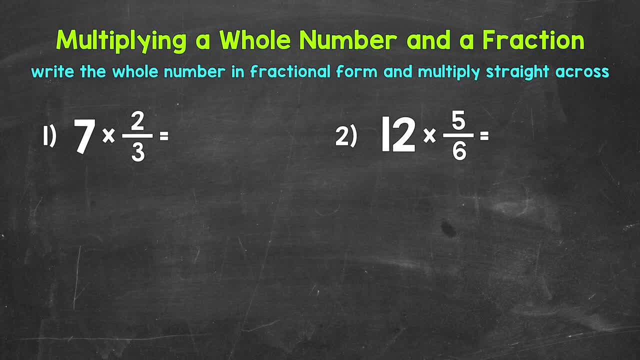 So multiply the numerators- the top numbers- and then multiply the denominators- the bottom numbers. Since we have a whole number within this problem, seven, we need to write that whole number in fractional form. That way we have a numerator and a denominator and we can multiply straight across. 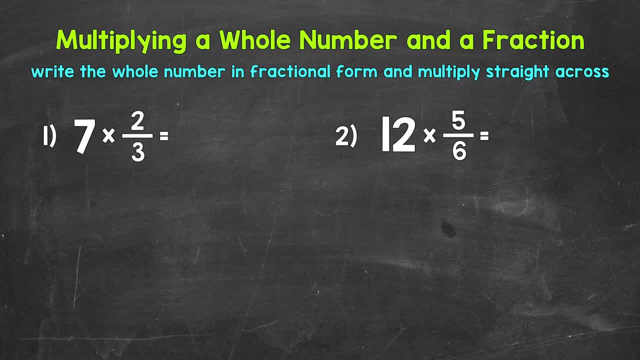 So let's write seven in fractional form. Now, in order to write a whole number in fractional form, all we need to do is put it over one. We're not changing the value of that whole number, We are just again putting it in fractional form. 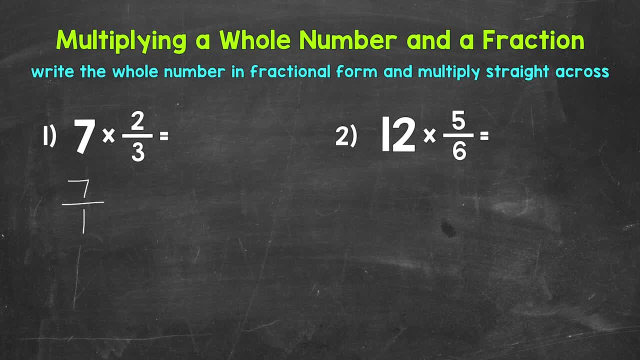 So we're not changing the value of this problem at all. Seven over one still has a value of seven. Then we have times two-thirds. Now we can multiply straight across. Let's start with the numerators. so the top numbers: seven times two. 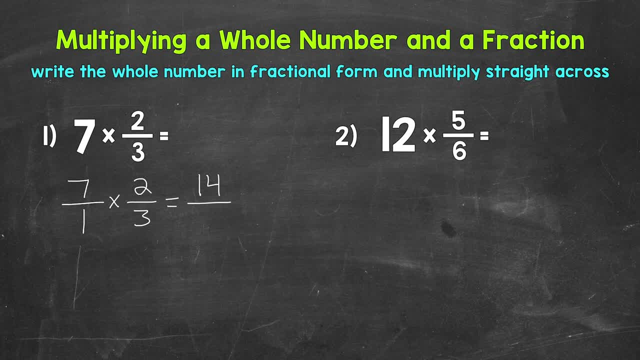 Is fourteen. Now for the denominators, the bottom numbers. one times three is three, So we get fourteen over three. fourteen-thirds. Now, that is our answer, but it is an improper fraction, So let's convert it to a mixed number. 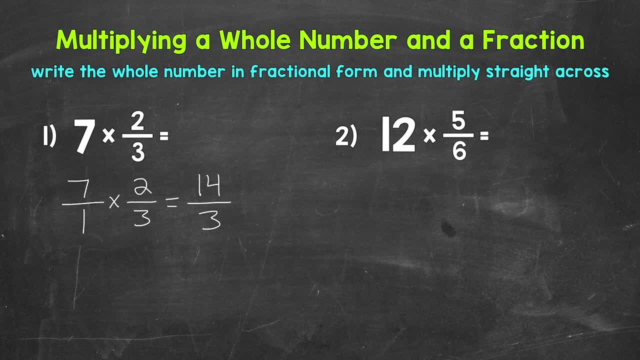 We do that by dividing the numerator by the denominator. So fourteen divided by three, How many whole groups of three in fourteen? Well, four, That's the whole number. part of our mixed number Now we don't hit fourteen. exactly Four whole groups of three gets us to twelve. 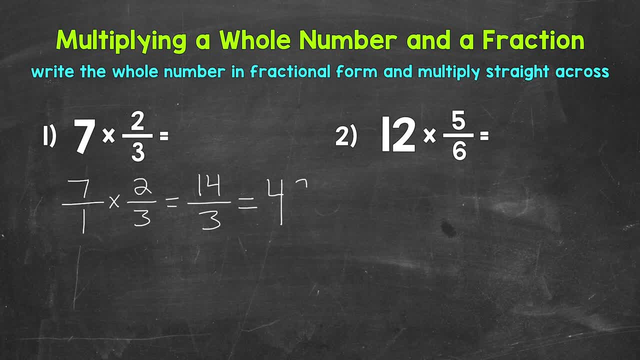 So we have a remainder of two. That remainder is the numerator of the fractional part of the mixed number, And then we keep the denominator of three the same. Always. look to see if you can simplify the fractional part of a mixed number. Two-thirds is in simplest form. 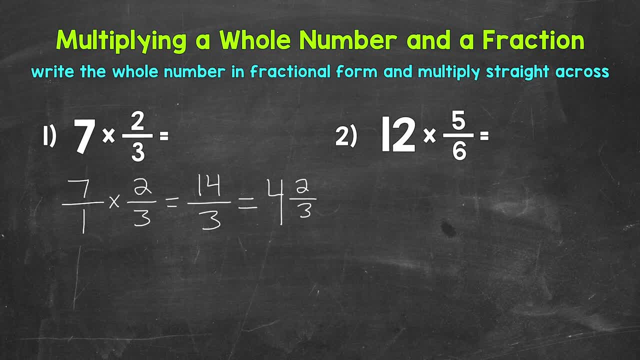 The only common factor between two and three is one. So we are done. Final answer: four and two-thirds. Now, just as a quick recap as far as how we went from fourteen-thirds, fourteen over three, that improper fraction to the mixed number. 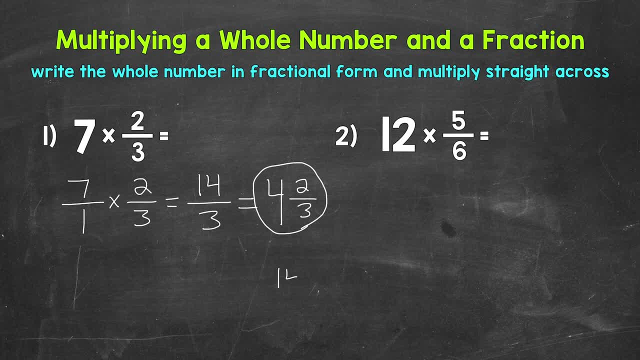 Again, we divided the numerator, so fourteen, and we divided by the denominator three, So fourteen. divided by three, How many whole groups of three? Three in fourteen? Well, four whole groups, That's the whole number portion of our mixed number. 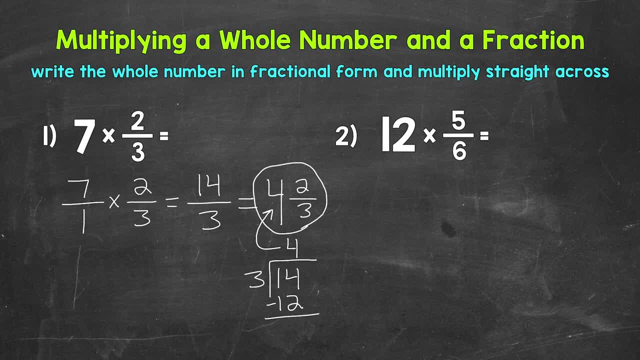 Four times three is twelve. Subtract fourteen minus twelve gives us two, So a remainder of two. That's the numerator of our fractional part of the mixed number. And then we keep the denominator of three the same, So four and two-thirds. 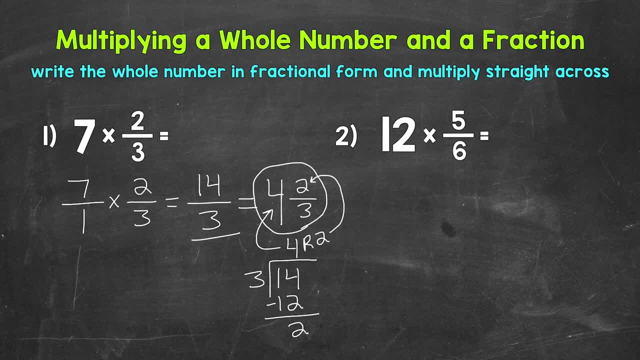 Let's move on to number two, where we have twelve times five-sixths. So let's rewrite twelve in fractional form by putting it over one times five-sixths. Now we can multiply straight across. Let's start with the numerators: Twelve times five is sixty. 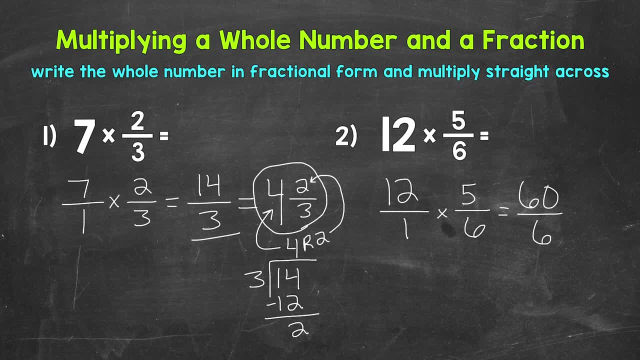 Now for the denominators. One times six is six. We get sixty-sixths or sixty over six, And that's our answer. but it's an improper fraction, So let's convert it to a mixed number. Let's divide the numerator sixty by the denominator six. 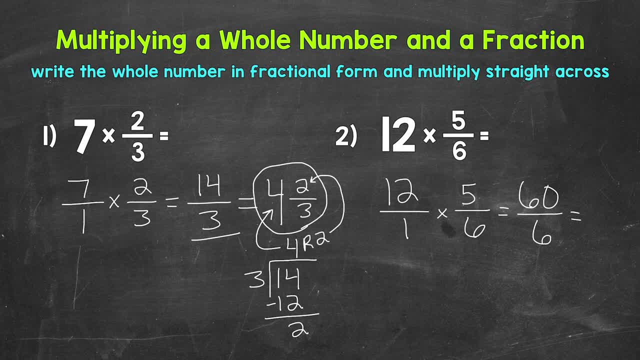 So sixty divided by six, How many whole groups of six in sixty? Well, ten, That hits sixty exactly. We don't have a remainder. So this is our final answer: We get a whole number answer And we don't have a remainder there. 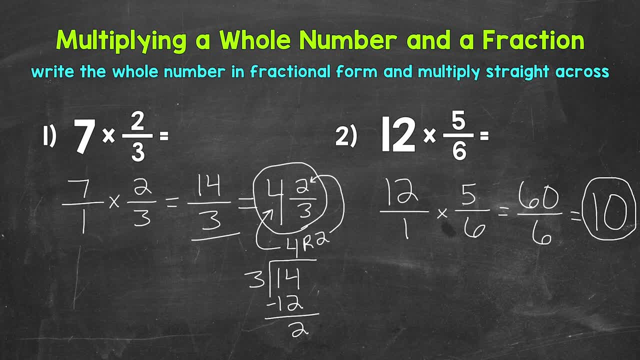 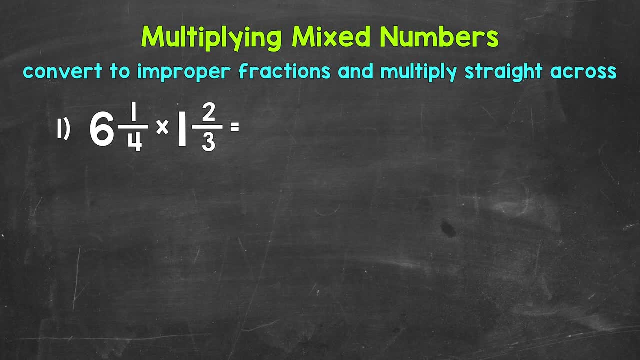 So our answer is just ten. There's how to multiply a whole number by a fraction. Let's move on to multiplying mixed numbers. Now we will take a look at how to multiply a mixed number by a mixed number. We will go through two examples. 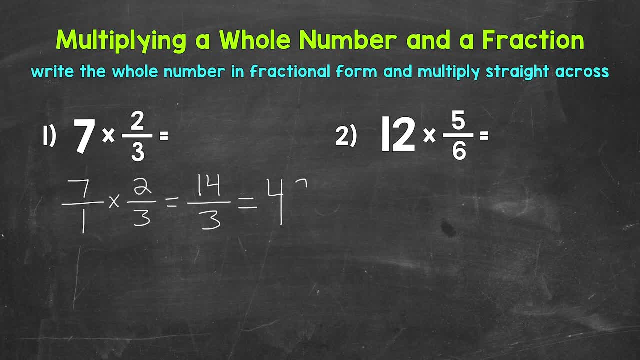 So we have a remainder of two. That remainder is the numerator of the fractional part of the mixed number, And then we keep the denominator of three the same. Always. look to see if you can simplify the fractional part of a mixed number. Two-thirds is in simplest form. 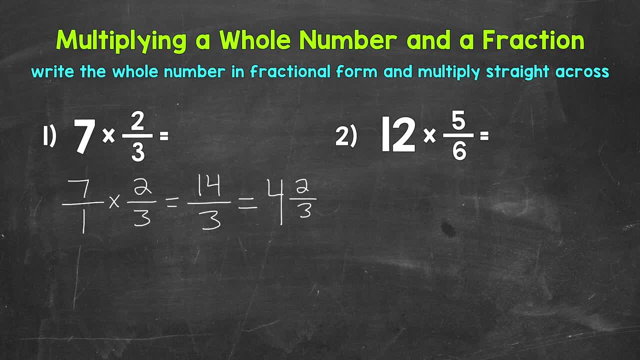 The only common factor between two and three is one. So we are done. Final answer: four and two-thirds. Now, just as a quick recap as far as how we went from fourteen-thirds, fourteen over three, that improper fraction to the mixed number. 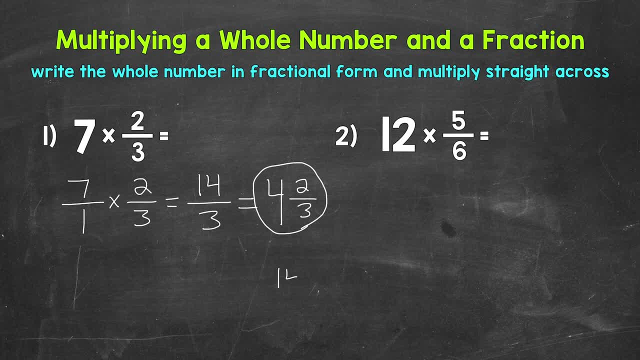 Again, we divided the numerator, so fourteen, and we divided by the denominator three, So fourteen. divided by three, How many whole groups of three? Three in fourteen? Well, four whole groups, That's the whole number portion of our mixed number. 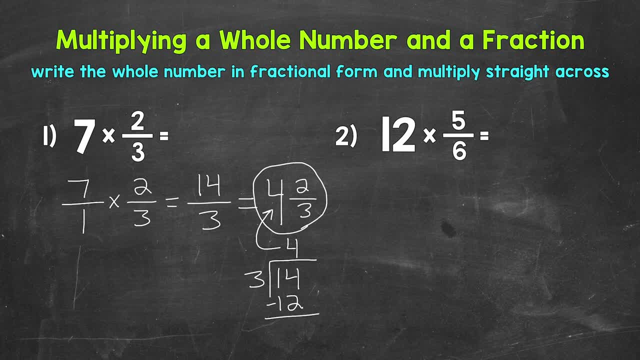 Four times three is twelve. Subtract Fourteen minus twelve gives us two, So a remainder of two. That's the numerator of our fractional part of the mixed number. And then we keep the denominator of three the same, So four and two-thirds. 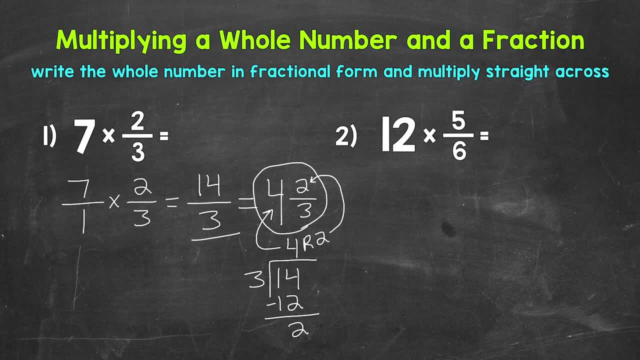 Let's move on to number two, where we have twelve times five-sixths. So let's rewrite twelve in fractional form by putting it over one Times five-sixths. Now we can multiply straight across. Let's start with the numerators: Twelve times five is sixty. 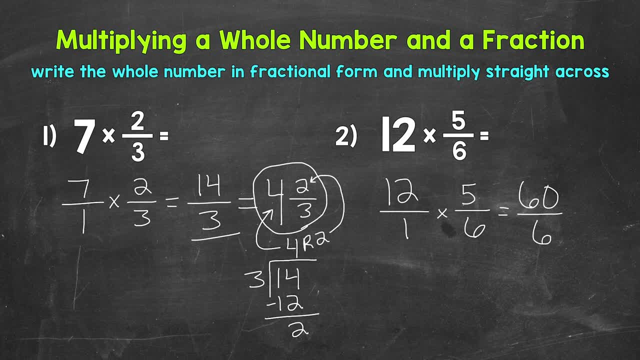 Now for the denominators. One times six is six, So we get sixty-sixths or sixty over six, And that's our answer. but it's an improper fraction, So let's convert it to a mixed number. Let's divide the numerator sixty by the denominator six. 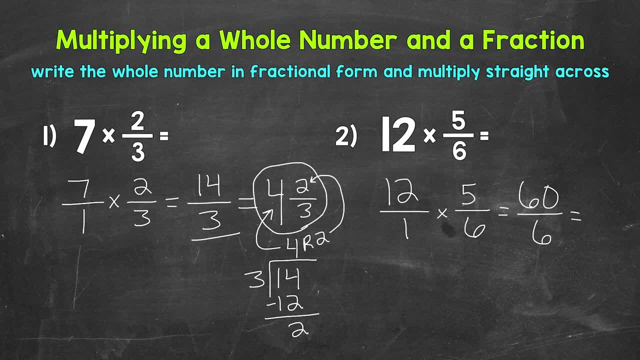 So sixty divided by six, How many whole groups of six in sixty? Well, ten, That hits sixty exactly. We don't have a remainder. So this is our final answer: We get a whole number. answer Again: we don't have a remainder there. 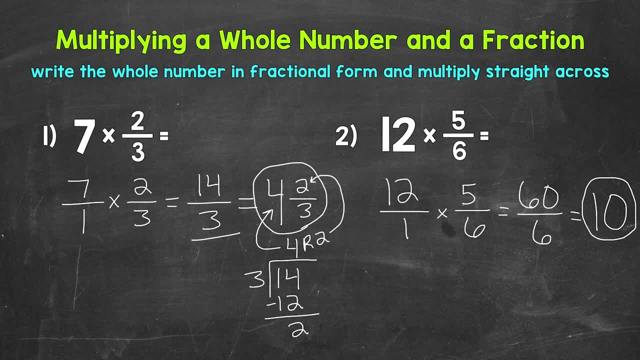 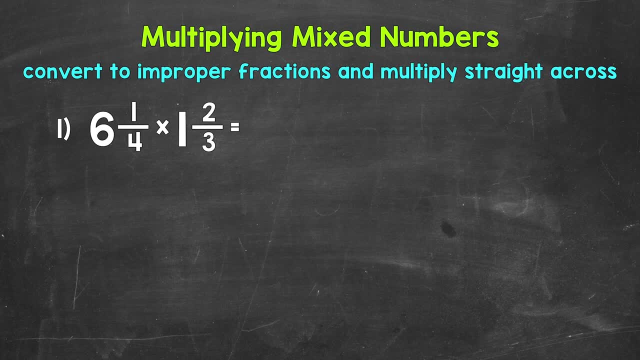 So our answer is just ten. There's how to multiply a whole number by a fraction. Let's move on to multiplying mixed numbers. Now we will take a look at how to multiply a mixed number by a mixed number. We will go through two examples. 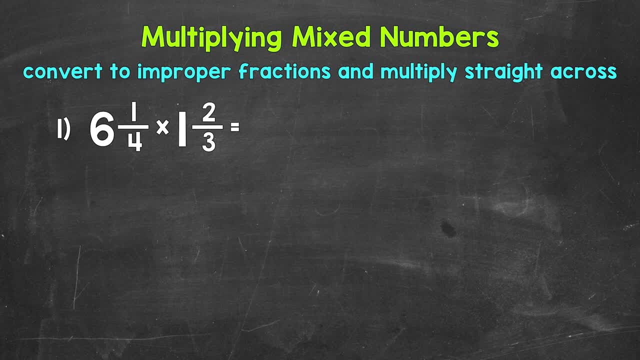 Let's jump into number one, where we have six and one-fourth times one and two-thirds. Now remember, when we have a multiplication problem that involves fractions, we can multiply straight across. So we multiply the numerators, the top numbers, and then we multiply the denominators, the bottom numbers. 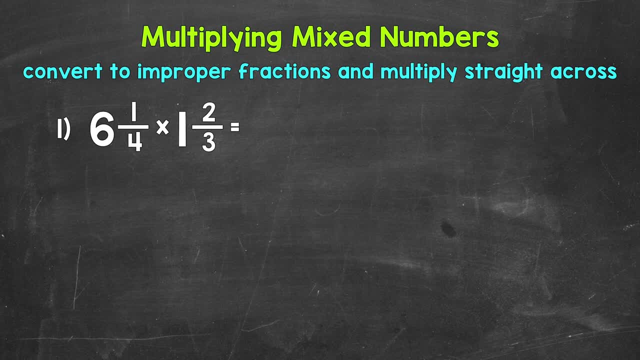 So our first step here is to convert the mixed numbers to improper fractions. That way we just have numerators and denominators and we can multiply straight across. So let's start by converting six And one-fourth to an improper fraction. We do that by starting at the bottom and working our way to the top. 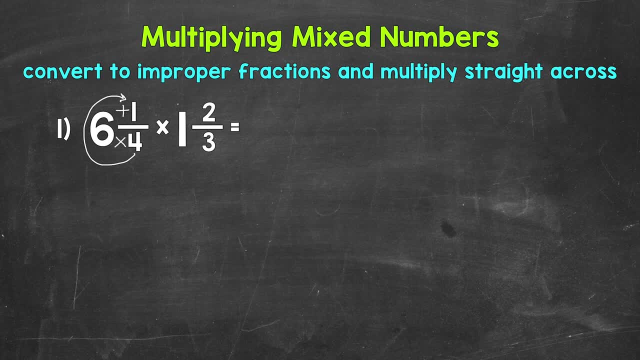 We multiply and then add. So we multiply the denominator by the whole number and then add the numerator. So four times six is twenty-four plus one is twenty-five. That's the numerator of the improper fraction. Then we keep the denominator the same. 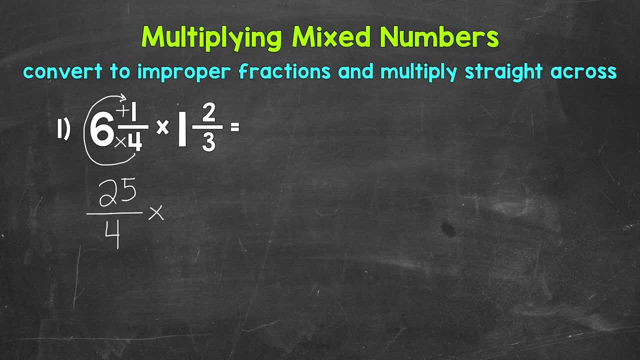 So that is four times, and then we can convert one and two-thirds to an improper fraction. So multiply and then add Three times. one is three plus two is five. Keep the denominator of three the same. Now we just have numerators and denominators. 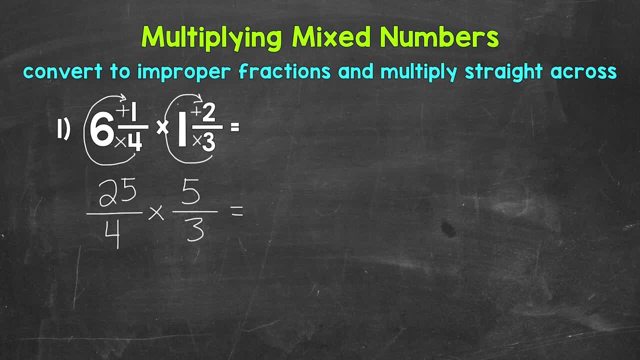 And we can multiply straight across. Let's start with the numerators. So twenty-five times five, that gives us one hundred twenty-five. Now for the denominators: four times three, that gives us twelve. So we end up with one hundred twenty-five over twelve, or one hundred twenty-five twelfths. 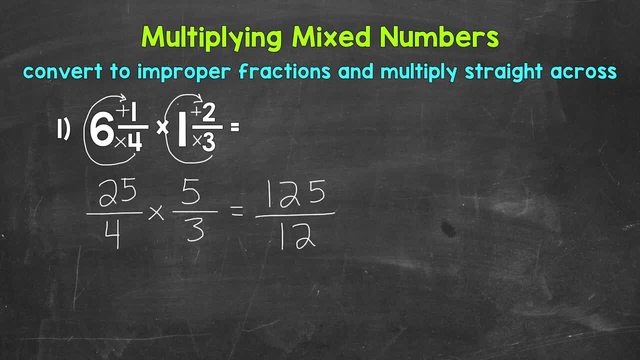 which is our answer. but it's an improper fraction, So let's convert it to a mixed number. We do that by dividing the numerator one hundred twenty-five by the denominator twelve. So one hundred twenty-five divided by twelve, How many whole groups of twelve in one hundred twenty-five? 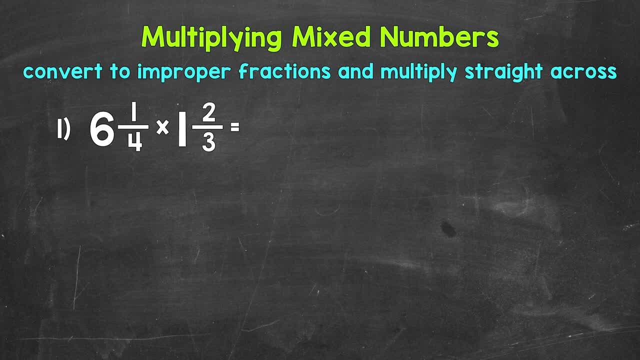 Let's jump into number one, where we have six and one-fourth times one and two-thirds. Now remember, when we have a multiplication problem that involves fractions, we can multiply straight across. So we multiply the numerators, the top numbers, and then we multiply the denominators, the bottom numbers. 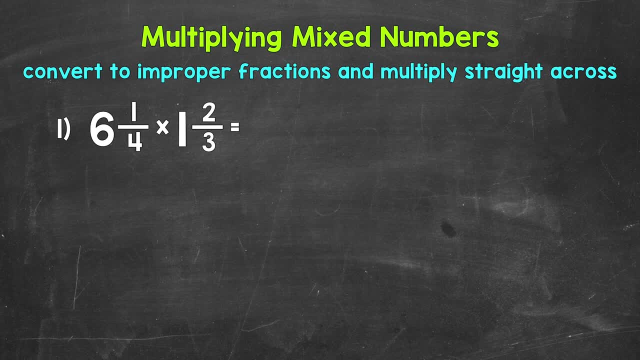 So our first step here is to convert the mixed numbers to improper fractions. That way we just have numerators and denominators and we can multiply straight across. So let's start by converting six and one-fourth to an improper fraction. We do that by starting at the bottom and working our way to the top. 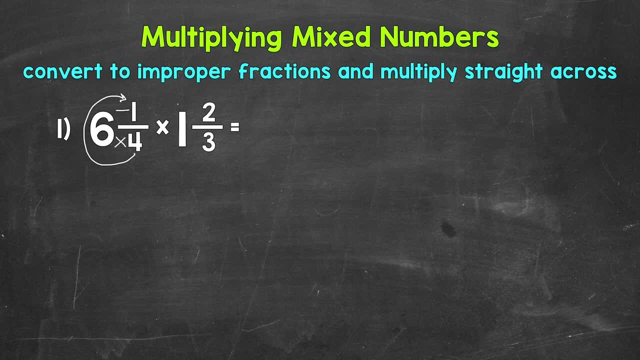 We multiply and then add. So we multiply the denominator by the whole number and then add the numerator. So four times six is twenty-four plus one is twenty-five. That's the numerator of the improper fraction. Then we keep the denominator the same. 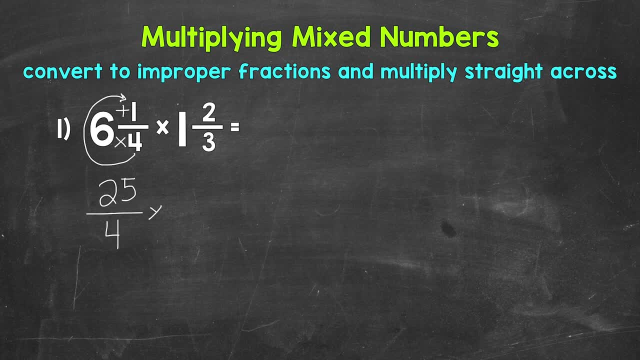 So that is four times, and then we can convert one and two-thirds to an improper fraction. So multiply and then add Three times. one is three plus two is five. Keep the denominator of three the same. Now we just have numerators and denominators and we can multiply straight across. 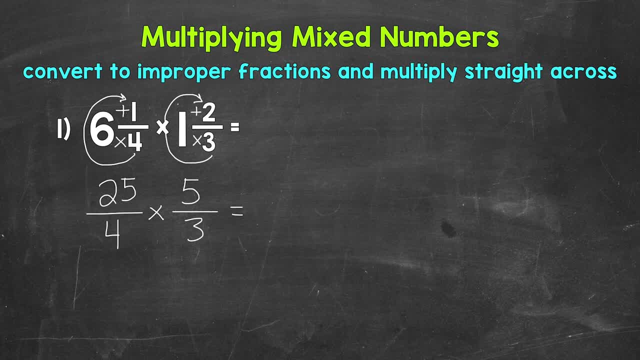 Let's start with the numerators. So twenty-five times five, That gives us one hundred twenty-five. Now for the denominators: Four times three, That gives us twelve. So we end up with one hundred twenty-five over twelve, or one hundred twenty-five twelfths. 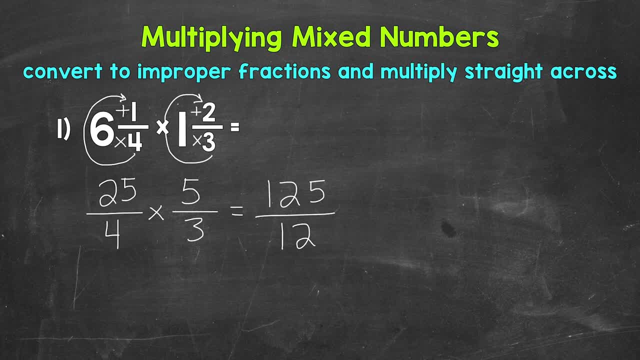 which is our answer. but it's an improper fraction, So let's convert it to a mixed number. We do that by dividing the numerator one hundred twenty-five by the denominator twelve. So one hundred twenty-five divided by twelve, How many whole groups of twelve in one hundred twenty-five? 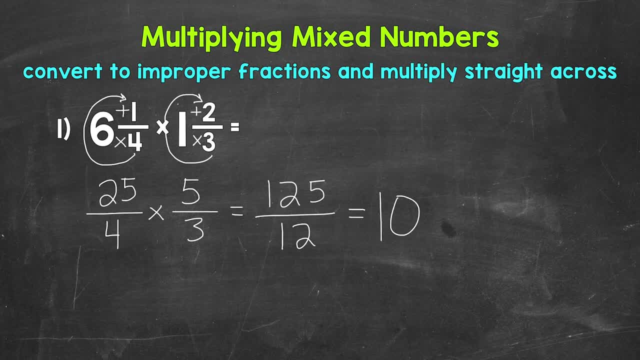 Well, ten, And that's the whole number of our mixed number. That gets us to one hundred twenty. So we have a remainder of five. We don't hit one hundred twenty-five. exactly That remainder of five is the numerator of the fractional part of the mixed number. 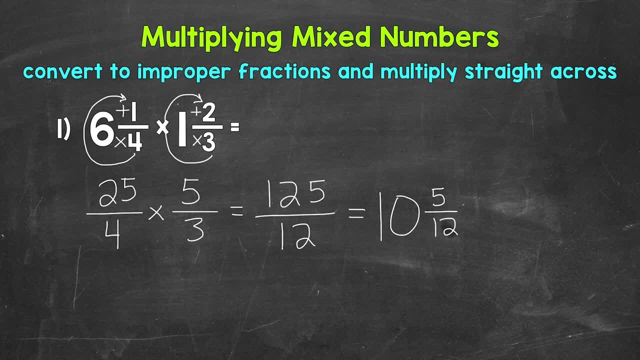 And then we keep the denominator of twelve the same And we get ten and five twelfths. We can look to see if we can simplify the fractional part of this mixed number. Five twelfths is, in simplest form. the only common factor between five and twelve is one. 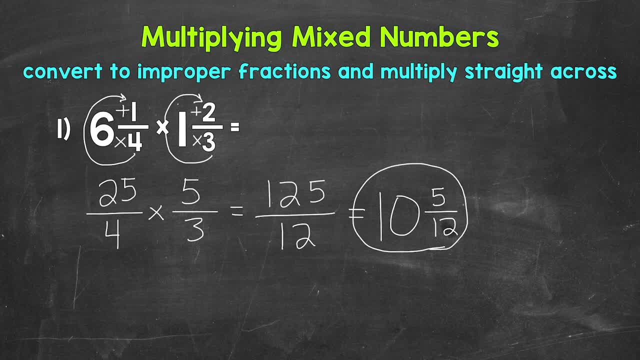 So we are done: Ten and five twelfths. Now, just for a quick recap, let's write out how we went from that improper fraction of one hundred twenty-five twelfths to the mixed number of ten and five twelfths. Again, we divide the numerator, so one hundred twenty-five. 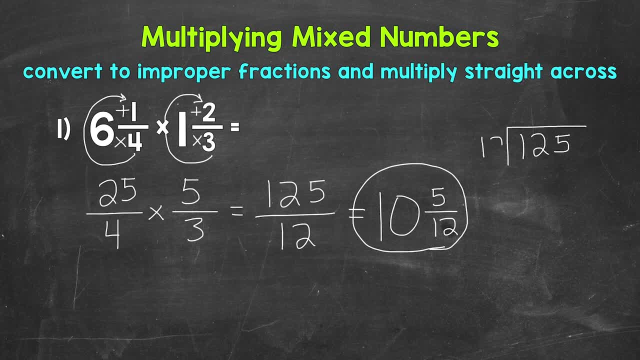 by the denominator twelve, So one hundred twenty-five divided by twelve. We can start with twelve divided by twelve, which is one Multiply one times twelve is twelve. Subtract Five minus twelve is zero, And then bring down. Now we repeat, so go back to divide. 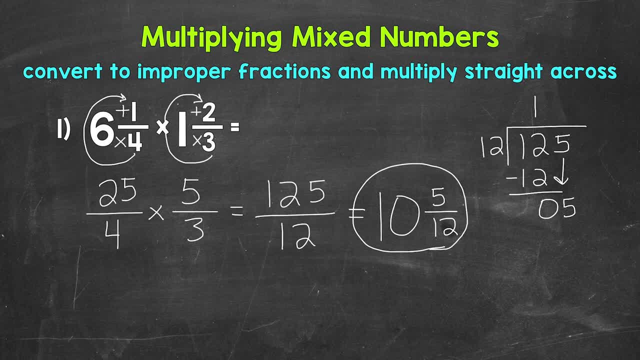 So we have five divided by twelve, which we can't do that, so we need a zero here. Zero times twelve is zero. Subtract Five minus zero is five, So ten remainder five. Ten is the whole number of our mixed number. 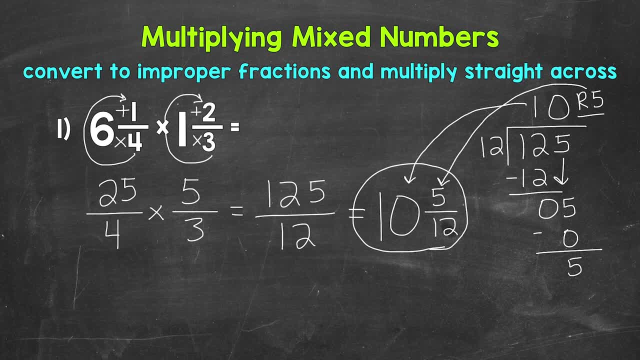 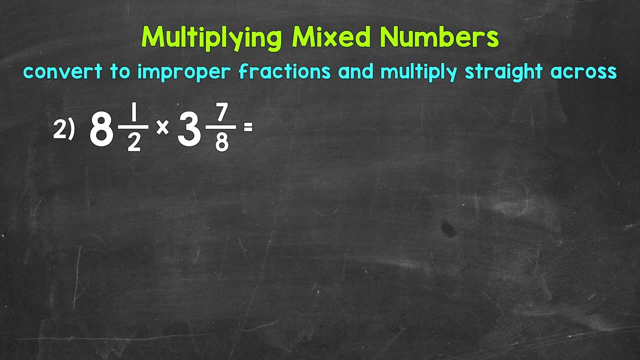 The remainder of five is the numerator, And then we keep the denominator of twelve the same. So again, our final answer: ten and five, twelfths. Let's move on to number two. For number two, we have eight and one half times three and seven, eighths. 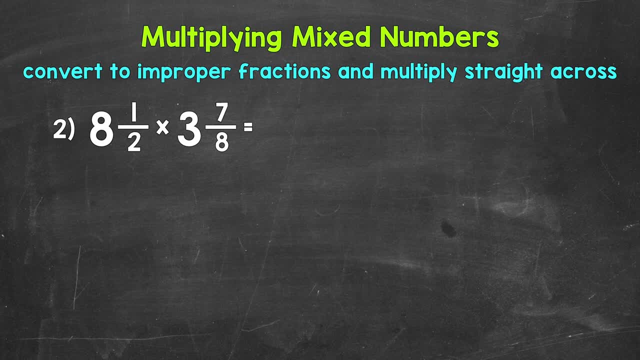 Let's start by converting these mixed numbers to improper fractions. We will do eight and one half first, So two times eight is sixteen Plus one is seventeen over two. So seventeen halves times now four, three and seven eighths. So multiply and then add. 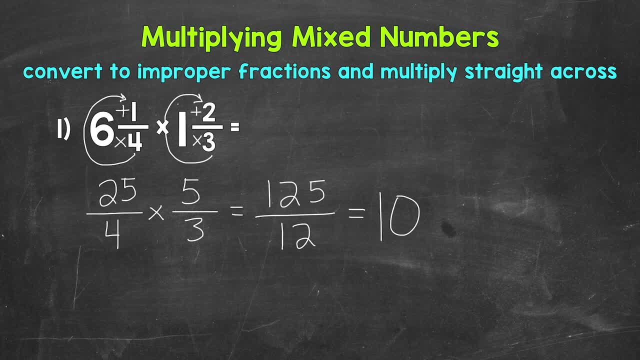 Well, ten, And that's the whole number of our mixed number. That gets us to one hundred twenty. So we have a remainder of five. We don't hit one hundred twenty-five. exactly That remainder of five is the numerator of the fractional part of the mixed number. 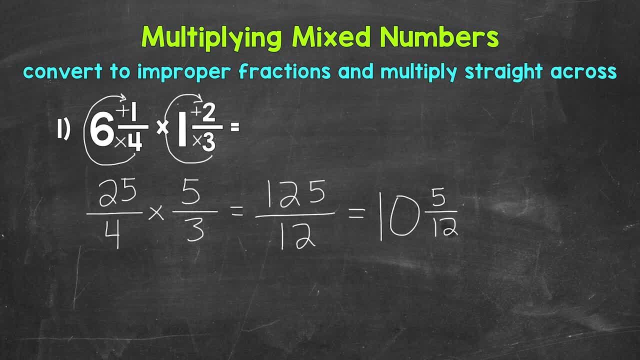 And then we keep the denominator of twelve the same And we get ten and five twelfths. We can look to see if we can simplify the fractional part of this mixed number. Five twelfths is, in simplest form. the only common factor between five and twelve is one. 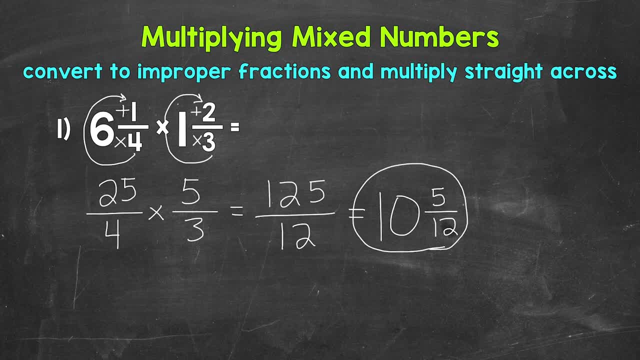 So we are done: Ten and five twelfths. Now, just for a quick recap, I'm going to write out how we went from that improper fraction of one hundred twenty-five twelfths to the mixed number of ten and five twelfths. 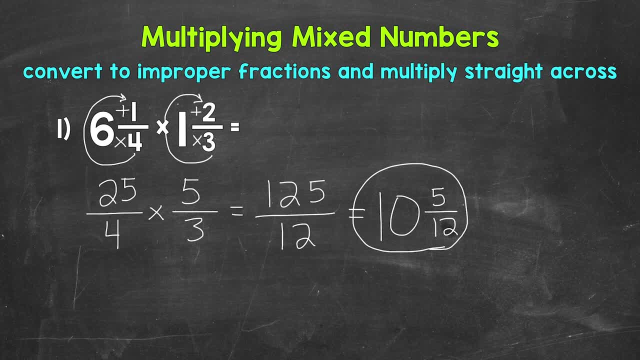 Again, we divide the numerator, so one hundred twenty-five, by the denominator twelve, So one hundred twenty-five divided by twelve. We can start with twelve divided by twelve, which is one. multiply one times twelve is twelve. subtract twelve minus twelve is zero. 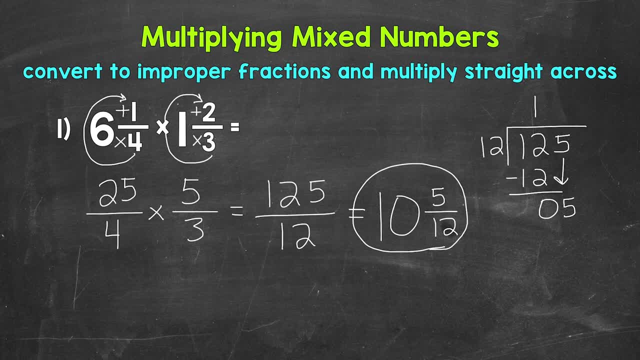 and then bring down. Now we repeat: so go back to divide. So we have five divided by twelve, which we can't do that, so we need a zero here. Zero times twelve is zero. Subtract five minus zero is five. 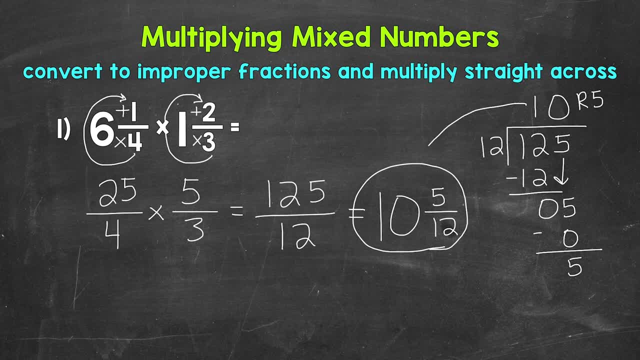 So ten remainder five. Ten is the whole number of our mixed number. The remainder of five is the numerator, and then we keep the denominator of twelve the same. So again, our final answer: ten and five twelfths. Let's move on to number two. 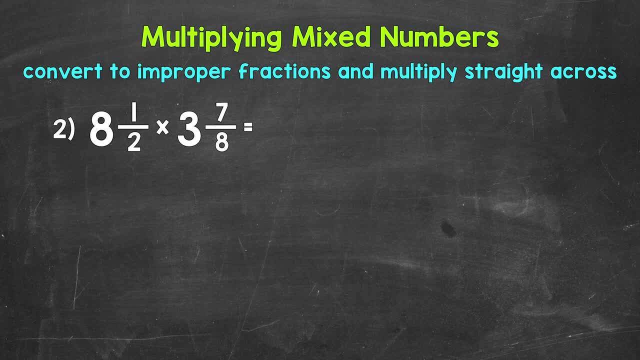 For number two we have eight and one half times three and seven eighths. Let's start by converting these mixed numbers to improper fractions. We will do eight and one half one half first. so two times eight is sixteen plus one is seventeen over two. 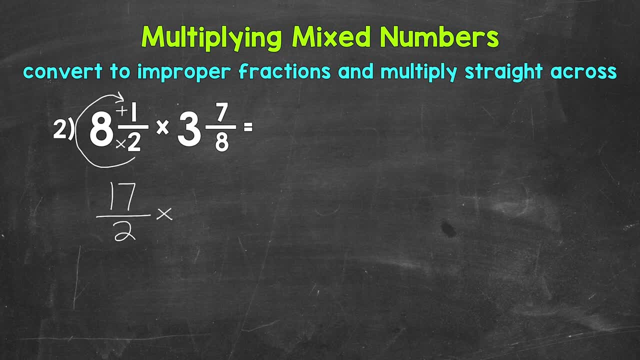 so seventeen halves times now, four, three and seven, eighths. So multiply and then add Eight times three is twenty-four plus seven is thirty-one, And then we keep the denominator of eight the same. Now we can multiply straight across. 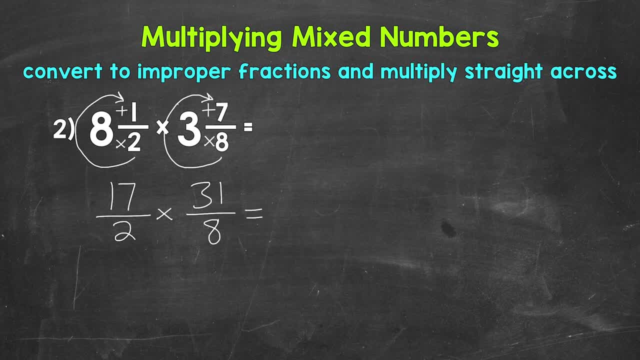 and we will start with the numerators. So seventeen times thirty-one For number two. this is going to take a little more work than number one. I'm not sure what seventeen times thirty-one is, so I'm going to go to the side and write this out and multiply. 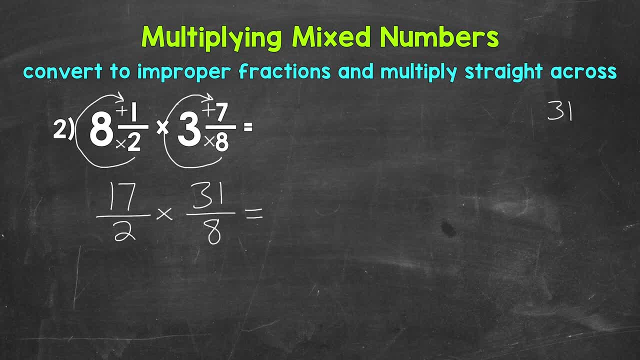 So let's do thirty-one. I'll put the larger number in value on top times seventeen. Seven times one is seven. Seven times three. Seven times three is twenty-one. Now we need a zero, And then we have one times one is one. 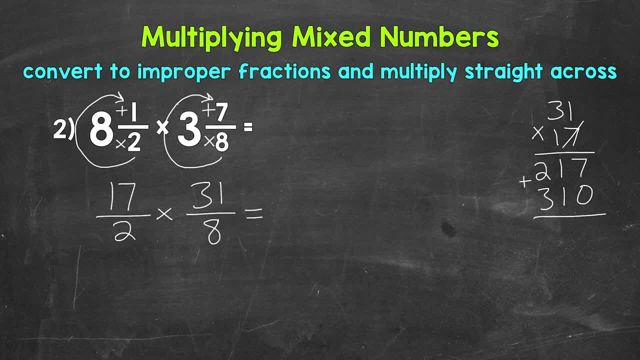 And then one times three is three. Add Seven plus zero is seven. One plus one is two, And then two plus three is five. So we get five hundred twenty-seven for the numerator, And then, as far as the denominators, we have two times eight. 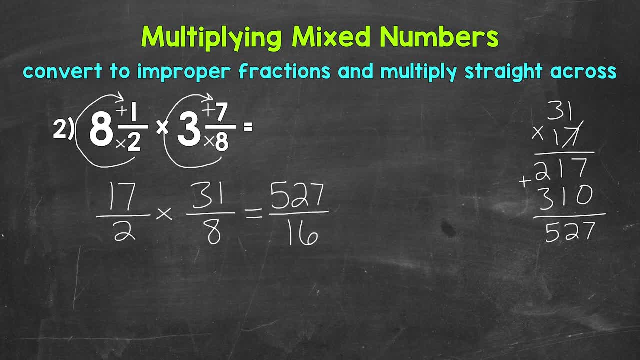 Which is sixteen. So we end up with five hundred twenty-seven over sixteen or five hundred twenty-seven sixteenths. That is our answer, but it's an improper fraction, So let's convert it to a mixed number by dividing the numerator five hundred twenty-seven. 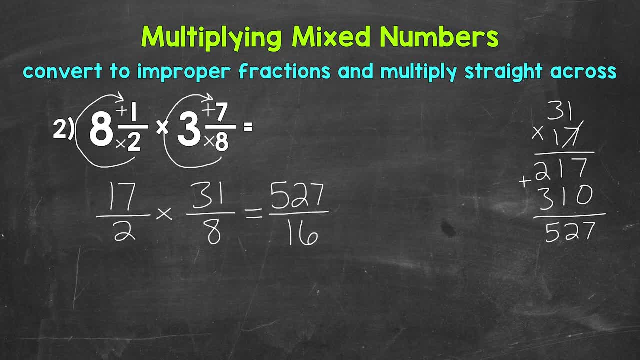 by the denominator sixteen. Now I'm not sure what that answer is, So again, I'm going to come off to the side and work through that. So five hundred twenty-seven divided by sixteen, So we will start with fifty-two divided by sixteen. 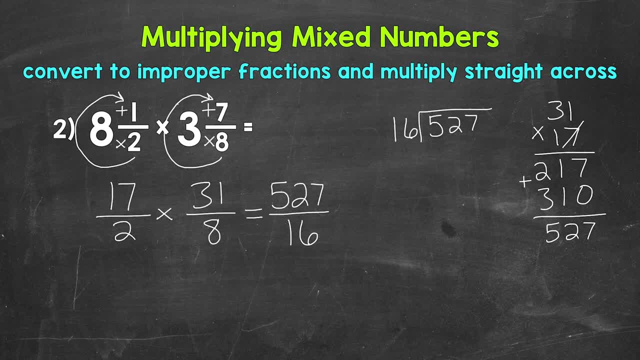 How many whole groups of sixteen in fifty-two? Well, three, That gets us to forty-eight. Multiply Three times sixteen is forty-eight. Fifty-two minus forty-eight is four. Bring down the seven, And now we repeat, So we divide. We have forty-seven divided by sixteen. 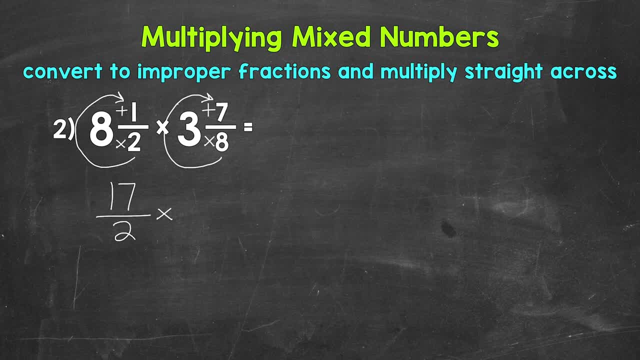 Eight times three is twenty. four plus seven is thirty one, And then we keep the denominator of eight the same. Now we can multiply straight across and we will start with the numerators. So seventeen times thirty one For number two, this is going to take a little more work than number one. 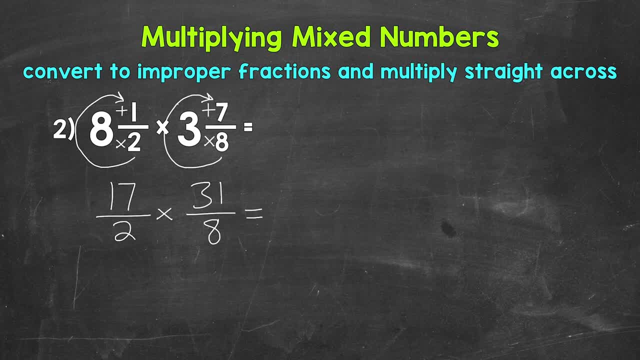 I'm not sure what seventeen times thirty one is, So I'm going to go to the side and write this out and multiply. So let's do thirty one. I'll put the larger number in value on top times seventeen. Seven times one is seven. 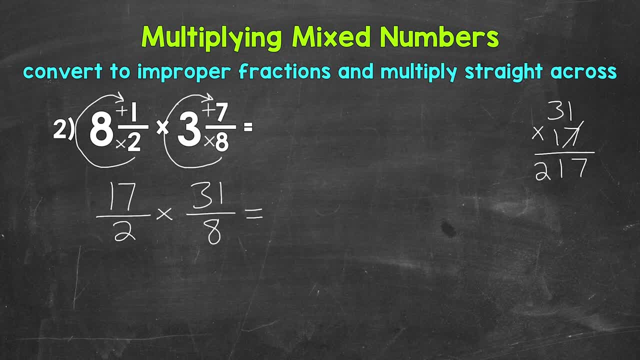 Seven times three is twenty one. Now we need a zero And then we have: one times one is one, And then one times three is three. Add seven plus zero is seven. One plus one is two, And then two plus three is five. 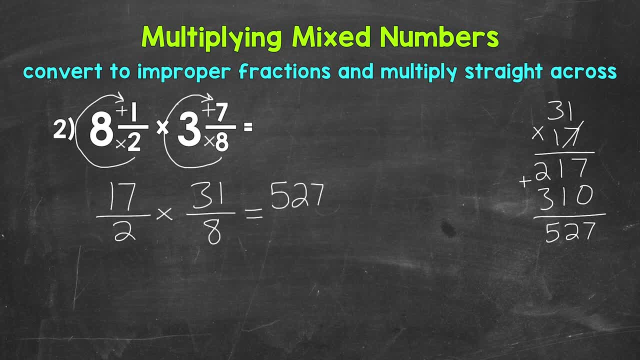 So we get five hundred twenty seven for the numerator, And then, as far as the denominators, we have two times eight, which is sixteen. So we end up with five hundred twenty seven Over sixteen, or five hundred twenty seven sixteenths. 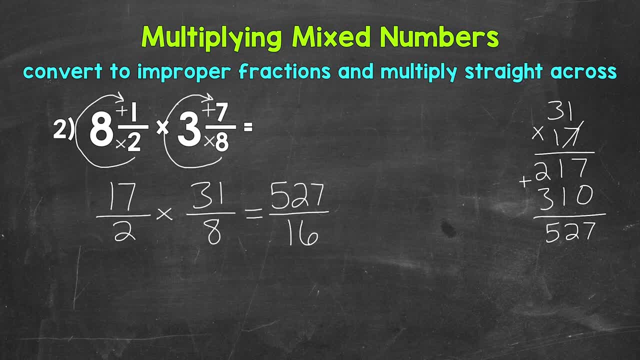 That is our answer, but it's an improper fraction, So let's convert it to a mixed number by dividing the numerator Five hundred twenty seven by the denominator Sixteen. Now I'm not sure what that answer is, So again, I'm going to come off to the side and work through that. 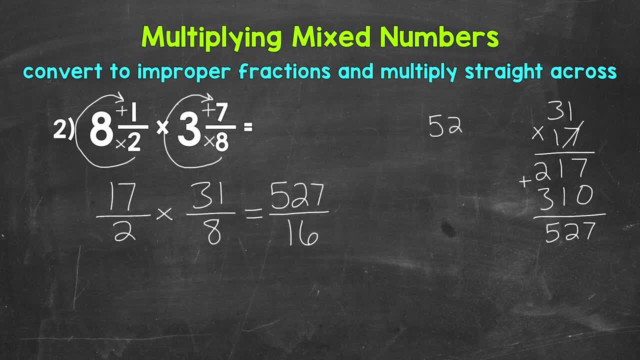 So five hundred twenty seven Divided by Sixteen, So we will start With fifty two divided by sixteen, How many whole groups of sixteen in fifty two? Well, three, that gets us to forty eight. Multiply three times sixteen Is forty eight. 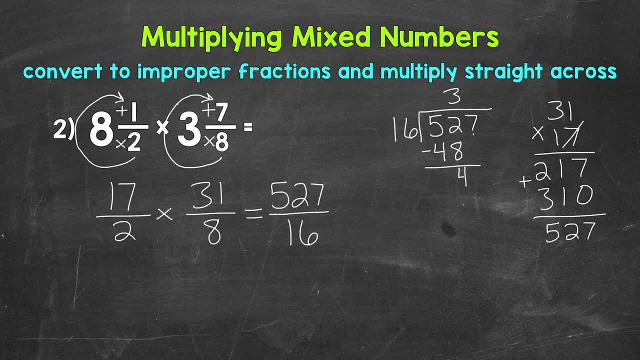 Fifty two minus forty eight is four. Bring down the seven, And now we repeat, So we divide. We have forty seven divided by sixteen, How many whole groups of sixteen in forty seven? Well, two That gets us to thirty two. 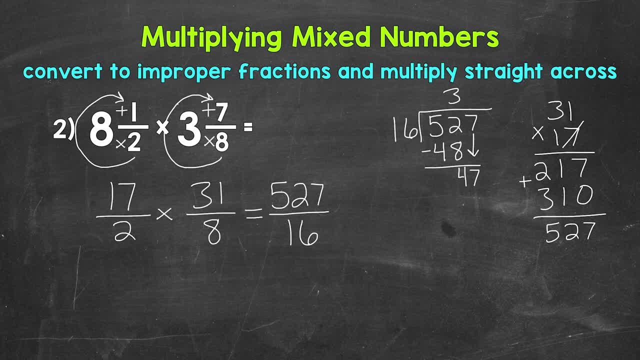 How many whole groups of sixteen in forty-seven? Well, two That gets us to thirty-two. And now we can multiply Two times. sixteen is thirty-two, Subtract, And we get fifteen, So thirty-two remainder. fifteen, That means thirty-two whole groups of sixteen in five hundred twenty-seven. 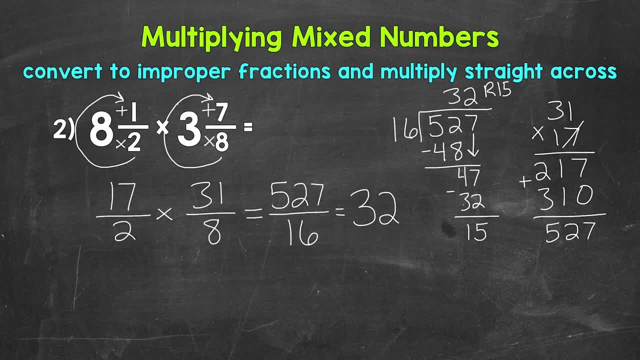 So that's the whole number of our mixed number. And then we have a remainder of fifteen, So that's the numerator of the fractional part. And then we keep the denominator of sixteen the same, So we get thirteen and fifteen-sixteenths. 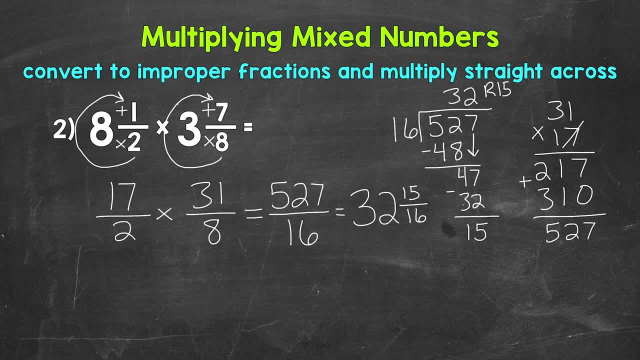 We can check to see if we can simplify the fractional part of the mixed number. Fifteen-sixteenths is in simplest form: the only common factor between fifteen and sixteen is one. So we are done. Final answer: thirty-two and fifteen-sixteenths. 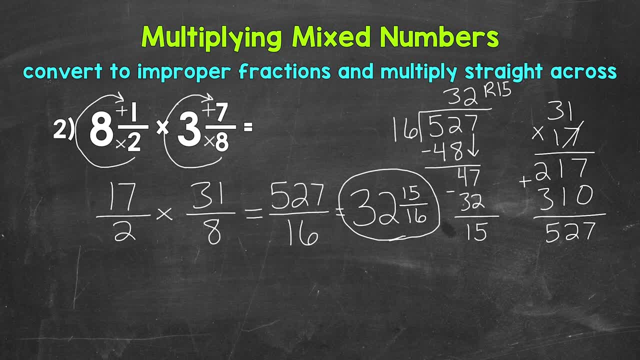 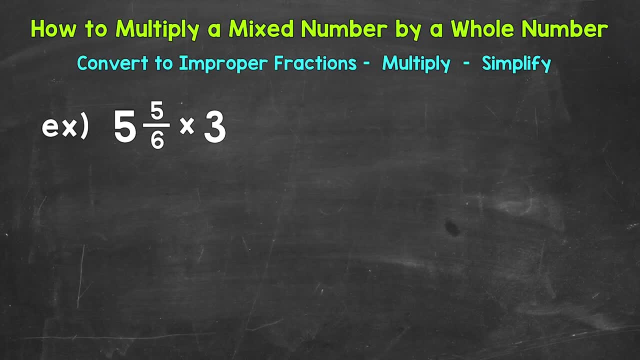 So there you have it. There's how to multiply a mixed number by a mixed number. Let's move on to multiplying a mixed number by a whole number. Now we will take a look at multiplying a mixed number by a whole number. Let's jump into our example, where we have five and five-sixths times three. 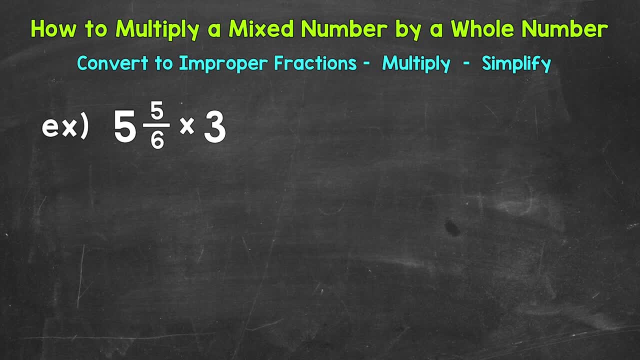 Now the first thing that we want to do, we want to convert our mixed number to an improper fraction and then write our whole number as an improper fraction. Let's start with the mixed number And we start at the bottom and work our way up. 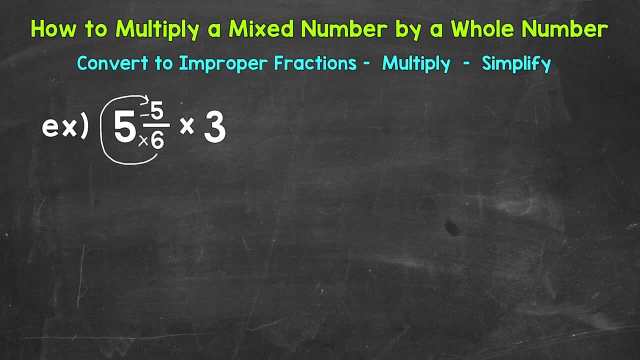 So we multiply and then add. So we do, our denominator times the whole number, So six times five, which is thirty, plus the numerator of five. So thirty plus five is thirty-five. That's the numerator of our improper fraction. We keep the denominator of six the same. 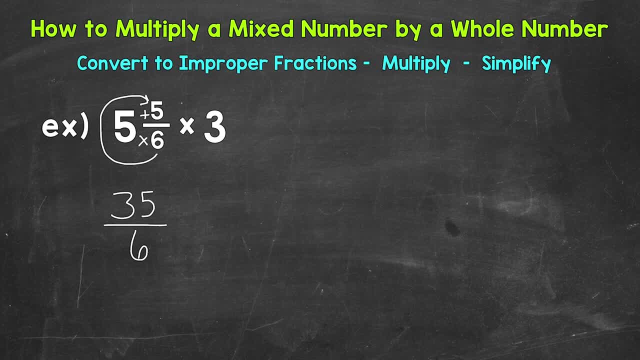 So we get thirty-five over six. Now that improper fraction is equivalent to the mixed number. We just converted it to an improper fraction, So we're not changing the value of the problem at all. Now we need to write our three as a fraction. 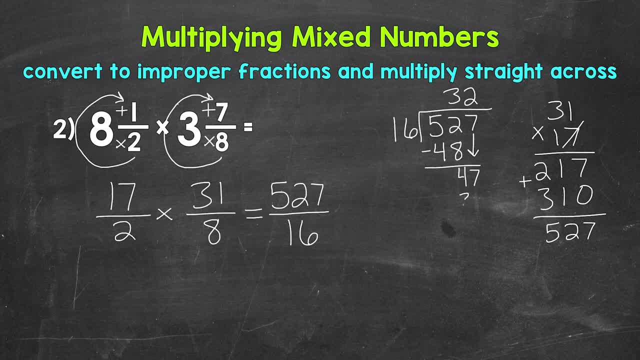 And now we can multiply Two times. sixteen Is thirty two Subtract, And we get fifteen, So thirty two Remainder fifteen, That means Thirty two whole groups of sixteen in five hundred twenty seven. So that's the whole number of our mixed number. 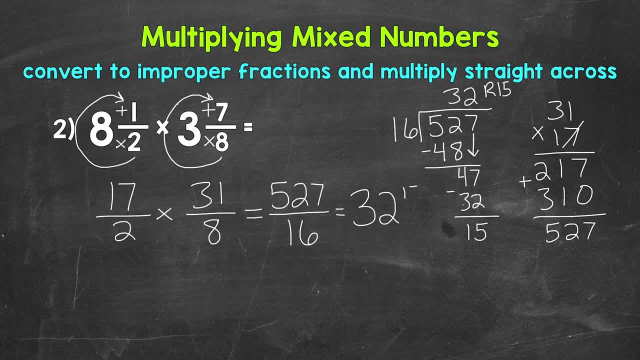 And then we have a remainder of fifteen, So that's the numerator of the fractional part. And then we keep the denominator of sixteen the same, So we get thirteen and fifteen, sixteenths. We can check to see if we can simplify the fractional part of the mixed number. 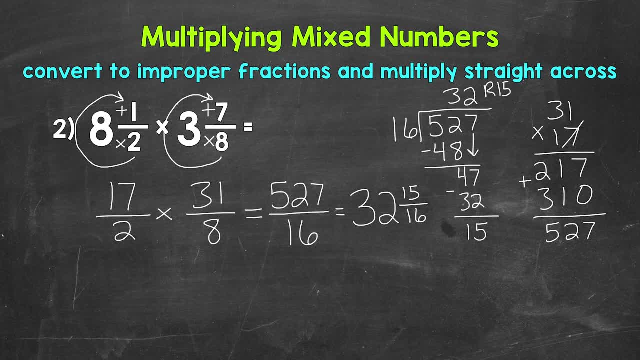 Fifteen sixteenths is in simplest form. The only common factor between fifteen and sixteen is one. So we are done. Final answer: Thirty two and fifteen sixteenths. So there you have it. There's how to multiply a mixed number by a mixed number. 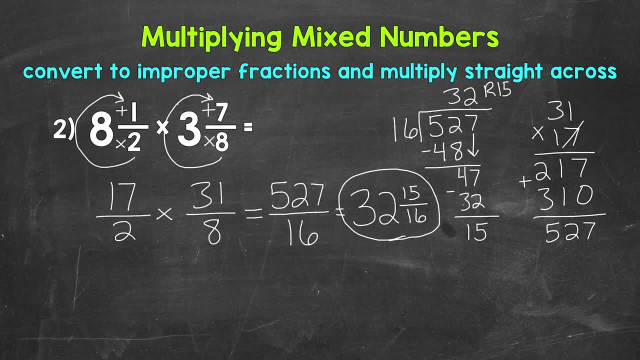 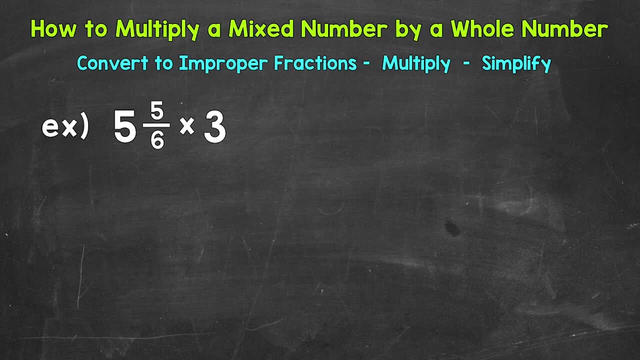 Let's move on to multiplying a mixed number by a whole number. Now we will take a look at multiplying a mixed number by a whole number. Let's jump into our example where we have five and five, sixths times three. Now, the first thing that we want to do, we want to convert our 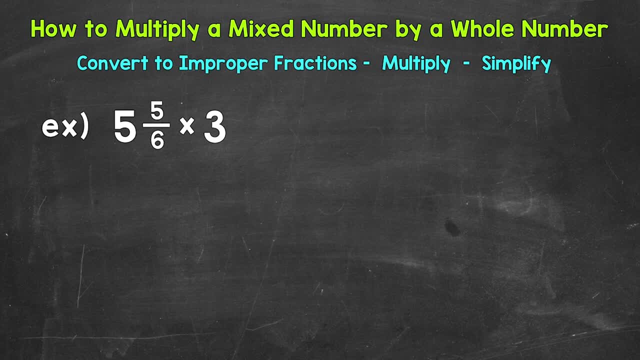 mixed number to an improper fraction and then write our whole number as an improper fraction. Let's start with the mixed number and we start at the bottom and work our way up. So we multiply And then add. So we do our denominator times the whole number. 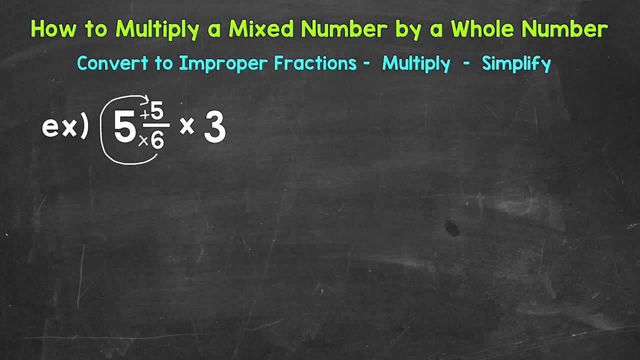 So six times five, which is thirty plus the numerator of five. So thirty plus five is thirty five. That's the numerator of our improper fraction. We keep the denominator of six the same, So we get thirty five over six. Now that improper fraction is equivalent to the mixed number. 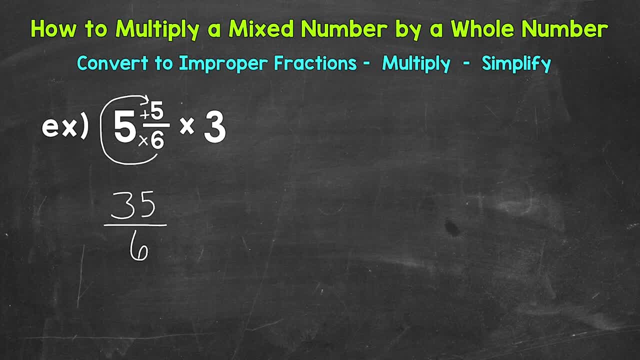 We just converted it to an improper fraction, So we're not changing the value of the problem at all. Now we need to write our three as a fraction, So put it into fractional form, And all we need to do to put a whole number in fractional form is put it over one. 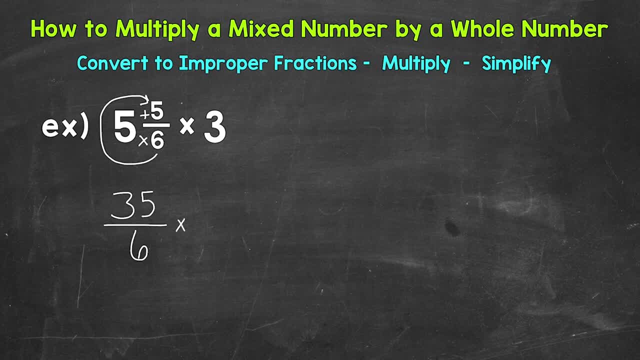 So put it into fractional form, And all we need to do to put a whole number in fractional form is put it over one. We want an improper fraction and the whole number to be in fractional form, So all we have is a top and a bottom. 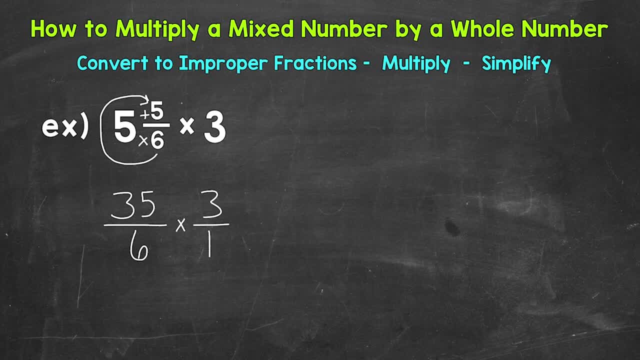 That way we can multiply straight across. So once we're at this point, we can multiply straight across. So, numerator times numerator and denominator times denominator. Let's start with the numerators. So thirty-five times three, Thirty-five times three gives us one hundred five. 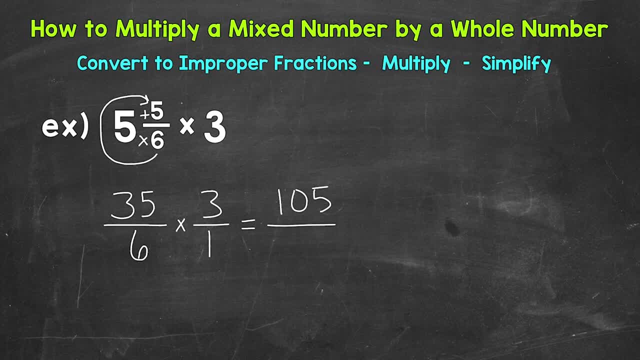 As far as our denominators, we have six times one, which is six. So our answer as an improper fraction, is one hundred five sixths, or one hundred five over six. Now let's convert that to a mixed number, And we do that by dividing our numerator by the denominator. 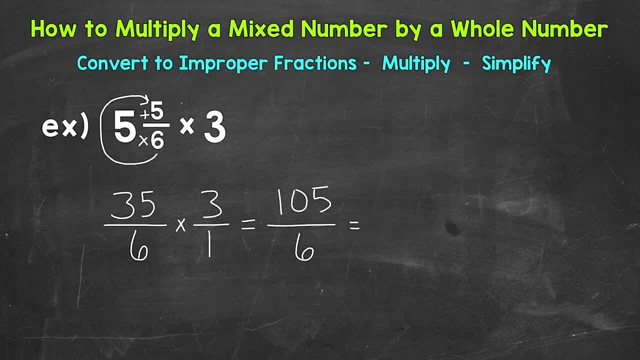 So one hundred five divided by six. I'm going to come to the side here to work through that. So we have one hundred five divided by six. The first thing we need to do we need to find out how many whole groups of six. 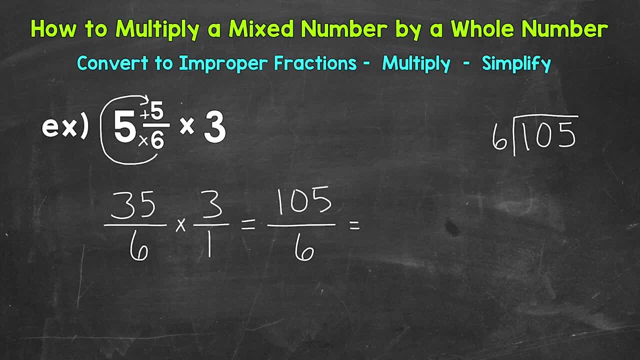 are in one hundred five. That's going to be the whole number, part of our mixed number. So let's start with ten divided by six, How many whole groups of six out of ten? Well, one One times six is six. Subtract Ten minus six is four. 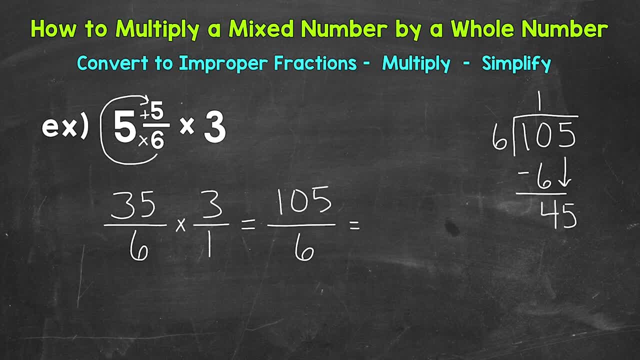 Bring down our five, So we have forty-five divided by six. now, How many whole groups of six out of forty-five? Well, that's going to be seven. That gets us to forty-two. So seven times six is forty-two Subtract. 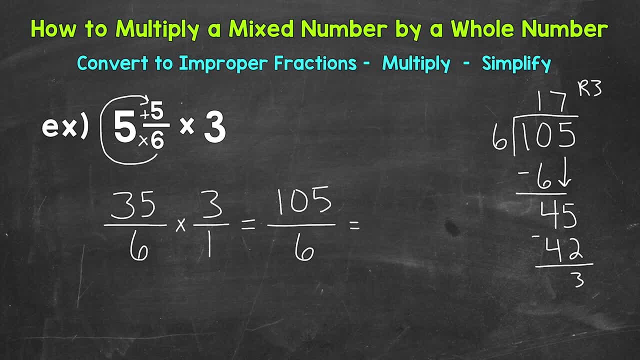 And we get a remainder of three. So we do not hit one hundred five exactly. We have something left over that remainder three. So seventeen whole groups of six out of one hundred five. That's going to be our whole number. portion of the mixed number. 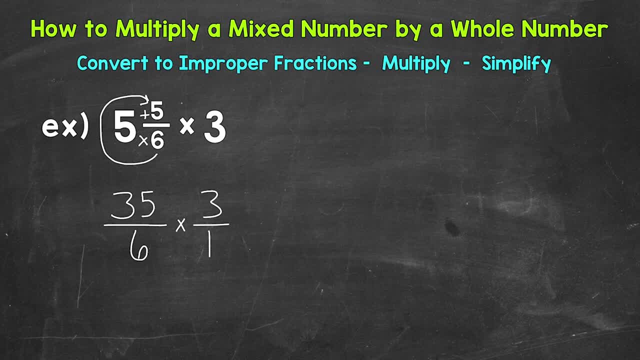 We want an improper fraction and the whole number to be in fractional form. So all we have is a top and a bottom. That way we can multiply straight across. So once we're at this point we can multiply straight across. So: numerator times numerator and denominator times denominator. 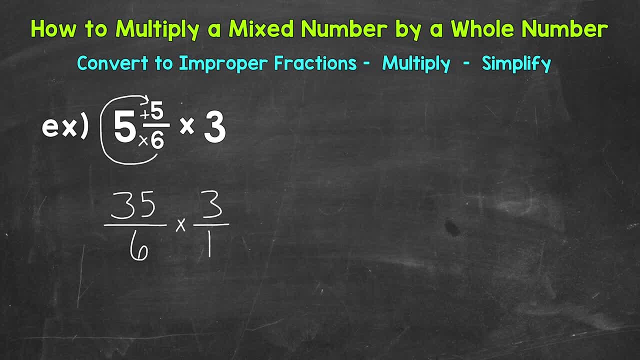 Let's start with the numerators. So thirty five times three, Thirty five times three gives us one hundred five. As far as our denominators, we have six times one, which is six. So our answer as an improper fraction is one hundred five sixths, or one hundred five over six. 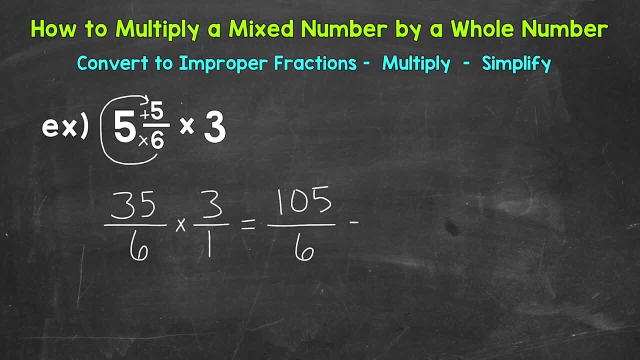 Now let's convert that to a mixed number. We do that by dividing our numerator by the denominator. So one hundred five divided by six. I'm going to come to the side here To work through that. so we have one hundred five divided by six. 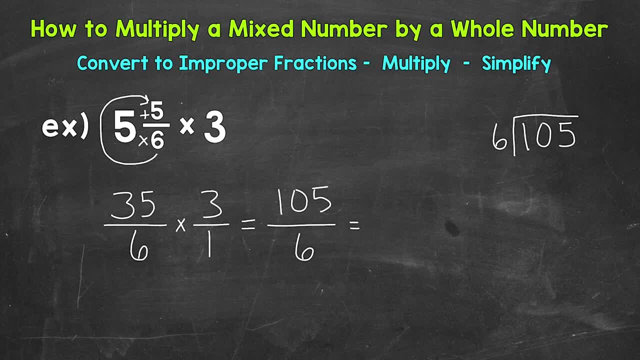 The first thing we need to do, we need to find out how many whole groups of six are in one hundred five. That's going to be the whole number, part of our mixed number. So let's start with ten divided by six: How many whole groups of six out of ten? 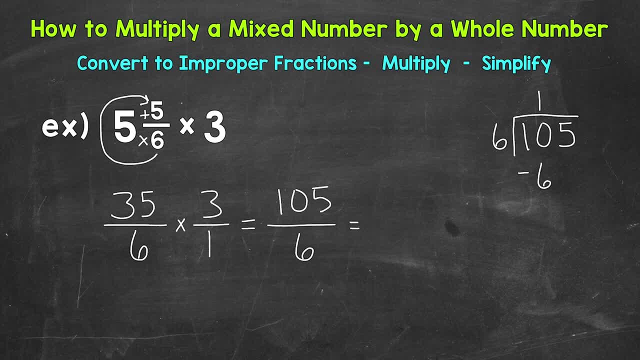 Well, one one times six is six. Subtract ten minus six is four. Bring down our five, So we have forty five divided by six. Now, how many whole groups of six out of forty five? Well, that's going to be seven. 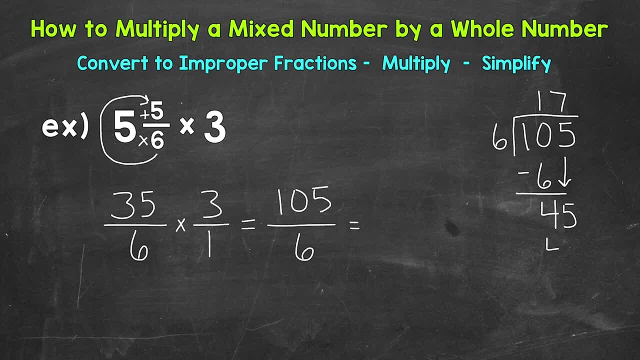 That gets us to forty two. So seven times six is forty two Subtract and we get a remainder of three. We do not hit one hundred five exactly, We have something left over that remainder three. So seventeen whole groups of six out of one hundred five. 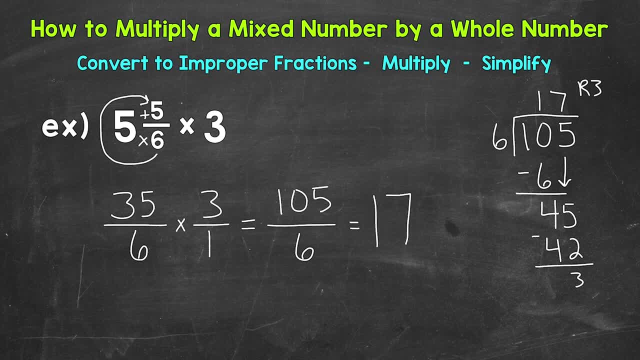 That's going to be our whole number portion of the mixed number. Now we had a remainder of three. That's going to be the numerator of the fractional part of our mixed number. And then we keep our denominator of six the same, So we get. 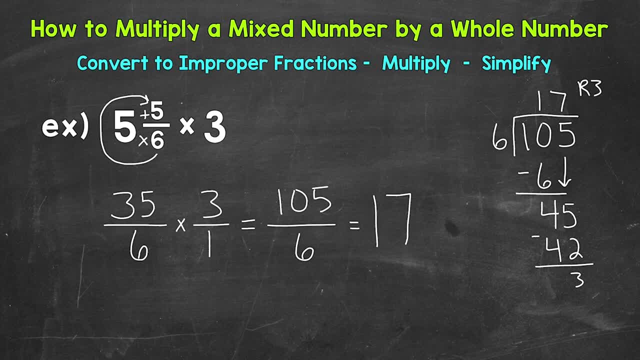 Now we had a remainder of three. That's going to be the numerator of the fractional part of our mixed number, And then we keep our denominator of six the same, So we get seventeen and three-sixths. Always check to see if you can simplify the fractional part of a mixed number. 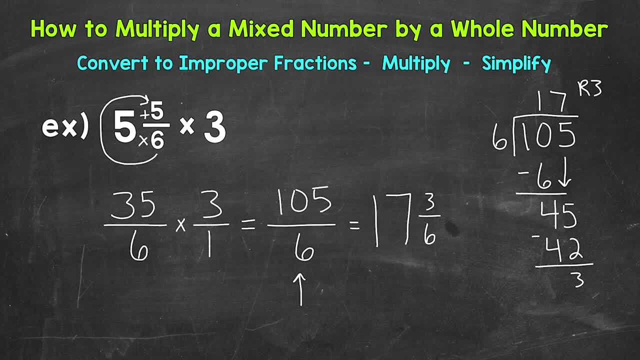 And in this case we can. We have a common factor of three, between three and six. So let's divide both of these by three in order to simplify, And we get seventeen. Three divided by three is one, And then six divided by three is two. 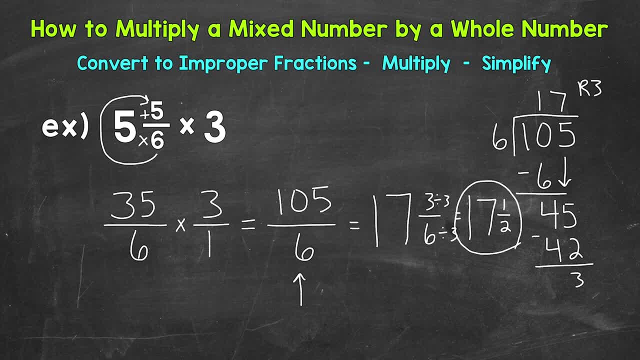 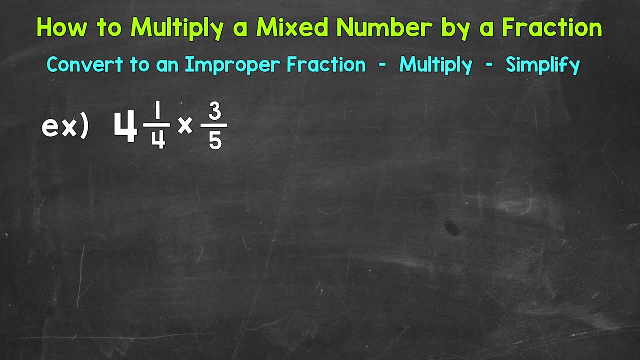 So we get seventeen and a half for our final simplified answer. There's how to multiply a mixed number by a whole number. Let's move on to multiplying a mixed number by a fraction. Now we will take a look at multiplying a mixed number by a fraction. 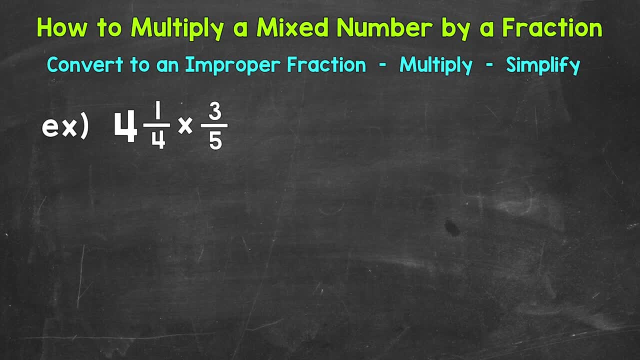 Let's jump into our example where we have four and one-fourth times three-fifths. Now the first thing that we need to do, we need to convert that mixed number to an improper fraction. That way, we just have a numerator and a denominator. 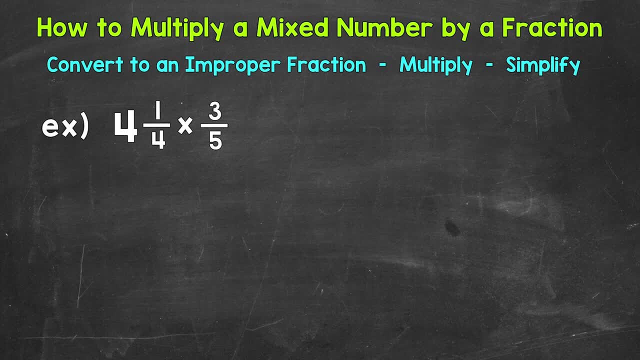 A top and a bottom. So we do that by multiplying and then adding. We start at the bottom and work our way to the top. So we multiply, then add, So our denominator times the whole number. Four times four is sixteen, And then we add the numerator. 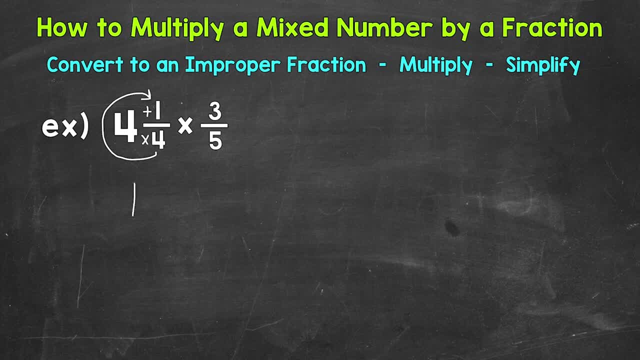 So one Sixteen plus one gives us seventeen. That's the numerator of our improper fraction. And then we keep the denominator of four, the same, Bring down our multiplication sign and then our fraction. At this point we are ready to multiply And we multiply straight across when we multiply fractions. 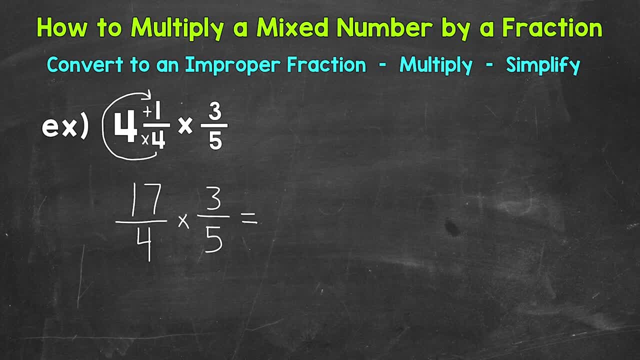 So the numerator, times numerator, and then denominator, times denominator. Let's start with the numerators, the top numbers. So seventeen times three, that gives us fifty-one. Our denominators, the bottom numbers, we have four times five, which gives us twenty. 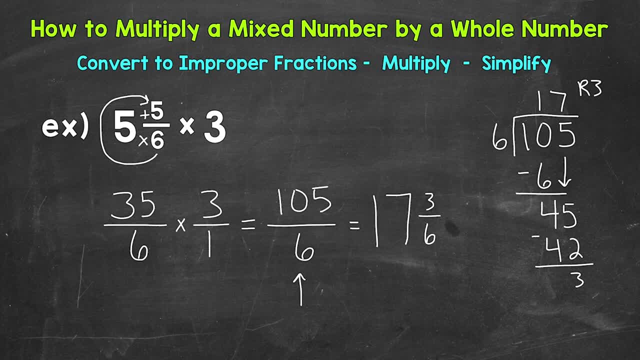 seventeen and three sixths. Always check to see if you can simplify the fractional part of a mixed number, And in this case we can. We have a common factor of three, between three and six, So let's divide both of these by three. 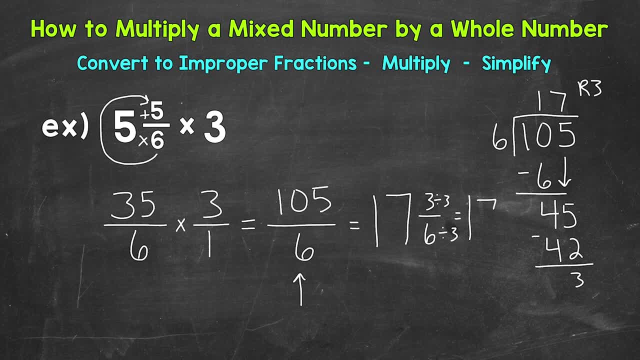 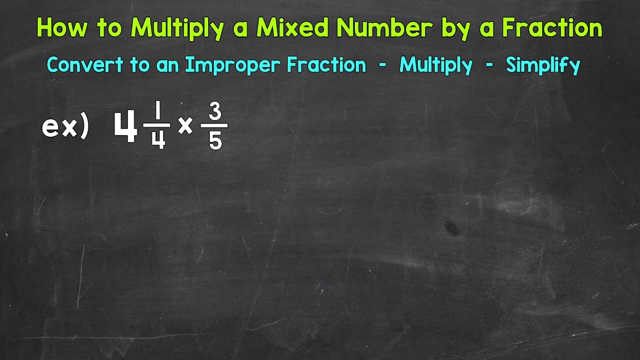 In order to simplify, and we get seventeen. three divided by three is one, and then six divided by three is two, so we get seventeen And a half. for our final simplified answer, There's how to multiply a mixed number by a whole number. Let's move on to multiplying a mixed number by a fraction. 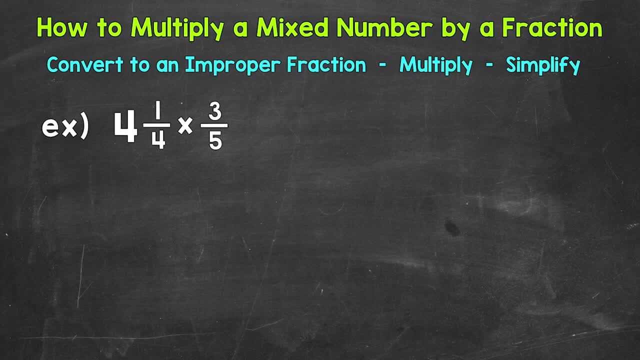 Now we will take a look at multiplying a mixed number by a fraction. Let's jump into our example where we have four and one, fourth times, three, fifths. Now the first thing that we need to do, we need to convert that mixed number to an. 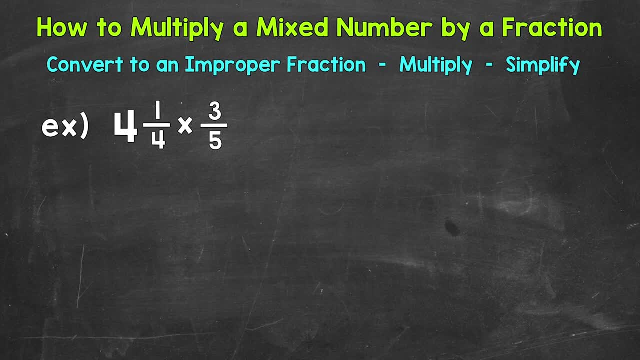 improper fraction. That way we just have a numerator and a denominator, a top and a bottom. So we do that by multiplying and then adding. We start at the bottom and work our way to the top. So we multiply, then add. 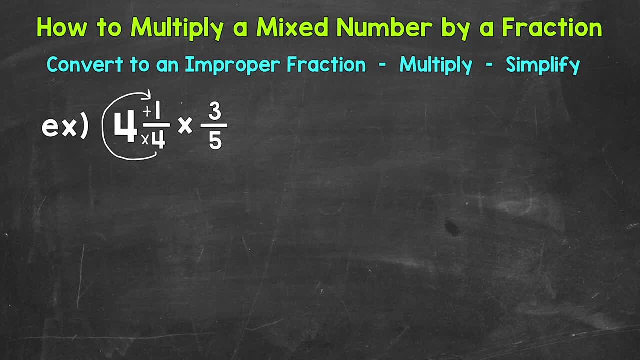 So our denominator times the whole number. four times four is sixteen. And then we add the numerator, So one sixteen plus one gives us seven. That's the numerator of our improper fraction. And then we keep the denominator of four the same, Bring down our multiplication sign and then our fraction. 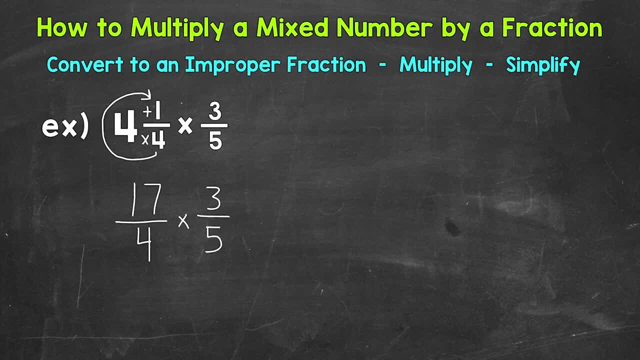 At this point we are ready to multiply And we multiply straight across when we multiply fractions. So the numerator times numerator, and then denominator times denominator. Let's start with the numerators, the top numbers. So seventeen times three, Seventeen times three. 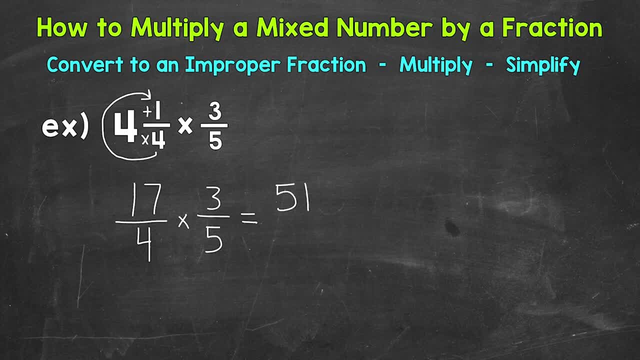 That gives us fifty-one. Our denominators, the bottom numbers, we have four times five, which gives us twenty. So we get to fifty-one, twentieths, And that's our final answer. as an improper fraction Now we can convert that to a mixed number. 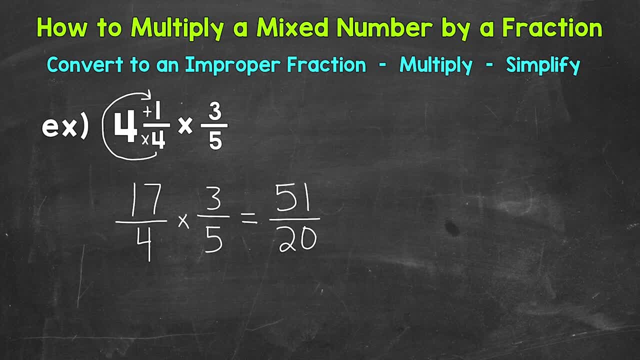 So we get to fifty-one-twentieths, And that's our final answer as an improper fraction. Now we can convert that to a mixed number. We do that by dividing. We divide our numerator fifty-one by our denominator twenty. 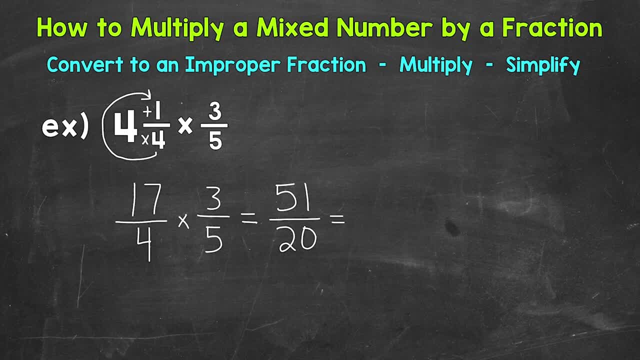 So we need to think: how many whole groups of twenty can we pull out of fifty-one? Well, two That gets us to forty. Now we do not hit fifty-one exactly. We have something left over, a remainder. So if we pull two whole groups of twenty out of fifty-one, 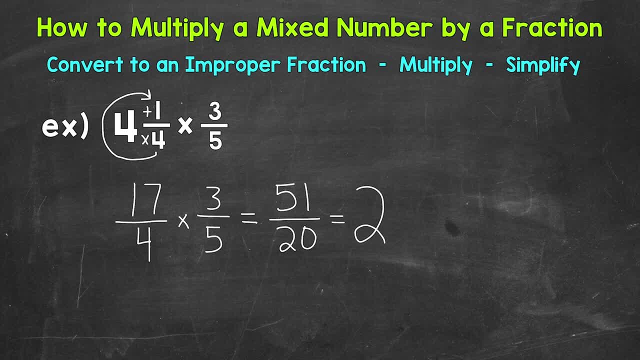 that's pulling forty out of fifty-one. So we have a remainder of eleven. That's the numerator of our mixed number, And we keep our denominator of twenty the same. So, to recap, I'm going to write this out off to the side. 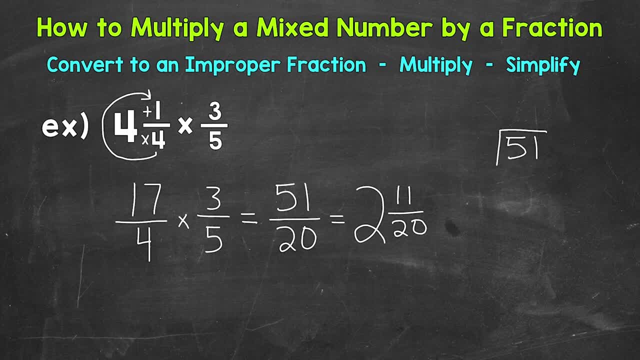 We did fifty-one divided by twenty. So how many whole groups of twenty out of fifty-one? Well, two, That's the whole number. part of our mixed number. Two times twenty is forty. So let's subtract to get our remainder. Fifty-one minus forty is eleven. 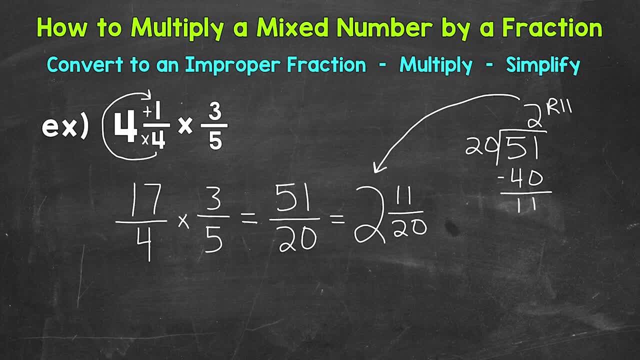 So we get two remainder eleven. That remainder of eleven is the numerator part of the fractional part of the mixed number. And then we keep our denominator of twenty the same. Always check to see if you can simplify the fractional part of a mixed number. 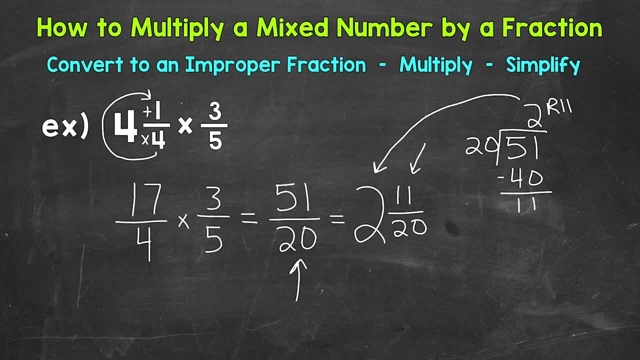 Eleven-twentieths is in simplest form. The only common factor between eleven and twenty is one. So we are done Four and one-fourth times three-fifths equals two and eleven-twentieths. There's how to multiply a mixed number by a fraction. 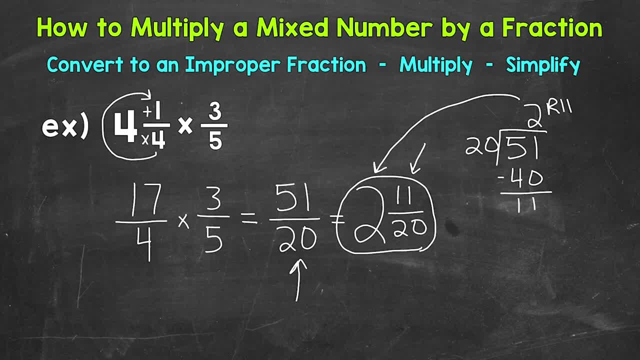 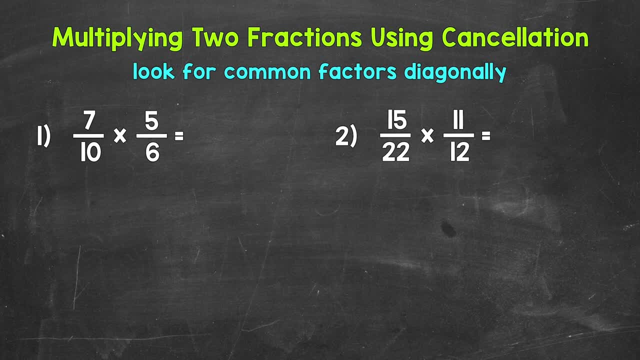 Let's move on to how to use cancellation when multiplying fractions. Now we will take a look at using cancellation, which is called cross cancellation, when multiplying two fractions. Cancellation is a way to simplify a problem before we multiply. Now remember when we multiply fractions. 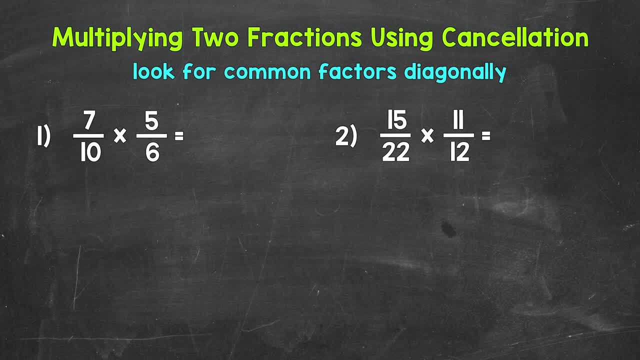 we multiply straight across. So multiply the numerators- the top numbers- and then multiply the denominators- the bottom numbers. We use cancellation before we multiply straight across. This strategy gives us smaller numbers in value to work with and easier numbers to work with. 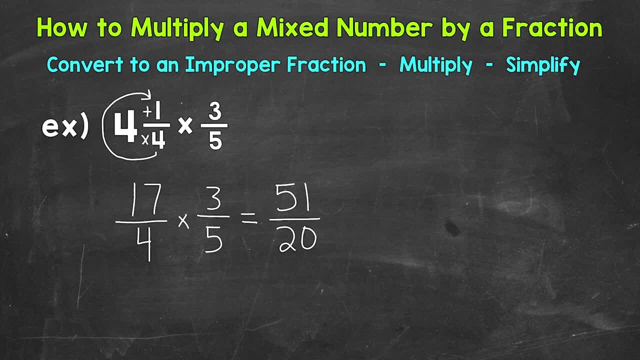 We do that by dividing. We divide our numerator fifty-one by our denominator twenty. So we need to think: How many whole groups of twenty can we pull out of fifty-one? Well, two That gets us to forty. Now we do not hit fifty-one exactly. 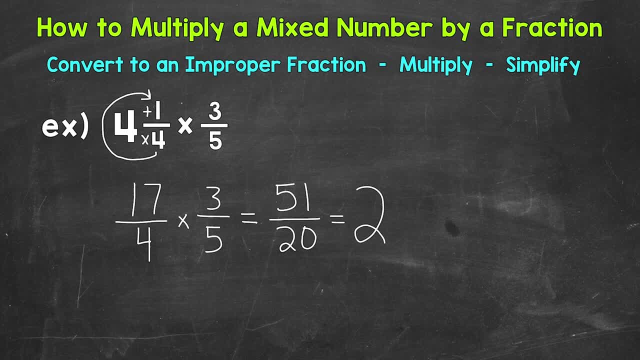 We have something left over, a remainder. So if we pull two whole groups of twenty out of fifty-one, that's pulling forty out of fifty-one, So we have a remainder of eleven. That's the numerator of our mixed number And we keep our denominator of twenty the same. 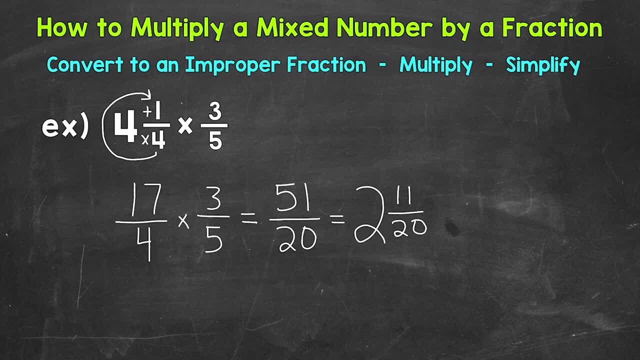 So, to recap- I'm going to write this out off to the side- We did fifty-one divided by twenty. So how many whole groups of twenty out of fifty-one? Well, two, That's the whole number, part of our mixed number. 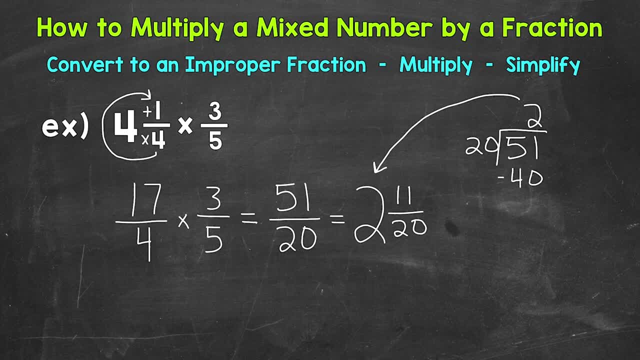 Two times twenty is forty. So let's subtract to get our remainder. Fifty-one minus forty is eleven, So we get two remainder eleven. That remainder of eleven is the numerator part of the fractional part of the mixed number. And then we keep our denominator of twenty the same. 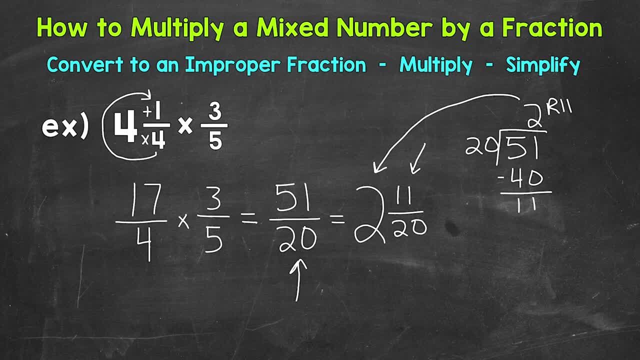 Always check to see if you can simplify the fractional part of a mixed number. Eleven twentieths is in simplest form: The only common factor between eleven and twenty is one. So we are done Four and one. fourth times three fifths equals two and eleven. 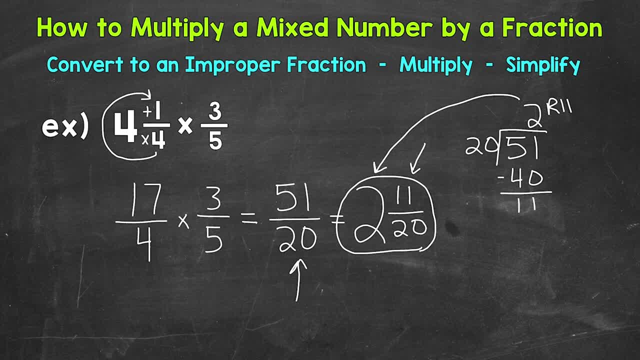 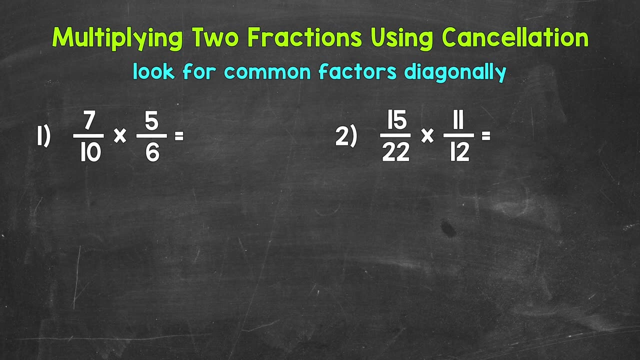 Eleven, twentieths. There's how to multiply a mixed number by a fraction. Let's move on to how to use cancellation when multiplying fractions. Now we will take a look at using cancellation, also called cross cancellation, when multiplying two fractions. Cancellation is a way to simplify a problem before we multiply. 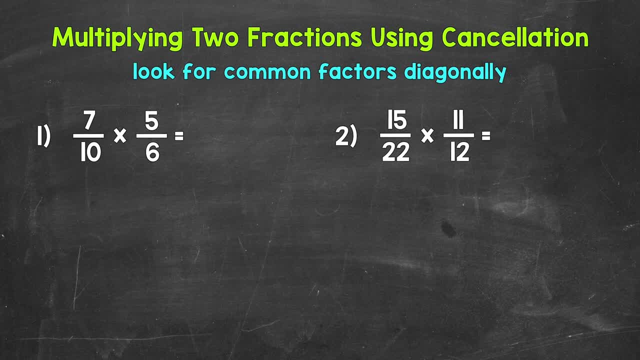 Now remember: when we multiply fractions, we multiply straight across. So multiply the numerators- The top numbers- and then multiply the denominators- the bottom numbers. We use cancellation before we multiply straight across. This strategy gives us smaller numbers in value to work with and easier numbers to work with. 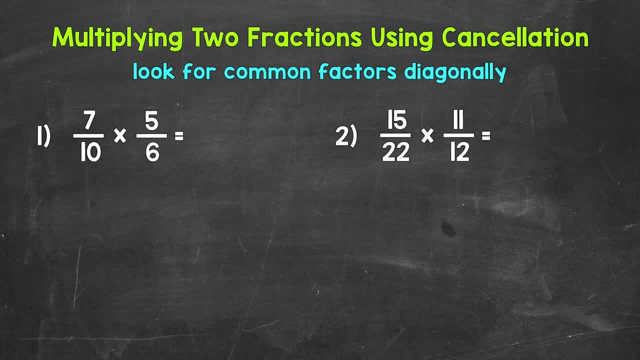 Let's jump into our examples, starting with number one, where we have seven tenths times five sixths When we use cancellation. again, we need to look to simplify the problem. before we multiply, Look for common factors other than one diagonally. 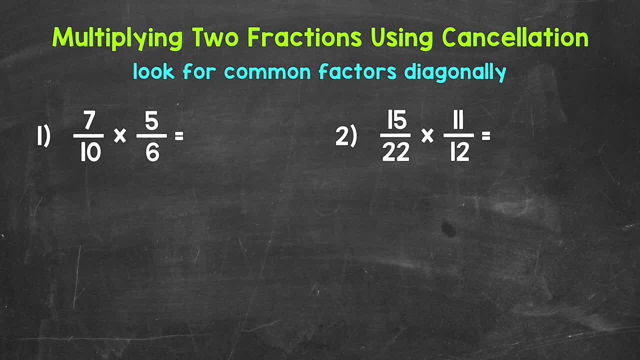 That way, we can divide those numbers by that common factor. in order to simplify the problem, before multiplying, Think of it like simplifying fractions, but we are looking diagonally, So let's look at seven and six first. Are there any common factors between seven and six other than one? 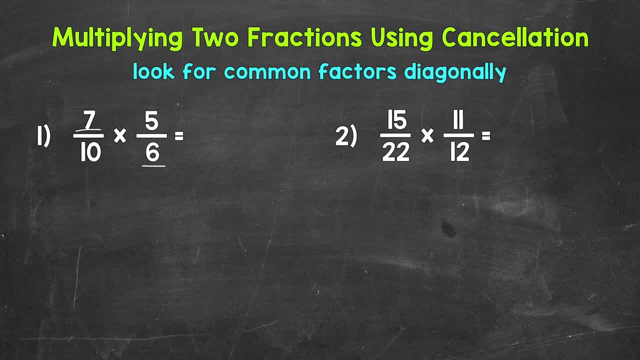 No, The only common factor is one, So we can't use cancellation with the seven and the six. Now let's take a look at the ten and the five. Are there any common factors other than one between ten and five? Yes, Five is a common factor and it happens to be the greatest common factor. 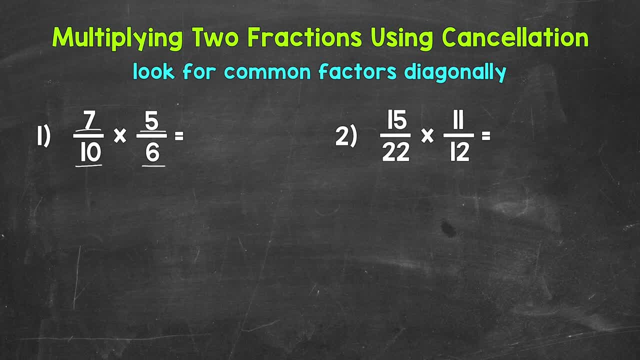 So let's divide ten and five by five. So ten divided by five gives us two. Five divided by five gives us one. Now we have a simpler problem. We have smaller numbers in value to work with, So let's multiply straight across. 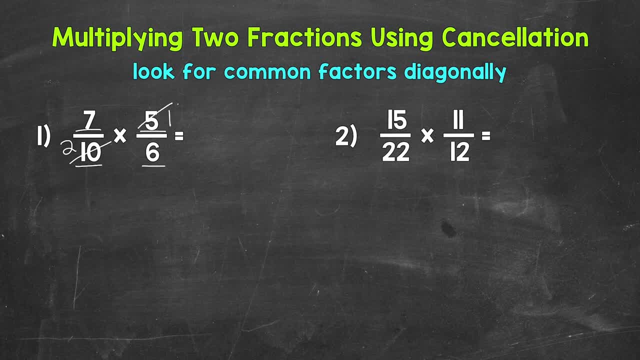 Now, starting with the numerators: seven times one is seven. Now for the denominators: two times six gives us twelve. Seven, twelfths is our final answer, and it is in simplest form. The only common factor between seven and twelve is one. 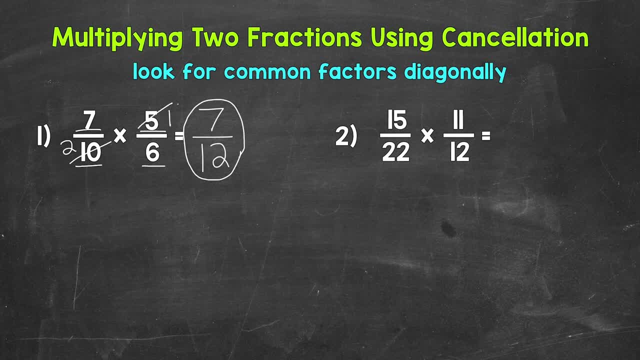 So we are done: Seven twelfths. Now let's go through that problem without using cancellation in order to see the difference. So we have seven tenths times five sixths. So let's multiply straight across again without using cancellation. We will start with the numerators. 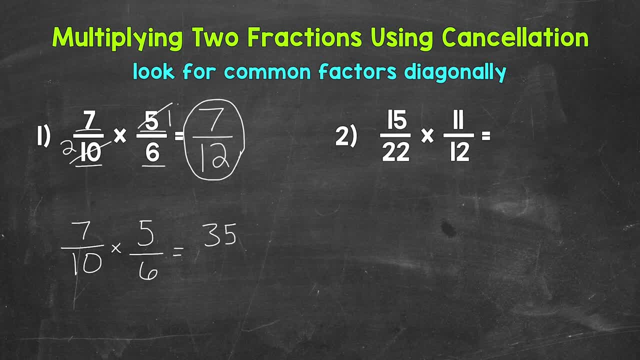 So seven times five is thirty-five. Now for the denominators, ten times six is sixty. So we get thirty-five sixtieths, which is different than when we used cancellation. Well, thirty-five sixtieths isn't in simplest form. 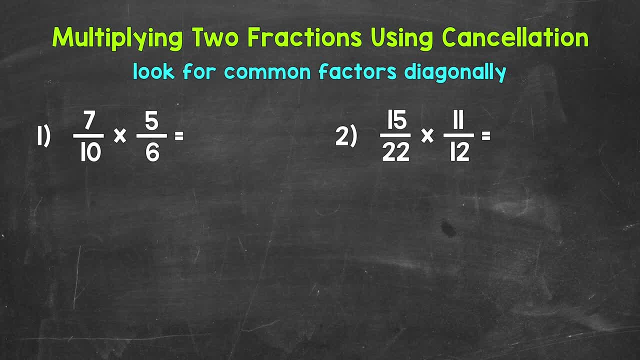 Let's jump into our examples, starting with number one, where we have seven-tenths times five-sixths When we use cancellation. again, we need to look to simplify the problem. before we multiply, Look for common factors other than one diagonally. 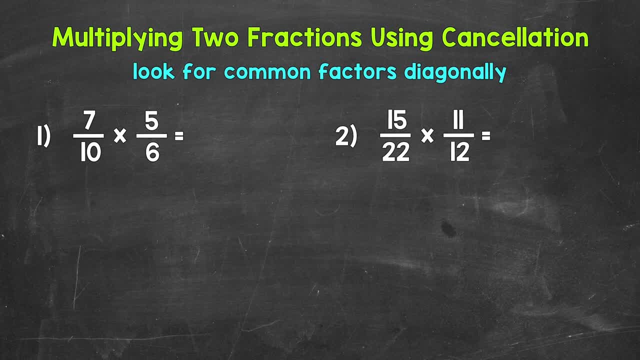 That way, we can divide those numbers by that common factor. in order to simplify the problem, before multiplying, Think of it like simplifying fractions, but we are looking diagonally, So let's look at seven and six first. Are there any common factors between seven and six other than one? 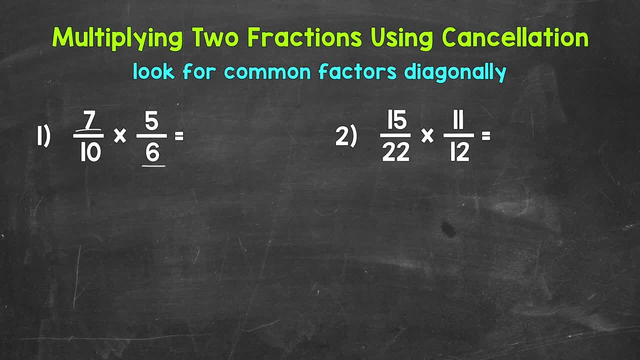 No, the only common factor is one, so we can't use cancellation with the seven and the six. Now let's take a look at the ten and the five. Are there any common factors other than one between ten and five? Yes, five is a common factor. 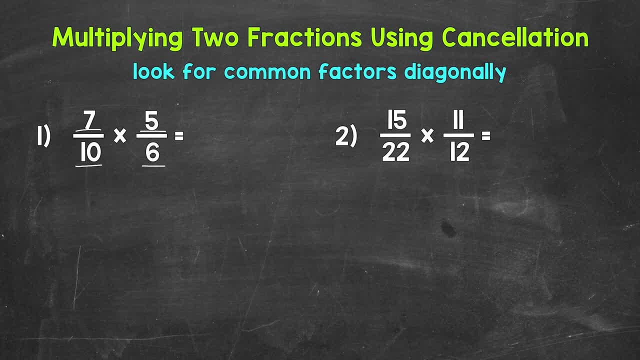 and it happens to be the greatest common factor. So let's divide ten and five by five. So ten divided by five gives us two. Five divided by five gives us one. Now we have a simpler problem. We have smaller numbers in value to work with. 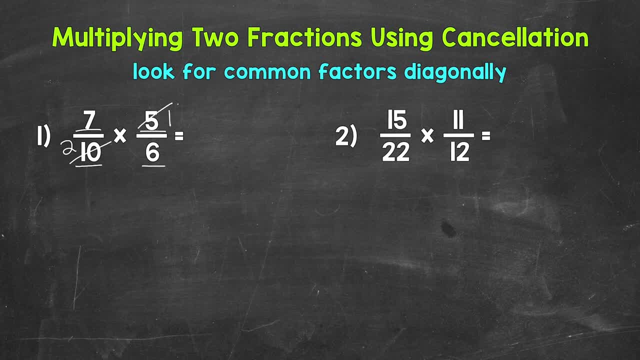 So let's multiply straight across now, starting with the numerators: Seven times one is seven. Now for the denominators: Two times six gives us twelve. Seven, twelfths is our final answer, and it is in simplest form. The only common factor between seven and twelve is one. 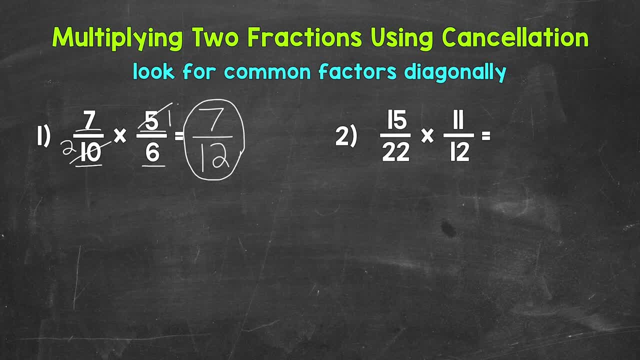 So we are done: Seven twelfths. Now let's go through that problem without using cancellation In order to see the difference. So we have seven tenths times five sixths. So let's multiply straight across again without using cancellation. We will start with the numerators. 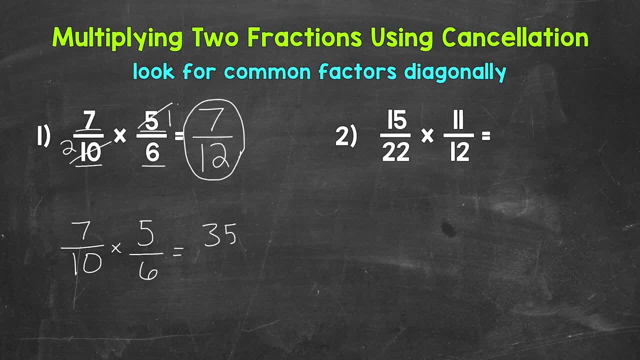 So seven times five is thirty-five. Now for the denominators, Ten times six is sixty, So we get thirty-five sixtieths, Which is different than when we used cancellation. Well, thirty-five sixtieths isn't in simplest form. 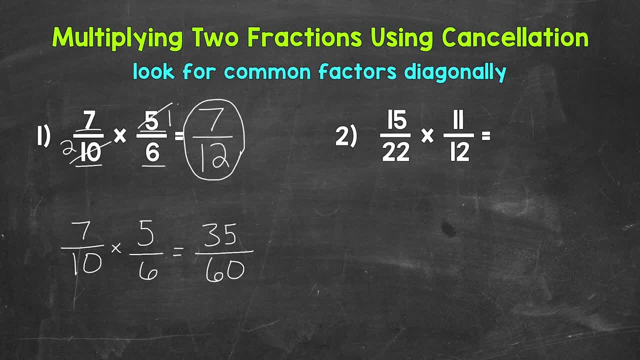 So let's simplify. Are there any common factors between thirty-five and sixty other than one? Yes, Five, And five is the greatest common factor. So let's divide thirty-five and sixty by five in order to simplify. Thirty-five divided by five is seven. 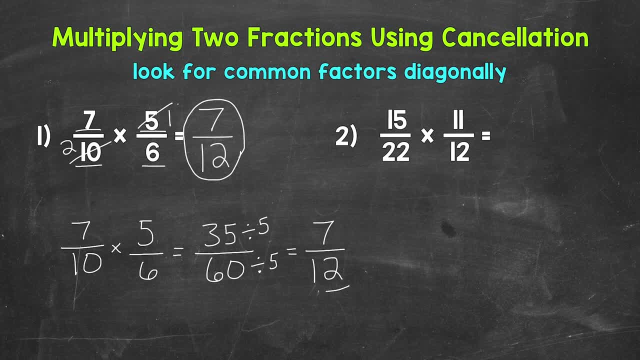 Sixty divided by five is twelve. So our final simplified answer: seven twelfths. The only common factor between seven and twelve is one. So that is in simplest form and we are done. So we get seven twelfths that way as well. 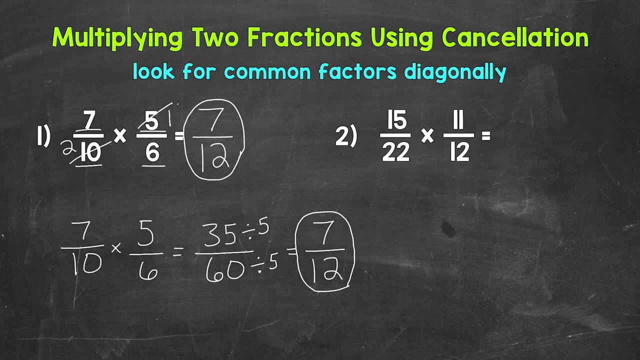 So do we have to use cancellation in order to multiply fractions? No, but it is a good strategy to be familiar with and use when possible. It can be helpful. Let's move on to number two, where we have fifteen, twenty seconds times eleven, twelfths. 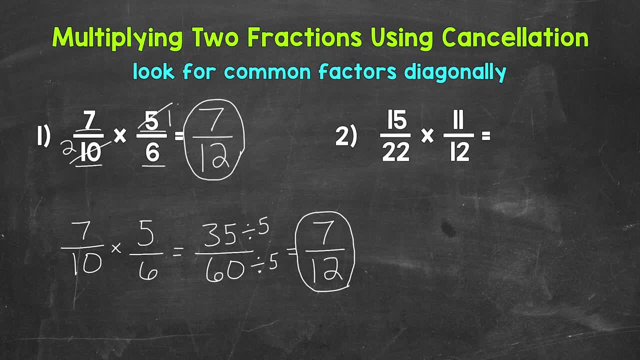 Let's look to use cancellation. And again, we look diagonally. So let's take a look at fifteen and twelve. First, do we have any common factors other than one? Yes, three is a common factor and the greatest common factor. 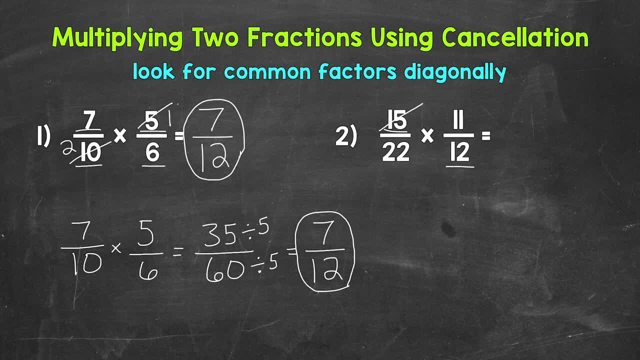 So let's divide them both by three. Fifteen divided by three is five. Twelve divided by three is four. Now let's take a look at twenty-two and eleven. Are there any common factors other than one between twenty-two and eleven? Yes, eleven. 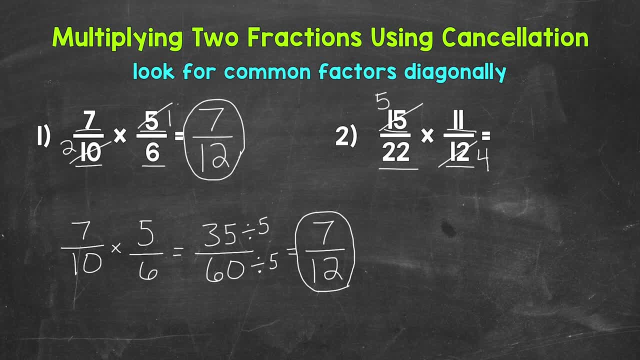 And eleven is the greatest common factor. So let's divide twenty-two by eleven: That gives us two. And then eleven divided by eleven, That gives us one. Now we can multiply straight across And you can see that we have much simpler and easier numbers to work with when we multiply straight across. 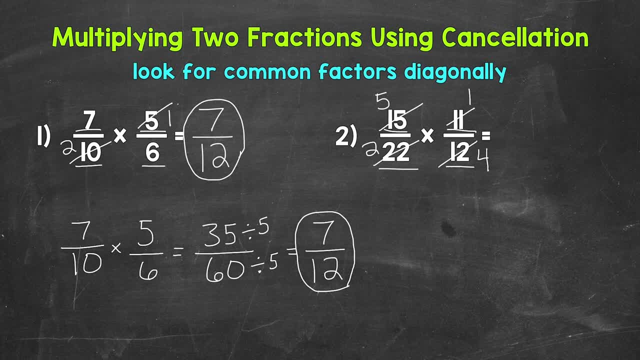 So let's start with the numerators. Five times one gives us five. Now for the denominator: Two times four gives us eight. So we get five-eighths. The only common factor between five and eight is one. So we are in simplest form and we are done. 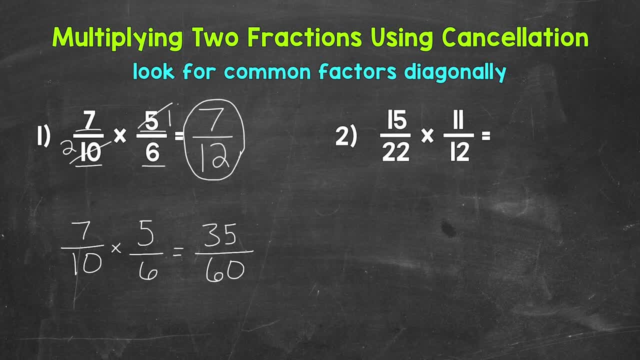 So let's simplify. Are there any common factors between thirty-five and sixty other than one? Yes, five, and five is the greatest common factor. So let's divide thirty-five and sixty by five in order to simplify. Thirty-five divided by five is seven. 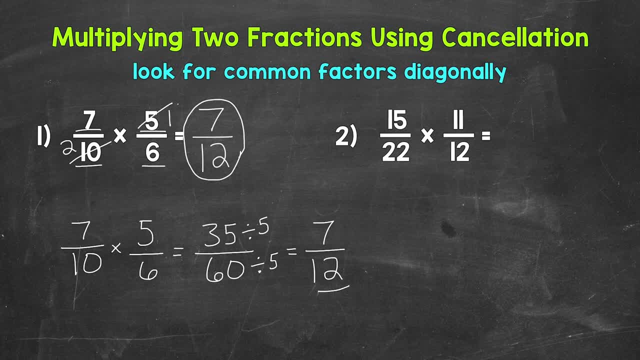 Sixty divided by five is twelve. So our final simplified answer: seven twelfths. The only common factor between seven and twelve is one. So that is in simplest form and we are done. So we get seven twelfths that way as well. 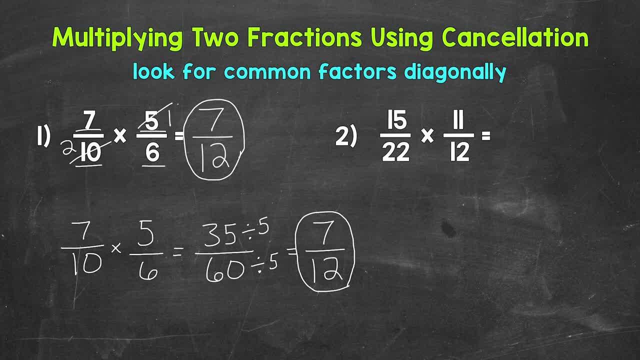 So do we have to use cancellation in order to multiply fractions? No, but it is a good strategy to be familiar with and use when possible. It can be helpful. Let's move on to number two, where we have fifteen, twenty-seconds times, eleven, twelfths. 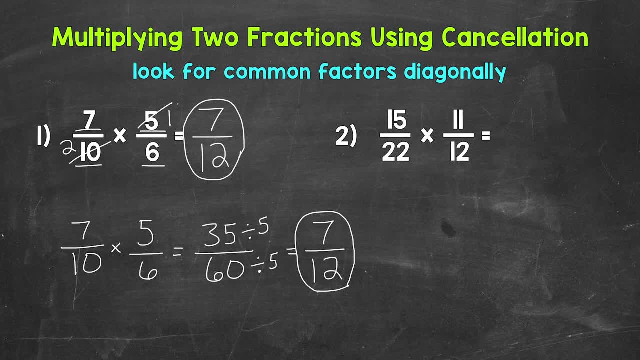 Let's look to use cancellation. And again, we look diagonally. So let's take a look at fifteen and twelve first. Do we have any common factors other than one? Yes, three is a common factor, and the greatest common factor, So let's divide them both by three. 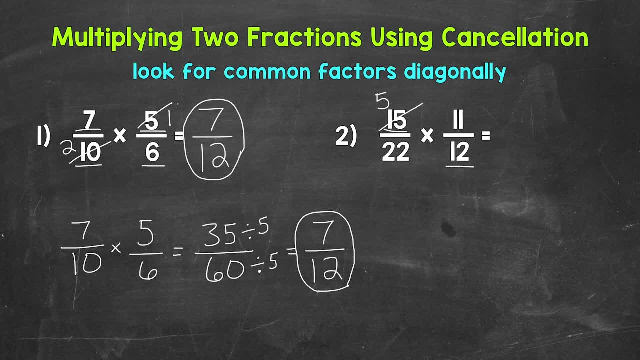 Fifteen divided by three is five. Twelve divided by three is four. Now let's take a look at twenty-two and eleven. Are there any common factors other than one between twenty-two and eleven? Yes, eleven And eleven is the greatest common factor. 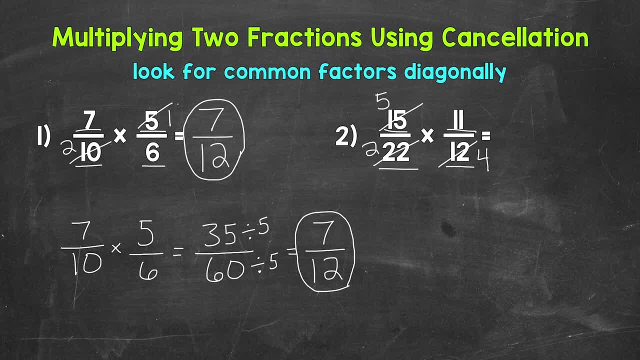 So let's divide twenty-two by eleven: That gives us two. And then eleven divided by eleven, That gives us one. Now we can multiply straight across And you can see that we have much simpler and easier numbers to work with when we multiply straight across. 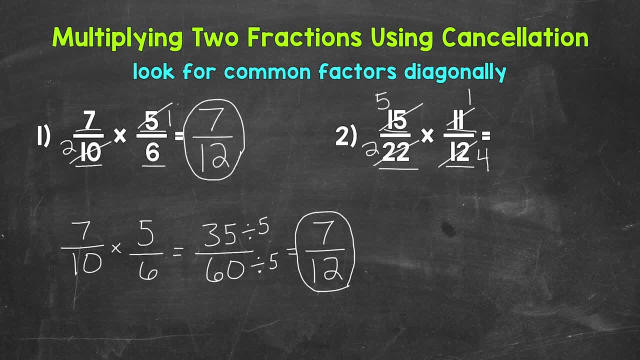 So let's start with the numerators. Five times one gives us five. Now for the denominators: Two times four gives us eight. So we get five-eighths. The only common factor between five and eight is one. So we are in simplest form. 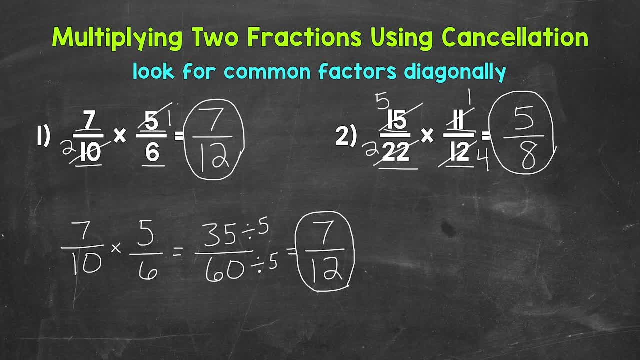 And we are done For number two. that problem was much simpler to work through after we used cancellation. We had five times one and two times four instead of fifteen times eleven and twenty-two times twelve. Now did we have to use cancellation? No, we could have gone straight across and done fifteen times eleven and then twenty-two times twelve, and then simplified. 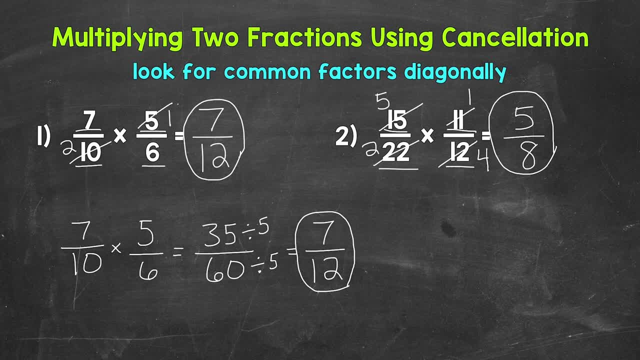 But the cancellation made it easier and simpler as far as multiplying straight across. So understanding cancellation and how to use it can be helpful when multiplying fractions. There's how to use cancellation when multiplying two fractions. Let's move on to using cancellation when multiplying mixed numbers. 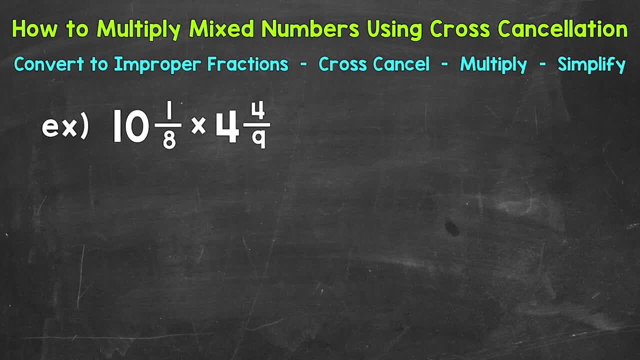 Now we will take a look at using cancellation when multiplying mixed numbers. Let's jump into our example where we have ten and one-eighth times four and four-ninths. Now the first thing that we need to do, we need to convert these mixed numbers to improper fractions. 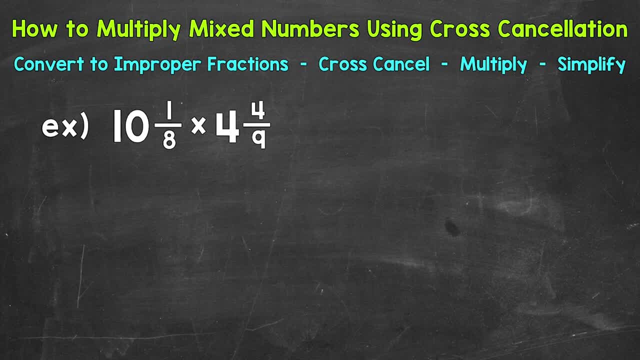 That way we just have a numerator and a denominator. We'll start with ten and one-eighth, So let's go from the bottom and work our way to the top. So we multiply and then add, We do our denominator times the whole number. 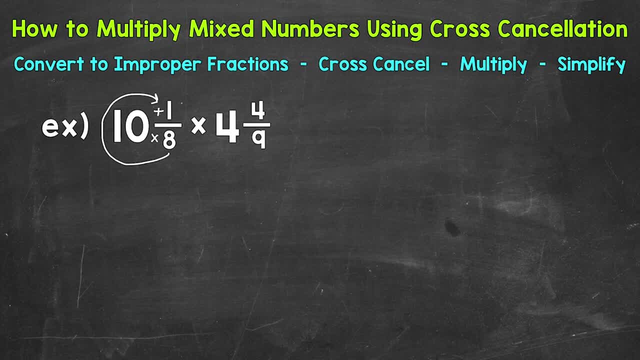 So eight times ten, which is eighty, plus our numerator, which is one. So eighty plus one is eighty-one. That's our numerator of the improper fraction. We keep our denominator of eight the same. We'll bring our multiplication sign down and then convert our second mixed number. 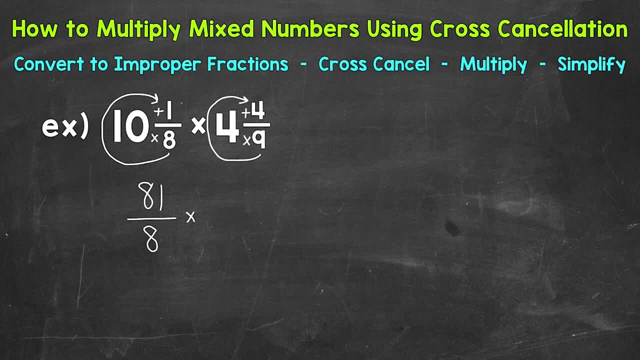 Start at the bottom. we multiply and then add. So nine times four is thirty-six Plus four is forty. So that's our numerator and we keep our denominator of nine the same, So we have eighty-one-eighths times forty-ninths. 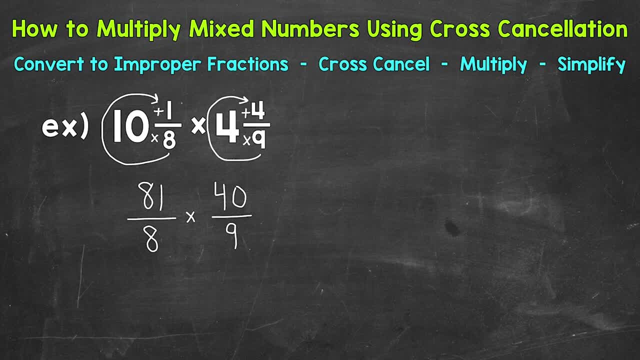 Eighty-one-eighths is equivalent to ten and one-eighth. It's just in the form of an improper fraction. And then ten and one-eighth is in the form of a mixed number. Both of those are equivalent. So when we convert to an improper fraction, 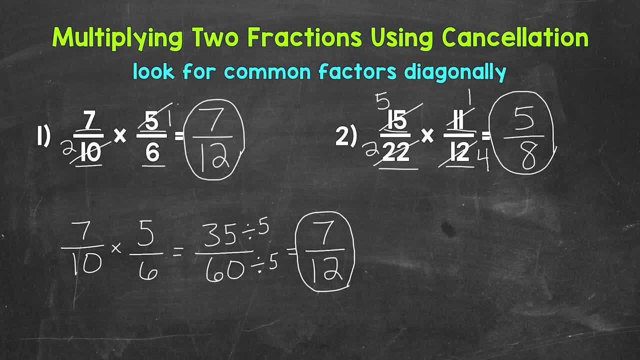 For number two. that problem was much simpler to work through after we used cancellation. We had five times one and two times four, instead of fifteen times eleven and twenty-two times twelve. Now did we have to use cancellation? No, we could have gone straight across and done fifteen times eleven and then twenty-two times twelve, and then simplified. 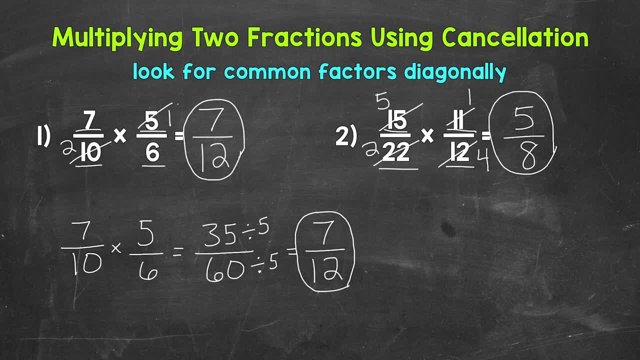 But the cancellation made it easier and simpler as far as multiplying straight across. So understanding cancellation and how to use it can be helpful when multiplying fractions. There's how to use cancellation when multiplying two fractions. Let's move on to using cancellation when multiplying mixed numbers. 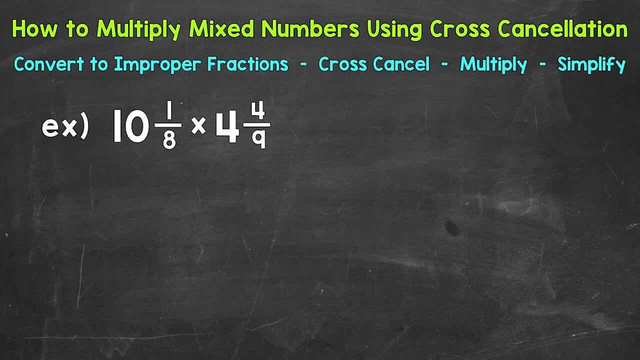 Now we will take a look at using cancellation when multiplying mixed numbers. Let's jump into our example where we have ten and one-eighth times four and four-ninths. Now the first thing that we need to do, we need to convert these mixed numbers to improper fractions. 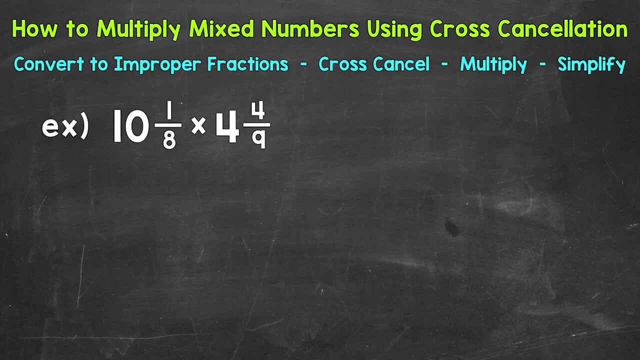 That way we just have a numerator and a denominator. We'll start with ten and one-eighth, So let's go from the bottom and work our way to the top. So we multiply and then add, We do our denominator times the whole number. 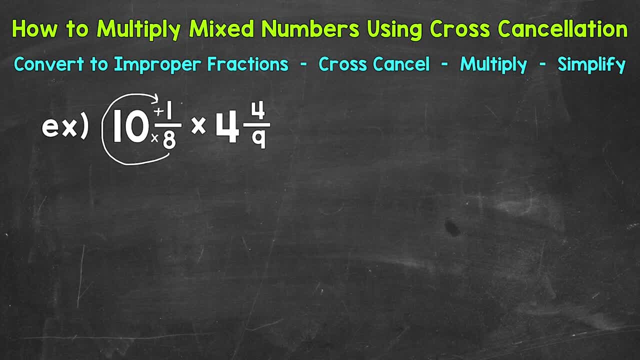 So eight times ten, which is eighty, plus our numerator, which is one. So eighty plus one is eighty-one. That's our numerator of the improper fraction. We keep our denominator of eight the same. We'll bring our multiplication sign down and then convert. 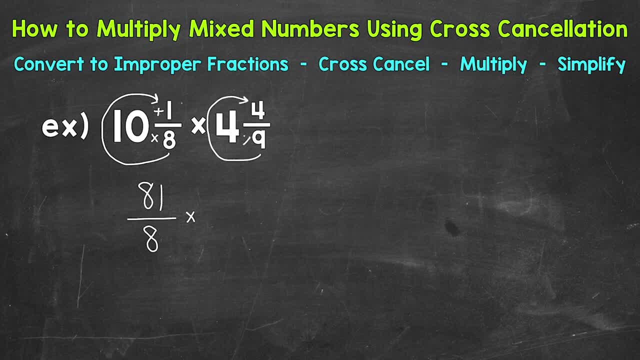 our second mixed number Start at the bottom. We multiply and then add. So nine times four is thirty-six plus four is forty. So that's our numerator And we keep our denominator of nine the same. So we have eighty-one-eighths times forty-ninths. 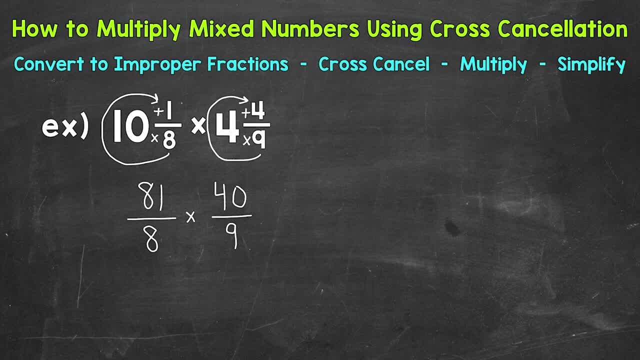 Eighty-one-eighths is equivalent to ten and one-eighth. It's just in the form of an improper fraction. And then ten and one-eighth is in the form of a mixed number. Both of those are equivalent. So when we convert to an improper fraction, 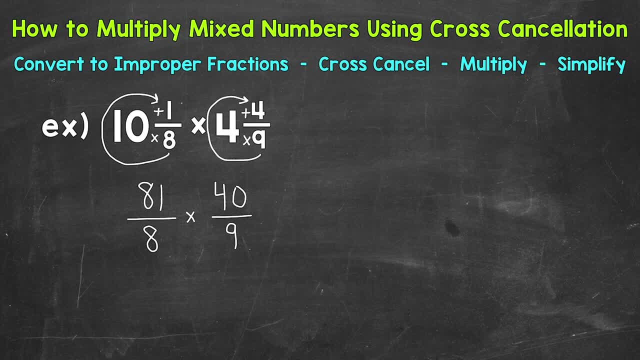 we're not changing the value of anything. And then forty-ninths is equivalent to four, and four-ninths Again. we did this. so we just have a numerator and a denominator and we are able to multiply. At this point we can multiply straight across. 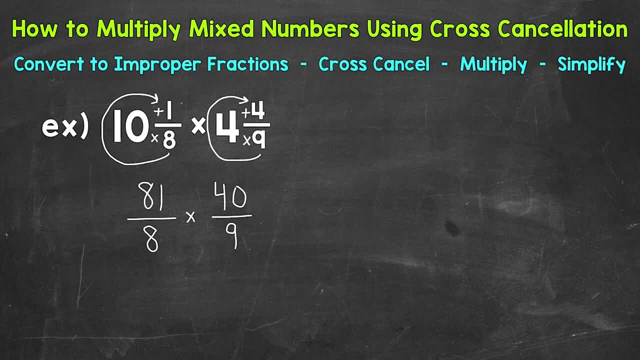 So we can do eighty-one times forty and then eight times nine, But we can use cross cancellation and this is a way to simplify fractions before multiplying. It gives us smaller and easier numbers to work with, Therefore a simpler problem to solve. 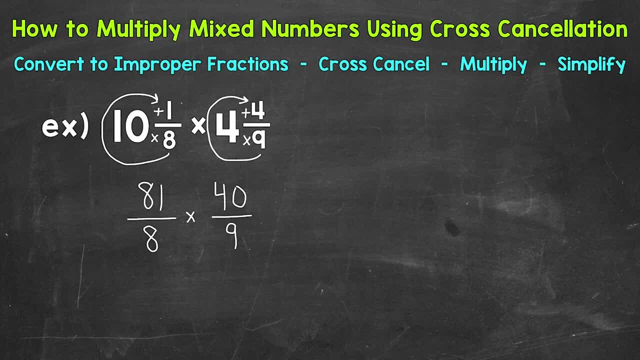 We cross cancel by looking for common factors between the numerators and denominators, So the top and bottom. Think of it as simplifying fractions. but we can look diagonally as well. For example, we have eighty-one and nine, So eighty-one right here and nine diagonally. 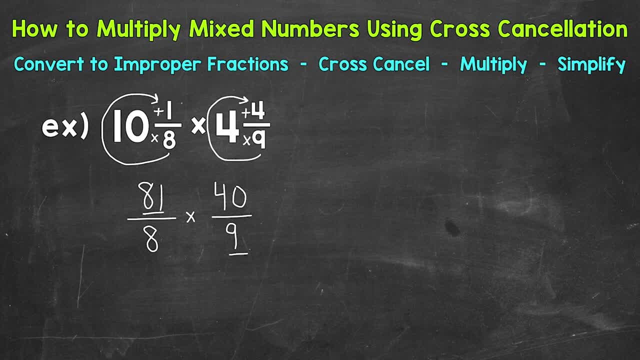 We can look for common factors there. A common factor between eighty-one and nine is nine. So what we can do, we can divide both of those by nine. So let's cross them out and divide them both by nine. Eighty-one divided by nine is nine. 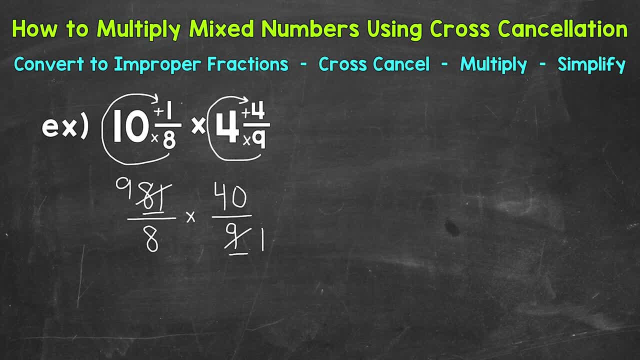 And then nine divided by nine is one. So you can see that gave us some smaller numbers in value and easier numbers to work with. We can also look the other way diagonally. So between eight and forty do we have any common factors? 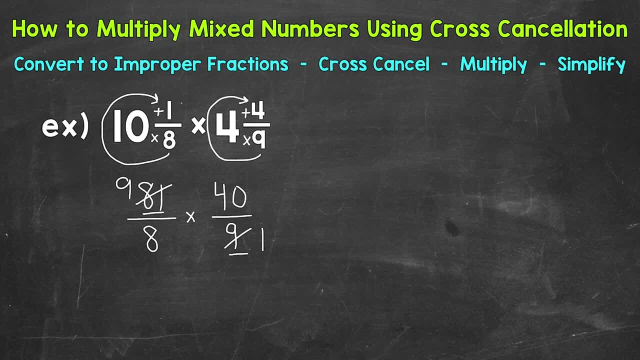 Yes, the greatest common factor between eight and forty is eight. So let's divide them both by eight. So eight divided by eight, let's cross it out. That's going to give us one. And then forty divided by eight is five. 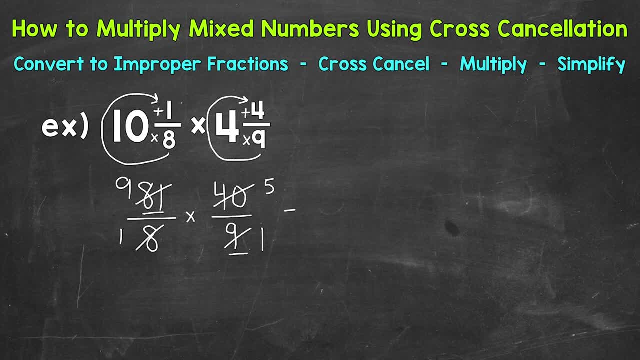 Once we get to this point, we can multiply straight across: Nine times five is forty-five, And then one times one is one. Now, forty-five over one that equals forty-five. So let's write our answer as a whole number instead of leaving it as an improper fraction. 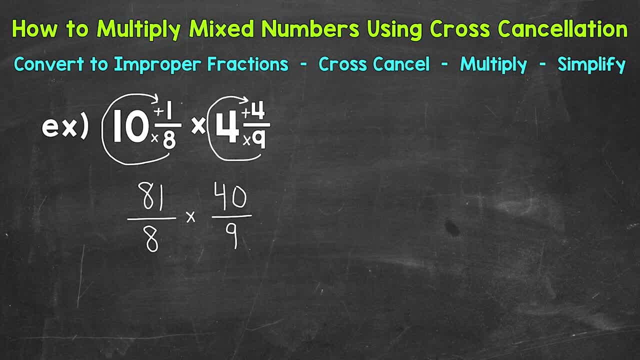 we're not changing the value of anything. And then forty-ninths is equivalent to four, and four-ninths Again. we did this. so we just have a numerator and a denominator and we are able to multiply. At this point we can multiply straight across. 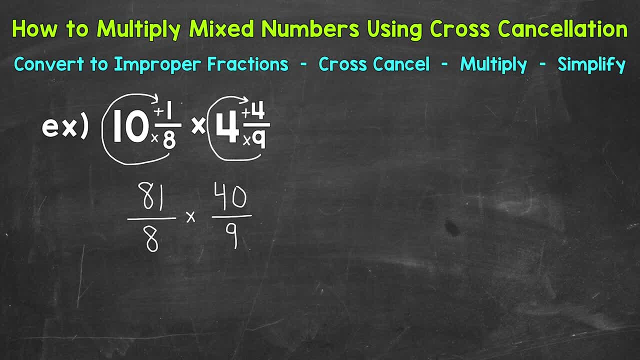 So we can do eighty-one times forty and then eight times nine, But we can use cross cancellation And this is a way to simplify fractions before multiplying. It gives us smaller and easier numbers to work with, Therefore a simpler problem to solve. 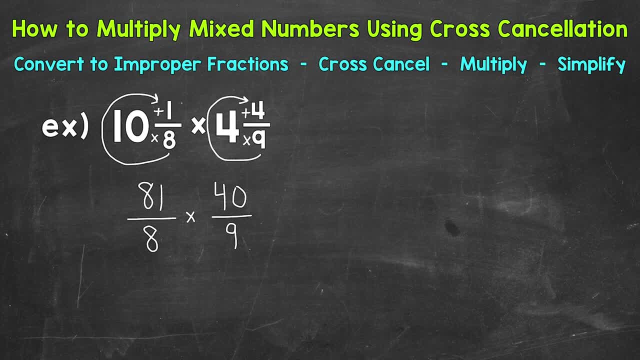 We cross cancel by looking for common factors between the numerators and denominators, So the top and bottom. Think of it as simplifying fractions. but we can look diagonally as well. For example, eighty-one and nine, So eighty-one right here and nine diagonally. 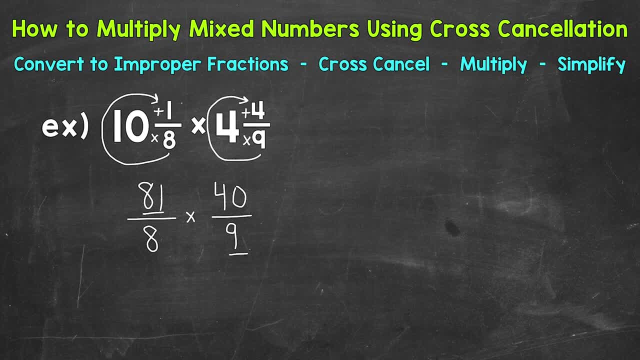 We can look for common factors there. A common factor between eighty-one and nine is nine. So what we can do, we can divide both of those by nine. So let's cross them out and divide them both by nine. Eighty-one divided by nine is nine. 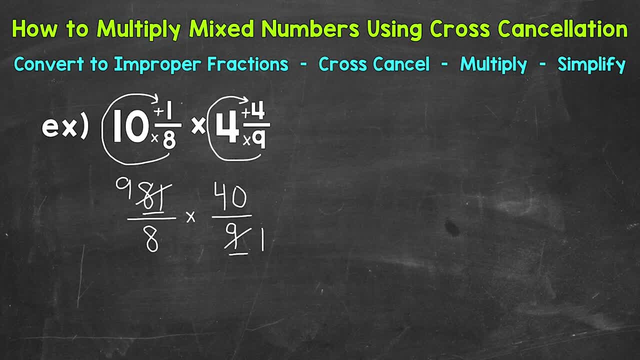 And then nine divided by nine is one. So you can see that gave us some smaller numbers in value and easier numbers to work with. We can also look the other way diagonally. So between eight and forty do we have any common factors? 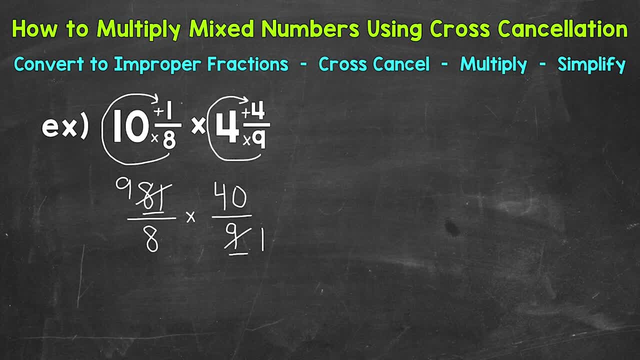 Yes, The greatest common factor between eight and forty is eight. So let's divide them both by eight. So eight divided by eight, Let's cross it out. That's going to give us one. And then forty divided by eight is five. 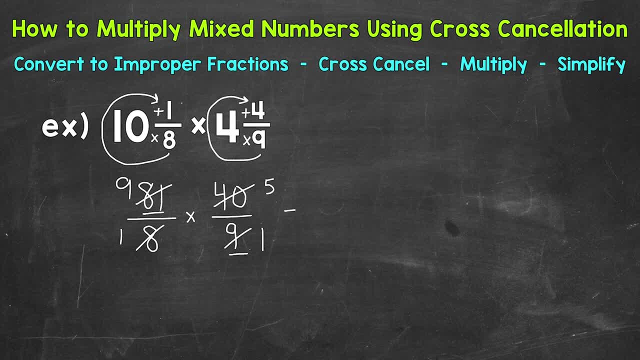 Once we get to this point, we can multiply straight. We're going to cross. nine times five is forty five, And then one times one is one. Now, forty five over one. that equals forty five. So let's write our answer as a whole number instead of leaving it as an improper fraction. 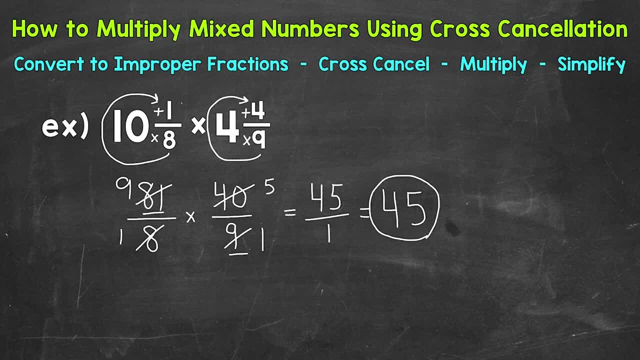 So our final answer: forty five. Now, if we did not use cross cancellation, we would have to multiply eighty one times forty, and then eight times nine, and then simplify from there, and eventually we're going to get the same answer. So cross cancellation is a useful tool when we have multiplication problems that involve fractions. 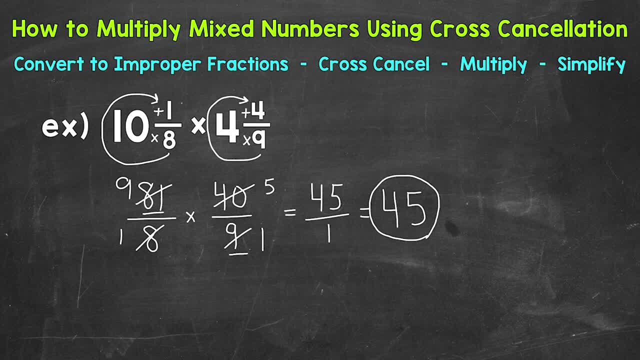 Again. it gives us smaller and easier numbers to work with. therefore, a simpler problem to solve. Think of it as simplifying the problem before multiplying. Now can we use cross cancellation for every single multiplication problem that involves fractions? No, We have to have common factors other than one between our numerators and denominators. 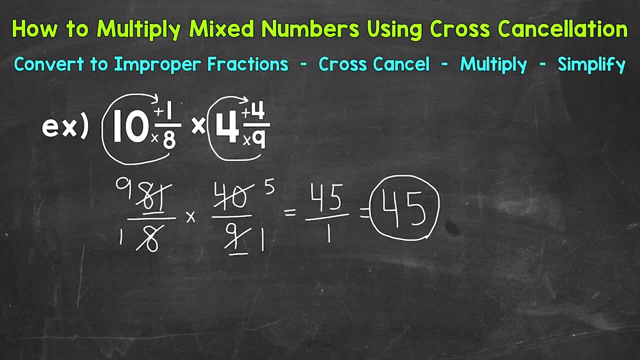 If the only common factor we have is one between our numerators and denominators, we can't use cross cancellation. So something to keep in mind. So there's how to use cancellation when multiplying mixed numbers. Let's move on to multiplying improper fractions. 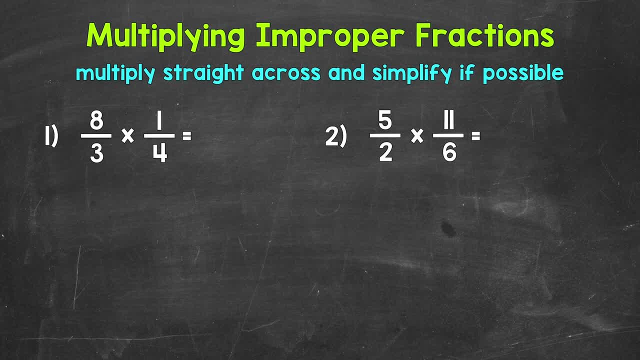 Now we will take a look at how to multiply improper fractions, So how to work through a multiplication problem involving one or more improper fractions. Now we go through any problem involving improper fractions the same way we do with proper fractions: Multiply straight across. So numerator times numerator, the top numbers, and then denominator times denominator. 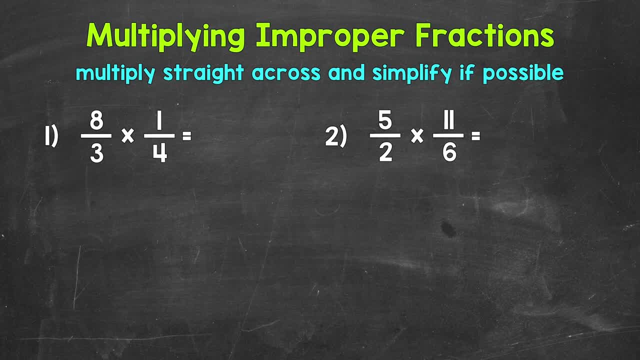 the bottom numbers and then simplify if possible. Improper fractions just have a value greater than one whole. If we're given a problem involving any improper fractions, that doesn't change the way we multiply. Let's jump into our examples, starting with number one, where we have eight thirds times one. fourth. 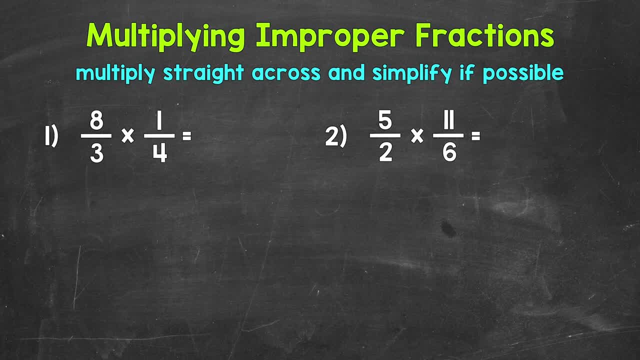 Let's multiply straight across, starting with the numerators. We have eight times one, so straight across here. eight times one is eight. Now for the denominators. So three times four is twelve. We end up with eight twelfths, which is correct. but we can simplify. 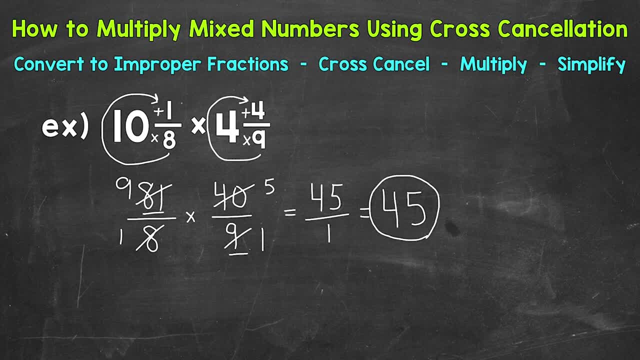 So our final answer: forty-five. Now, if we did not use cross cancellation, we would have to multiply eighty-one times forty, and then eight times nine, and then simplify from there, And eventually we're going to get the same answer. So cross cancellation is a useful tool. 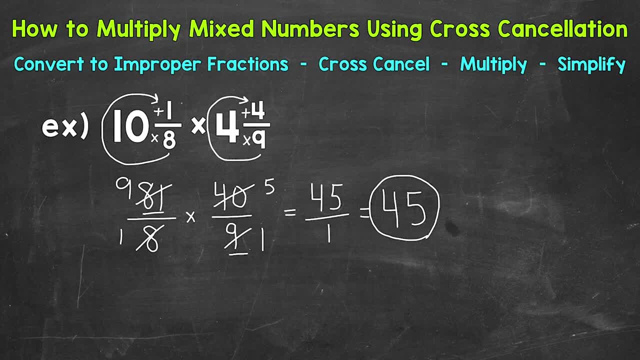 when we have multiplication problems that involve fractions. Again, it gives us smaller and easier numbers to work with, therefore a simpler problem to solve. Think of it as simplifying the problem before multiplying. Now can we use cross cancellation for every single multiplication problem that involves fractions? 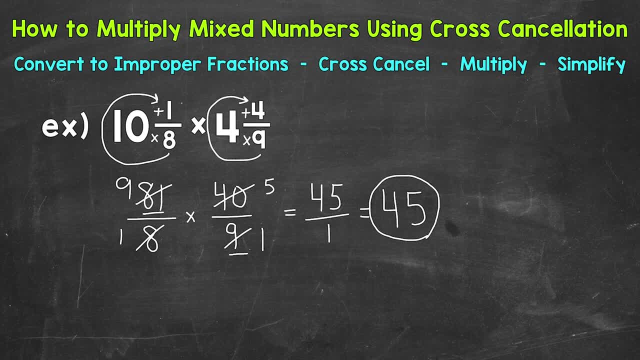 No, we have to have common factors other than one between our numerators and denominators. If the only common factor we have is one between our numerators and denominators, we can't use cross cancellation. So something to keep in mind. So there's how to use cancellation when multiplying mixed numbers. 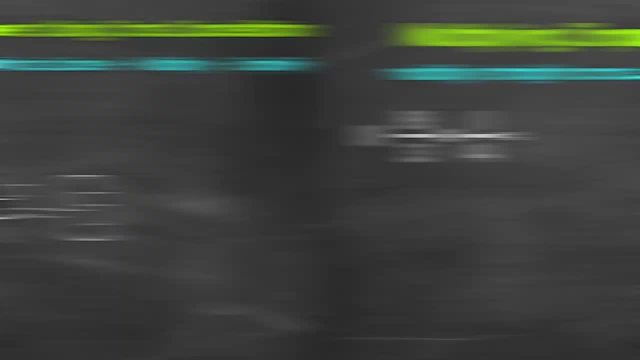 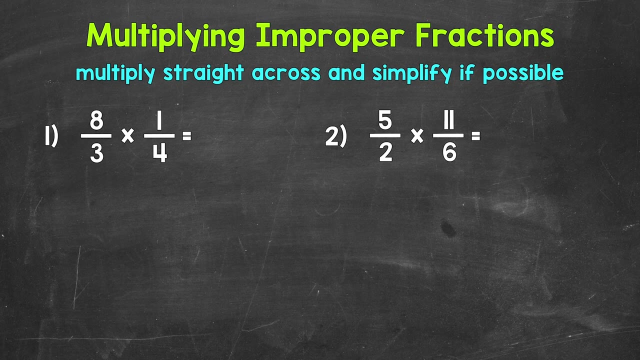 Let's move on to multiplying improper fractions. Now we will take a look at how to multiply improper fractions, So how to work through a multiplication problem involving one or more improper fractions. Now we go through any problem involving improper fractions the same way we do with proper fractions. 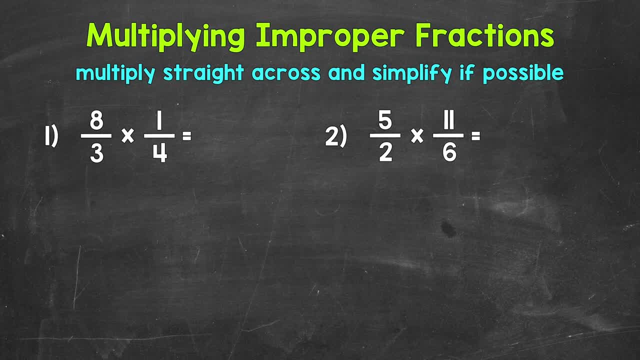 Multiply straight across, so numerator times numerator the top numbers, and then denominator times denominator the bottom numbers, and then simplify if possible. Improper fractions just have a value greater than one whole If we're given a problem involving any improper fraction. 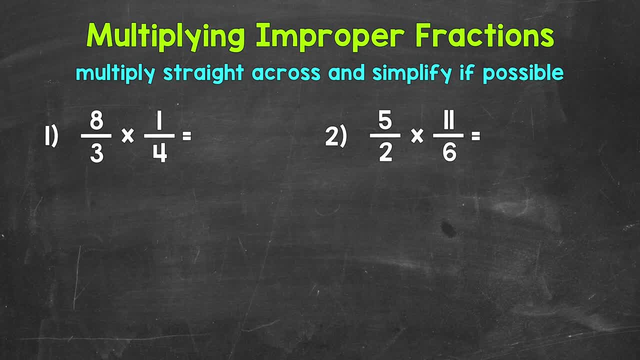 that doesn't change the way we multiply. Let's jump into our examples, starting with number one, where we have eight thirds times one. fourth, Let's multiply straight across, starting with the numerators: We have eight times one, so straight across here. 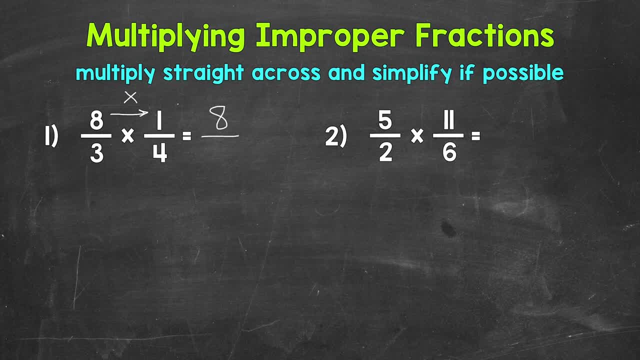 Eight times one is eight, Now for the denominators. So three times four is twelve. We end up with eight, twelfths, which is correct. but we can simplify. The greatest common factor between eight and twelve is four. Let's divide eight and twelve by four. 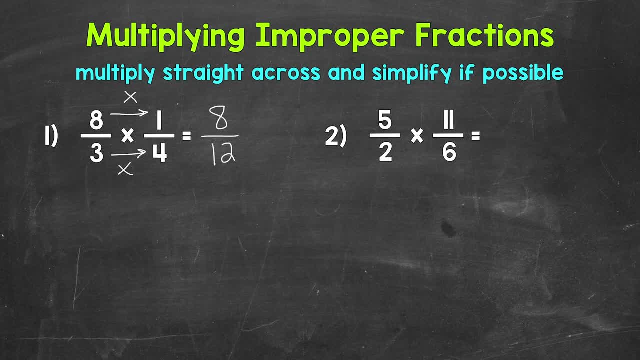 The greatest common factor between eight and twelve is four. Let's divide eight and twelve by four. So eight divided by four and twelve divided by four. Eight divided by four is two. Twelve divided by four is three. Two thirds is in simplest form. so this is our final simplified answer: two thirds. 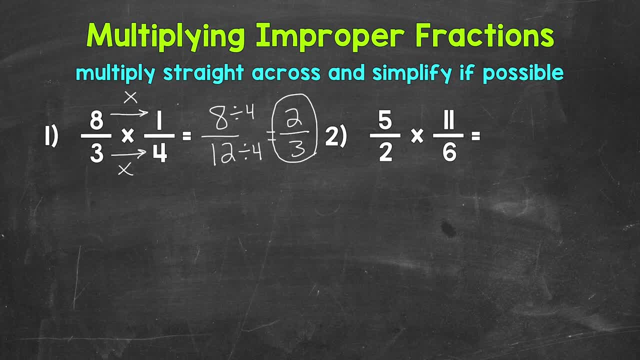 Let's move on to number two, where we have five halves times eleven sixths. Let's multiply straight across, starting with the numerators: Five times eleven is fifty-five. Now for the denominators: Two times six is twenty-five. Fifty-five is twelve. 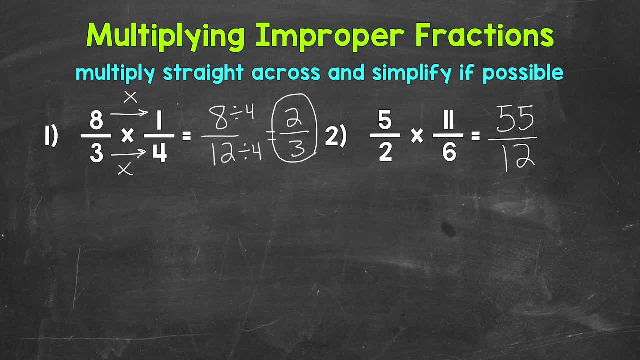 So we end up with fifty-five twelfths, which is an improper fraction. So let's convert this to a mixed number for our final answer. We do that by dividing. So we divide the numerator fifty-five by the denominator twelve. So fifty-five divided by twelve. 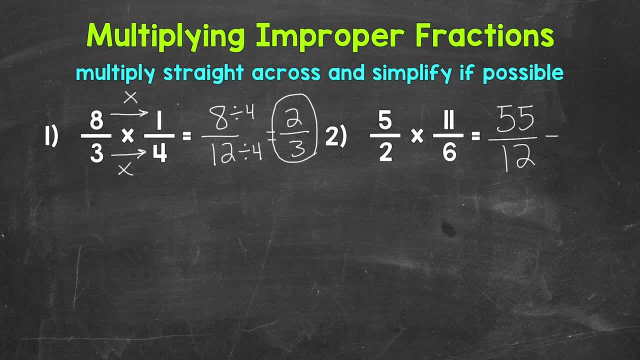 How many whole groups of twelve in fifty-five? Well, four, That gets us to forty-eight. We don't hit fifty-five exactly. We have a remainder of seven, And then we keep the denominator of twelve the same. We end up with four and seven twelfths. 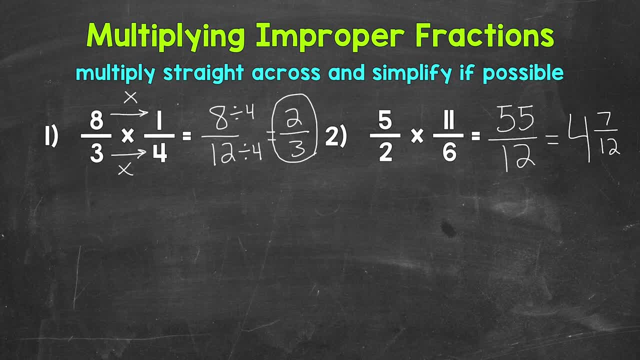 We can look to see if we can simplify that fractional part of the mixed number. Seven twelfths is in simplest form: the only common factor between seven and twelve is one. So our final answer: Four and seven twelfths. Now I do want to review real quick how we went from that improper fraction to a mixed number by writing out all of the steps. 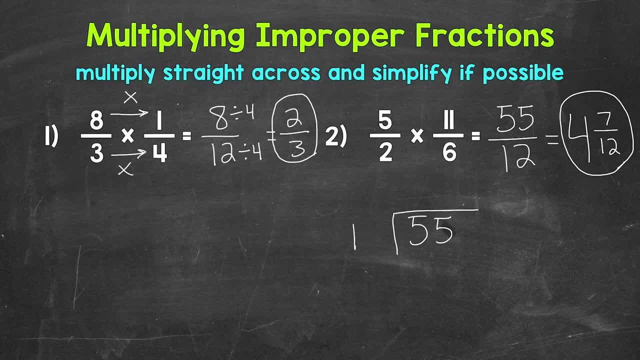 So we divided the numerator fifty-five by twelve. So fifty-five divided by twelve, How many whole groups of twelve in fifty-five Four? So that's the whole number part of our mixed number. Four times twelve is forty-eight. Fifty-five minus forty-eight gives us a remainder of seven. 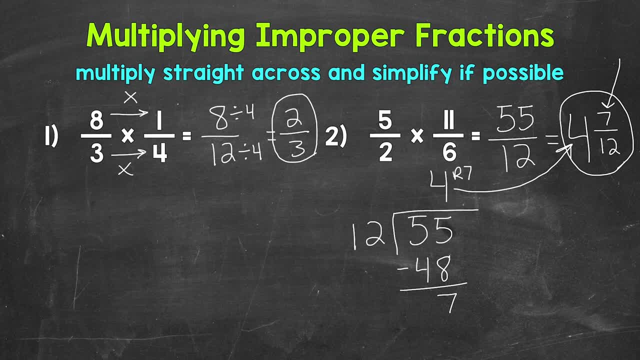 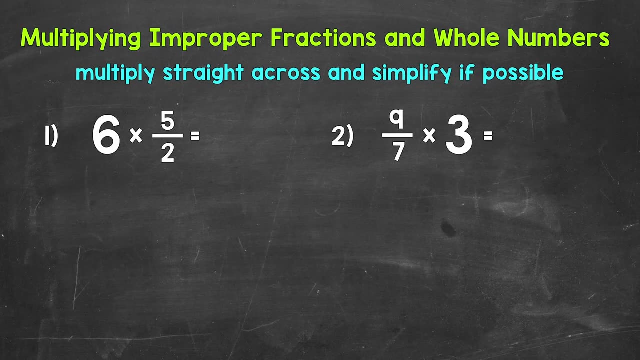 That goes right here. Then we keep the denominator of twelve the same, So we end up with four and seven twelfths. There's how to multiply improper fractions. Let's move on to multiplying improper fractions and whole numbers. Now we will take a look at how to multiply. 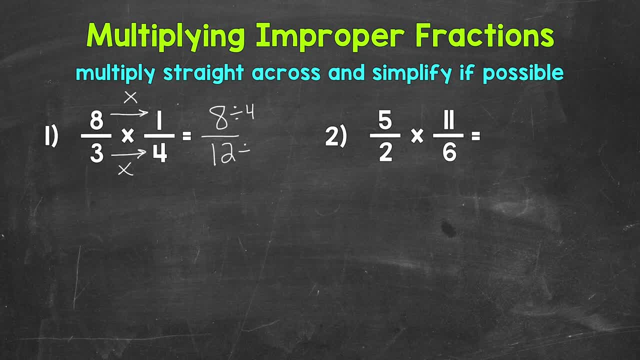 So eight divided by four and twelve divided by four, Eight divided by four is two. Twelve divided by four is three. Two thirds is in simplest form. so this is our final Simplified answer: two thirds. Let's move on to number two, where we have five halves times eleven, sixths. 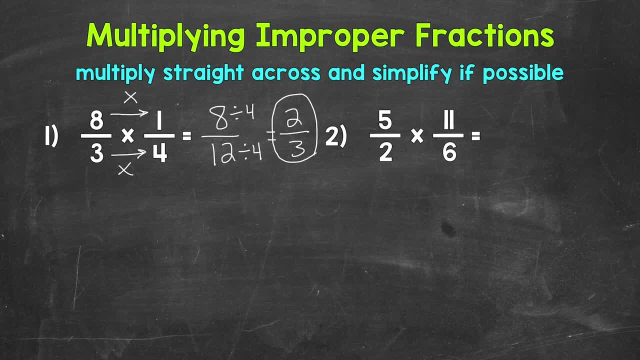 Let's multiply straight across, starting with the numerators: Five times eleven is fifty-five. Now for the denominators: Two times six is twelve, So we end up with fifty-five twelfths, which is an improper fraction. So let's convert this to a mixed number for our final answer. 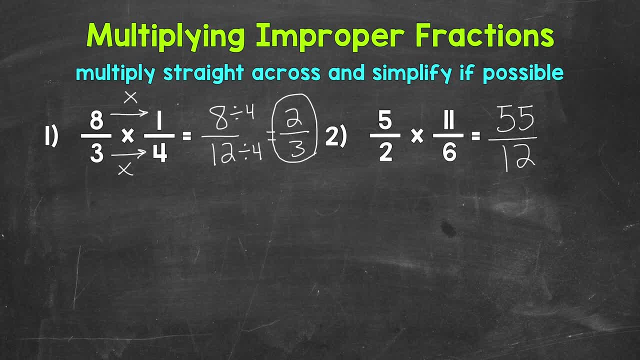 We do that by dividing. So we divide the numerator fifty-five by the denominator twelve. So fifty-five divided by twelve, How many whole groups of twelve in fifty-five? Well, four, That gets us to forty-eight. We don't hit fifty-five exactly. 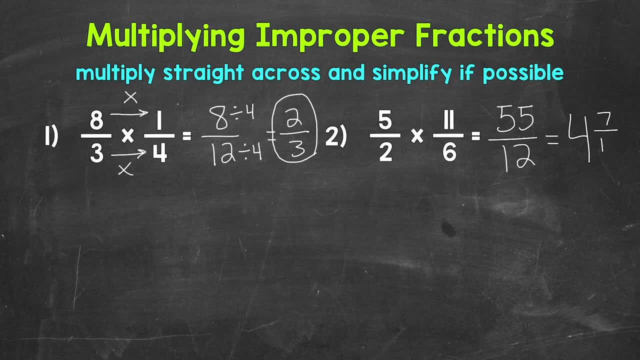 We have a remainder of seven And then we keep the denominator of twelve the same. We end up with four and seven twelfths. We can look to see if we can simplify that fractional part of the mixed number. Seven twelfths is in simplest form, the only common factor between seven and twelve is one. 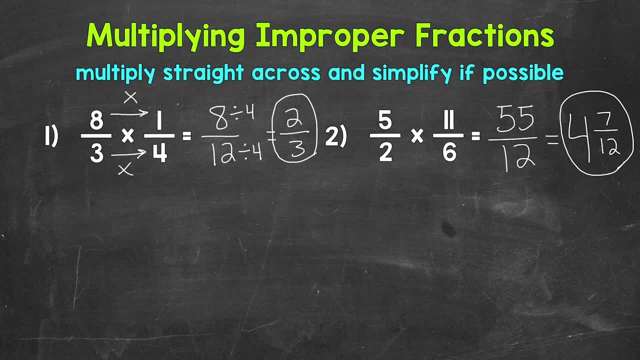 So our final answer: four and seven, twelfths. Now I do want to review real quick how we went from that improper fraction to a mixed number by writing out all of the steps. So we divided the numerator fifty-five by twelve. 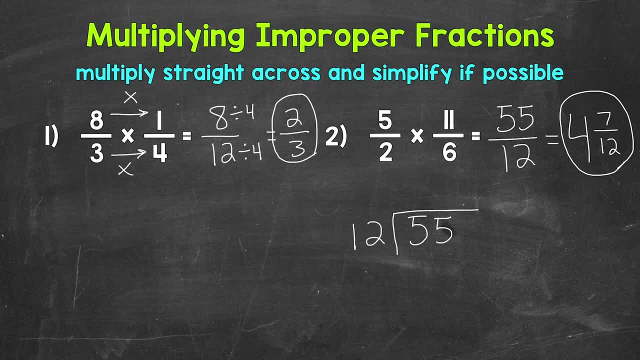 So fifty-five divided by twelve, How many whole groups of twelve in fifty-five? Four? So that's the whole number part of our mixed number. Four times twelve is forty-eight. Fifty-five minus forty-eight gives us a remainder of seven. That goes right here. 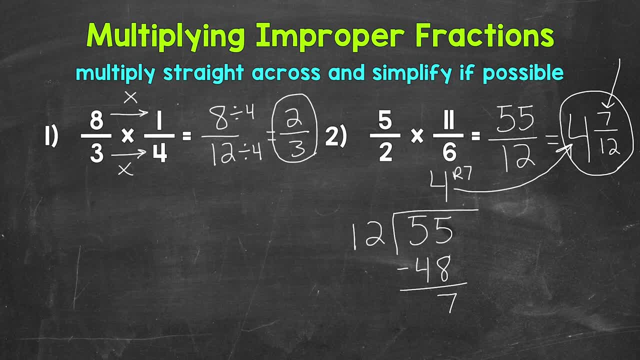 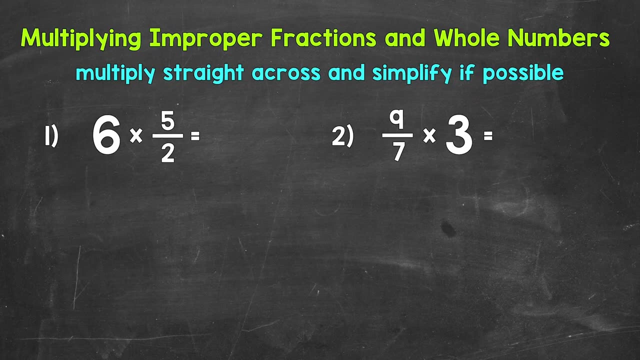 Then we keep the denominator of twelve the same, So we end up with four and seven twelfths. There's how to multiply improper fractions. Let's move on to multiplying improper fractions and whole numbers. Now we will take a look at how to multiply improper fractions and whole numbers. 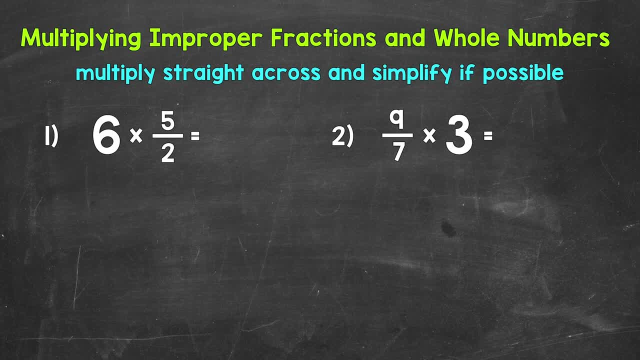 improper fractions and whole numbers. Let's jump into our examples, starting with number one, where we have six times five halves. Now we need to multiply straight across and simplify if possible. Since we need to multiply straight across, we need to rewrite the whole number in fractional form. 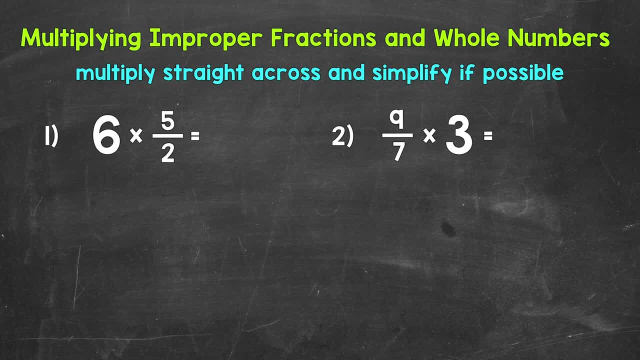 That way we have a numerator and denominator and we can multiply straight across. So let's rewrite that whole number Six in fractional form, And we do that by putting it over one. We can rewrite any whole number in fractional form by putting it over one. 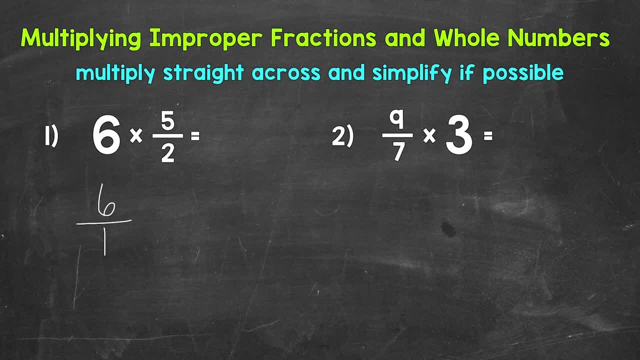 We're not changing the value of that six, That fraction six over one still has a value of six times five halves. Now we can multiply straight across. Since we rewrote that whole number in fractional form, we have a numerator and a denominator. 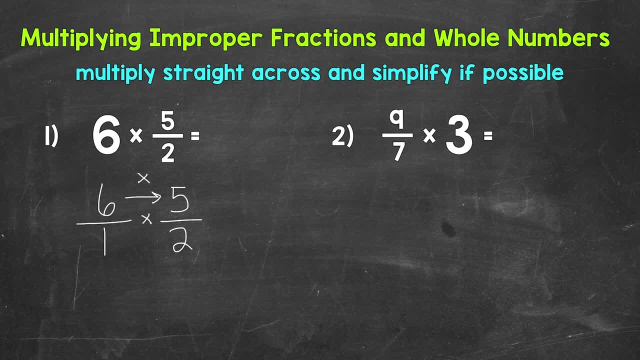 Let's start with the numerators. So six times five is thirty. Now for the denominators: one times two is two, So we end up with thirty halves thirty over two. But this is an improper fraction, So let's convert this to a mixed number. 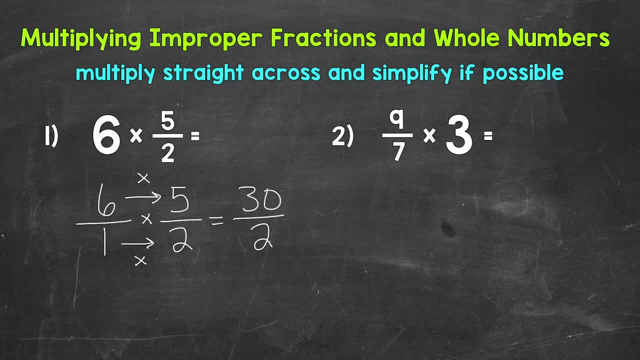 We do that by dividing the numerator by the denominator. So we have thirty divided by two. How many whole groups of two in thirty? Well, fifteen, And we hit thirty exactly. We do not have a remainder, So this actually works out to be a whole number, not a mixed number. 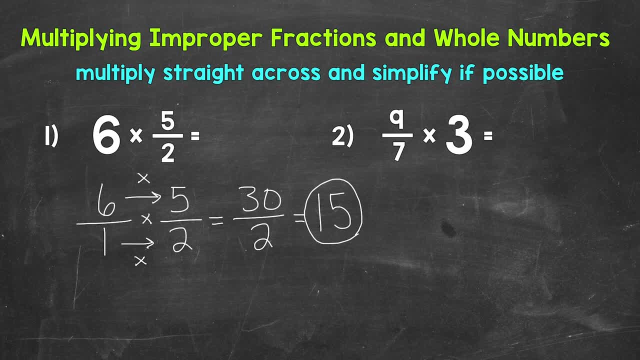 Again, because we don't have a remainder there. So six times five halves equals fifteen. Let's move on to number two, where we have nine sevenths times three. So let's rewrite this. Let's start with the whole number in fractional form. 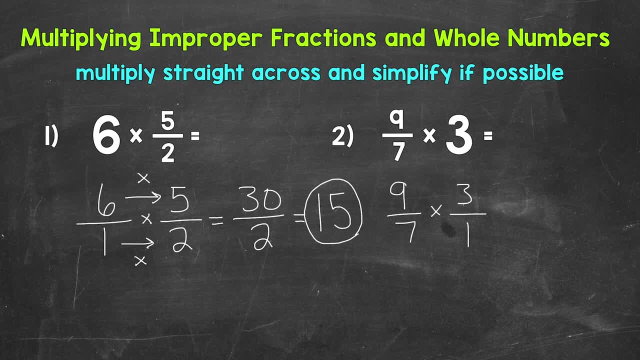 That way we have a numerator and a denominator and we can multiply straight across. Let's start with the numerators: Nine times three is twenty seven. Now for the denominators: seven times one is seven. So we end up with twenty seven sevenths, which is an improper fraction. 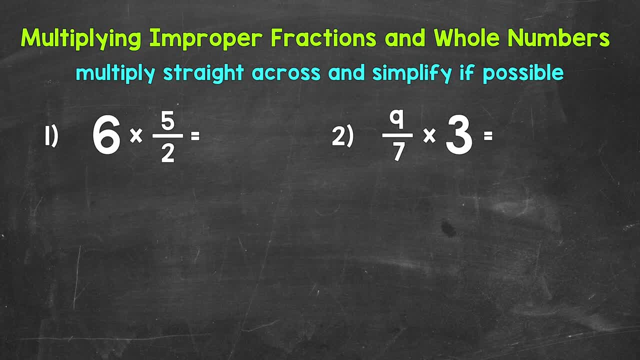 Let's jump into our examples, starting with number one, where we have six times five halves. Now we need to multiply straight across and simplify if possible. Since we need to multiply straight across, we need to rewrite the whole number in fractional form. 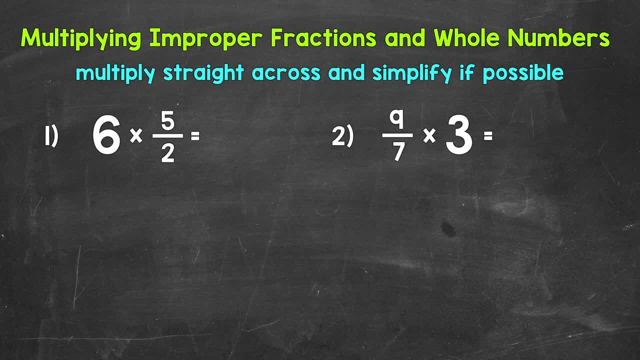 That way we have a numerator and denominator and we can multiply straight across. So let's rewrite that whole number six in fractional form, And we do that by putting it over one. We can rewrite any whole number in fractional form by putting it over one. 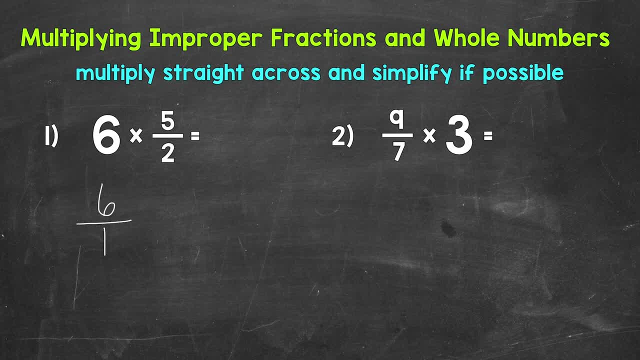 We're not changing the value of that six, That fraction six over one still has a value of six Times five halves. Now we can multiply straight across. Since we rewrote that whole number in fractional form, we have a numerator and a denominator. 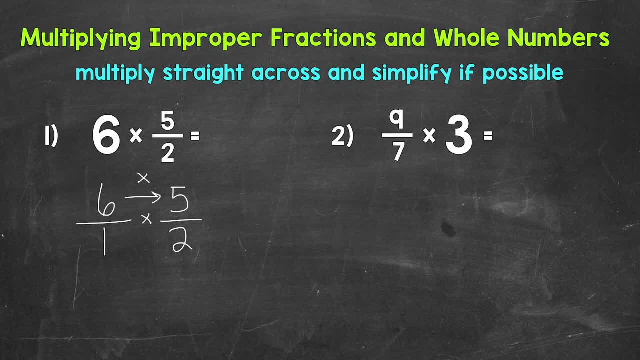 Let's start with the numerators. So six times five is thirty. Now for the denominators: One times two is two, So we end up with thirty halves Thirty over two. But this is an improper fraction, So let's convert this to a mixed number. 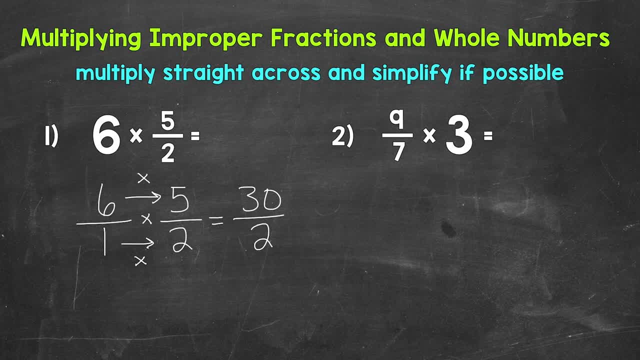 We do that by dividing the numerator by the denominator. So we have thirty divided by two. How many whole groups of two in thirty? Well, fifteen, And we hit thirty exactly. We do not have a remainder, So this actually works out to be a whole number, not a mixed number. 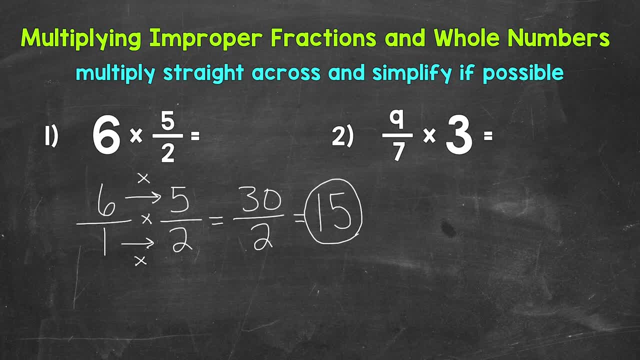 Again, because we don't have a remainder there. So six times five halves equals fifteen. Let's move on to number two, where we have nine sevenths times three. So let's rewrite this with the whole number in fractional form. That way we have a numerator and a denominator and we can multiply straight across. 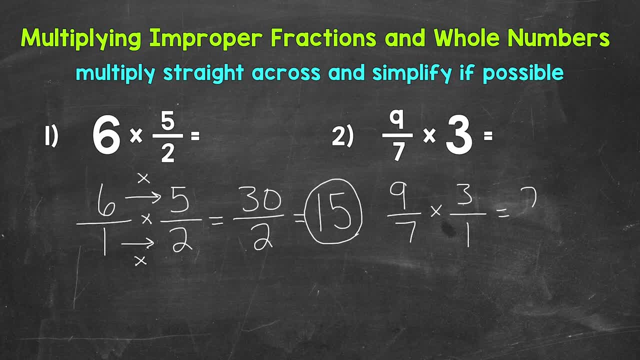 Let's start with the numerators. Nine times three is twenty seven. Now for the denominators: Seven times one is seven. So we end up with twenty seven sevenths, which is an improper fraction. So let's convert this to a mixed number. 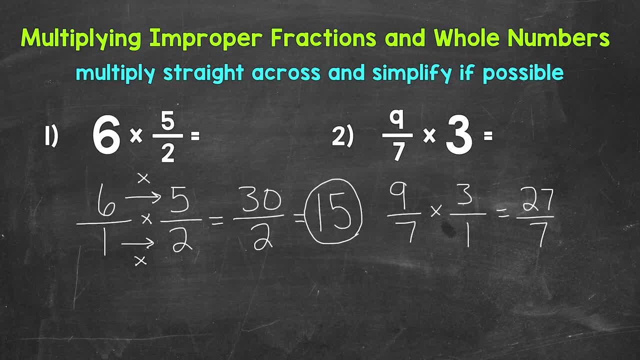 We divide the numerator by the denominator in order to do that. So twenty seven divided by seven, How many whole groups of seven in twenty seven? Well, three whole groups. That gets us to twenty one. So we have a remainder of six.